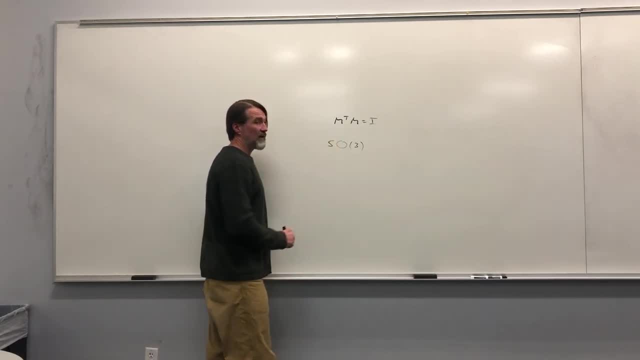 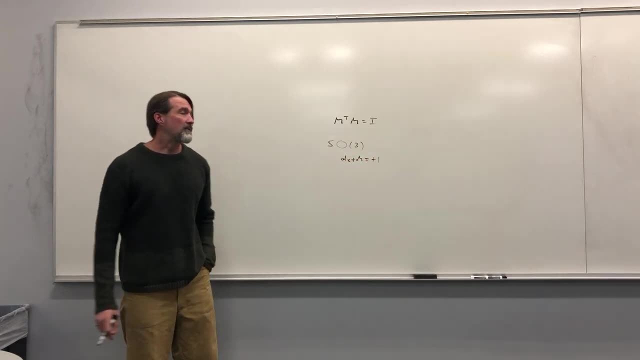 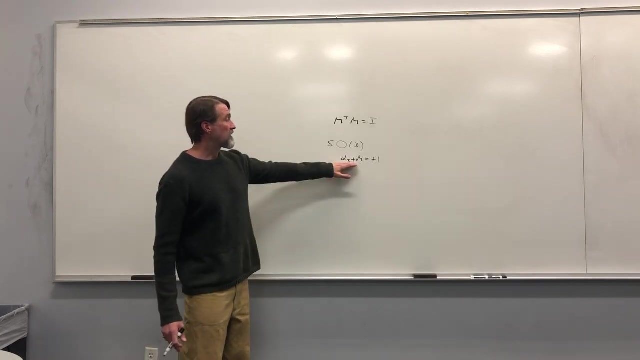 And then I said: well, you can also go to SO3, which is basically taking the determinant of all of these and setting it equal to plus one. And it turns out that for any matrix which satisfies this, the determinant is always going to be plus or minus one. but we're going to pick the set which has determinant plus one. 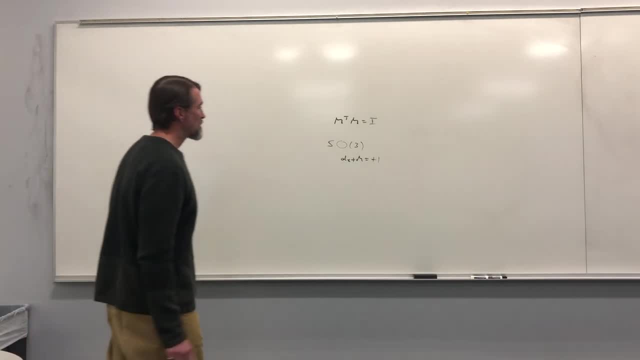 What I did not point out to you, which I thought might be obvious, but maybe it's not- is: if you want, If you want to use a Lie group, then you have to use SO3. You can't use O3.. 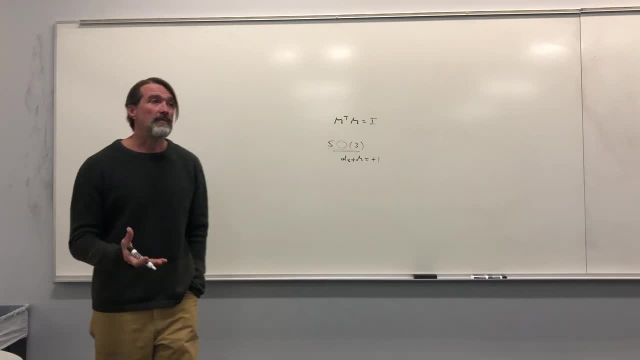 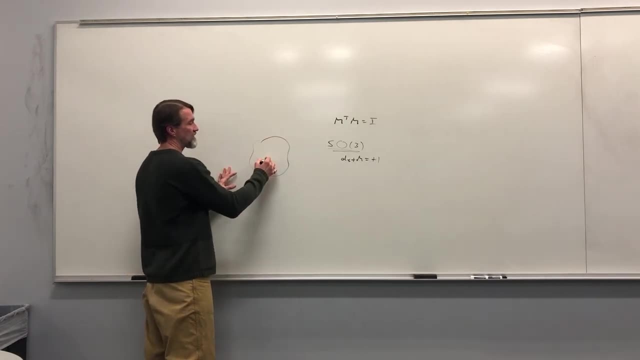 And the reason for that is hopefully somewhat intuitive. Remember I said that one of the important things about Lie groups is that you can take the whole space of all transformations and you can pretty much describe what's going on just very close to the identity. So if you know the infinitesimal forms of the transformations you can build up, 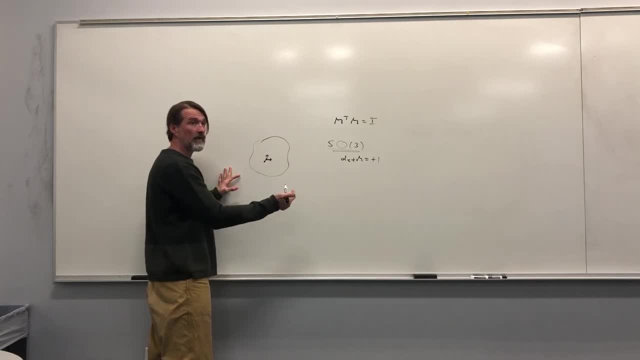 You can build up arbitrary ones just by putting those together. Okay. Here's the important thing, though: If you're really close to the identity, you have to have the same determinant that the identity does, and the identity has determinant plus one. 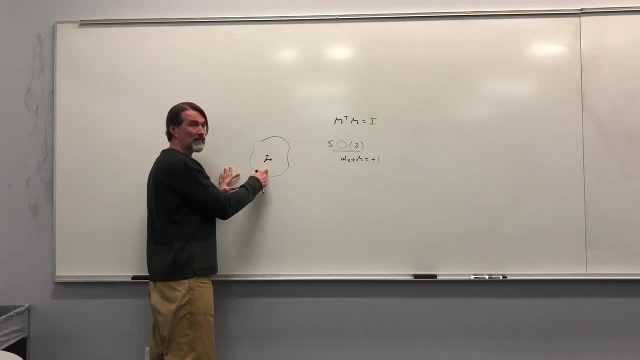 So for the transformations in O3 that are connected to the identity continuously, they're the SO3 transformations. Similarly, for the unitary groups, they're SUN Again that you have to use. You have to use for a Lie group, But anyway, that's just in detail. 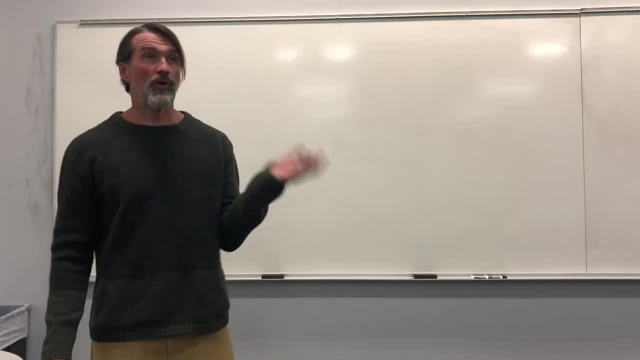 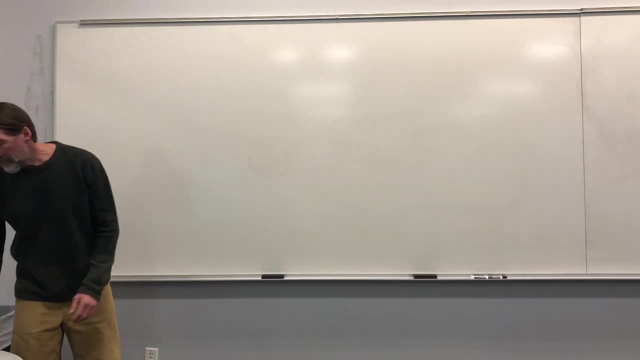 The groups we use in this class are obviously SO1,, SO4,, SU3,, SU2, and U1. So they're all of that type. Okay, All right. So I'm going to- Basically, we're going to take a step here which is going to be pretty amazing. 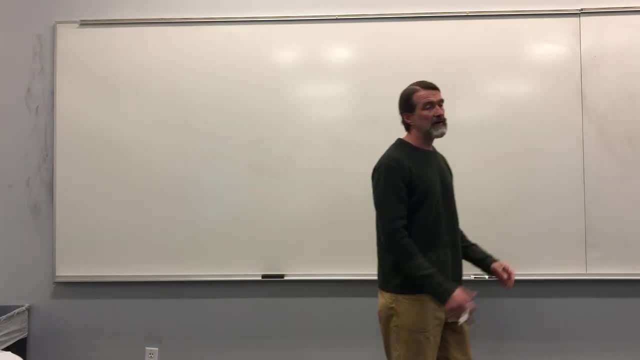 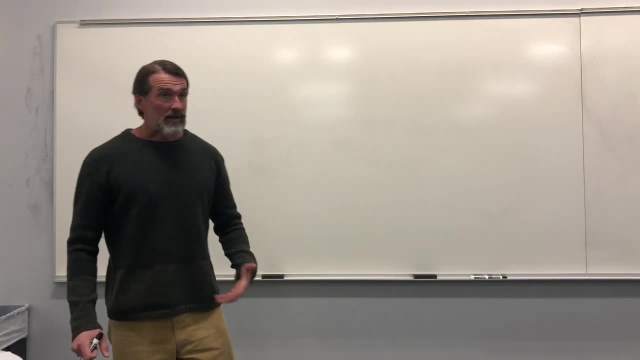 I'll get through an amazing aspect of it today, and then we'll finish the story next Tuesday. Today I'm going to be really heavy on computation. Nonetheless, at the end you'll be like: Oh, But on next Tuesday, which is, of course, the last lecture before our exam next Thursday. 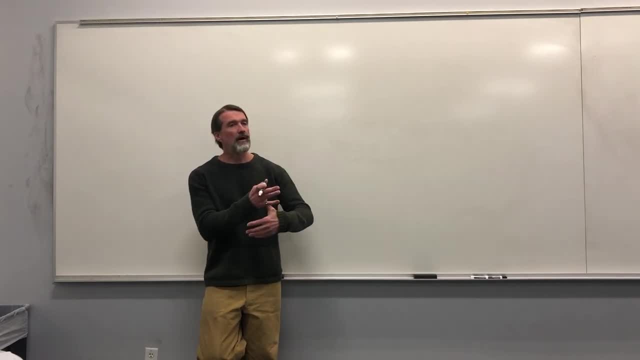 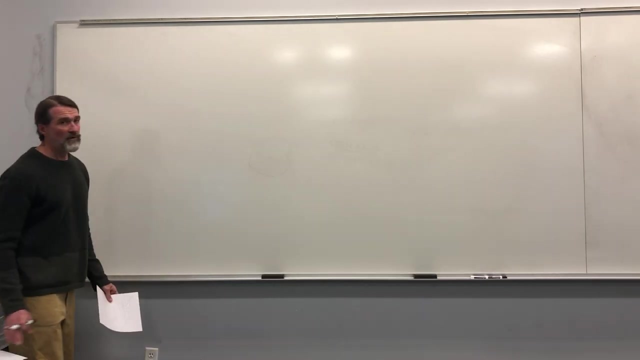 in our lecture next Tuesday we'll give a more picturesque version of what's going on and hopefully that will make more sense And I'll actually contact it to ideas that you've already seen in other contexts. But here we go. I'm going to start with just a review of where we are. 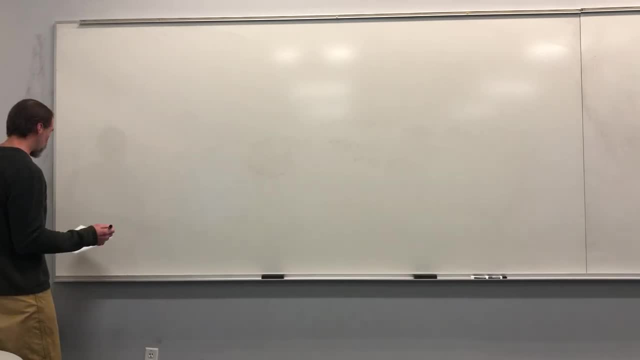 And then this will actually be Sort of a summary of what problems we have to figure out. So I'm going to write down a lot of stuff which we've already seen and used. So we started out with a set of free Lagrangians. 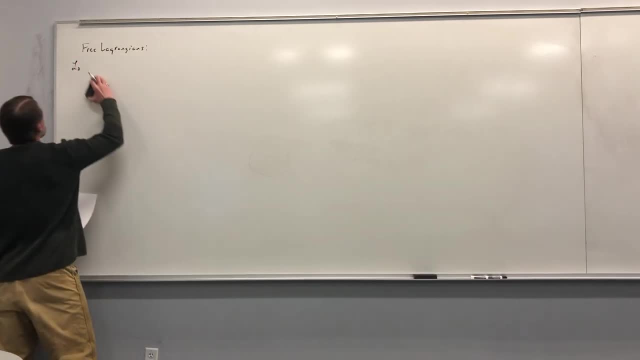 We have the spin zero particle Lagrangian, And these are free Lagrangians. So, yeah, just sit up there. So we have the Klein-Gordon expression, which is B mu phi, B mu phi, plus plus one-half mc over h-bar, squared, phi-squared. 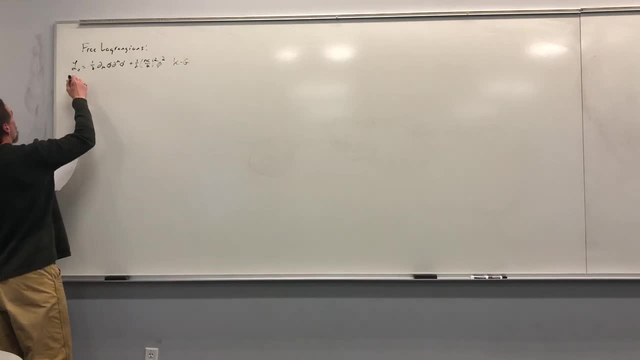 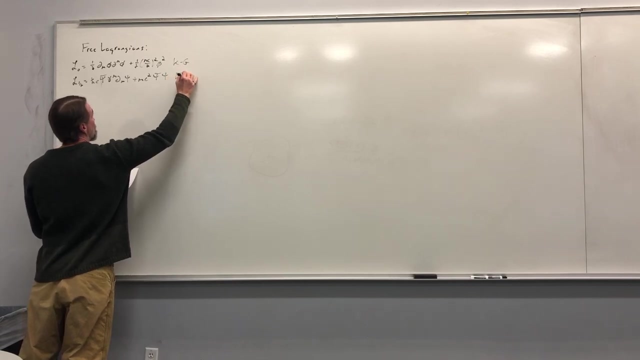 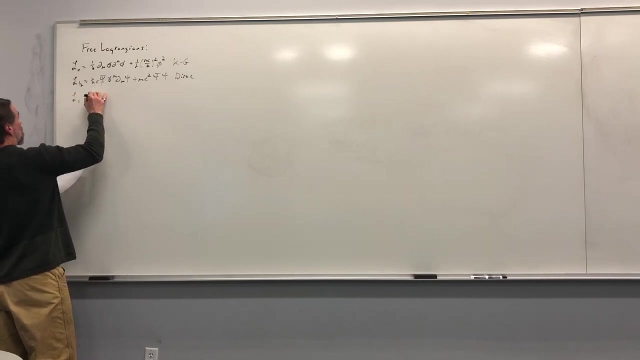 Okay, that's Klein-Gordon. And then we have the Dirac-Lagrangian, which is h-bar c, psi-bar gamma, mu, d, mu, psi plus mc squared psi-bar psi. That's Dirac. And we also have the Prokoh-Lagrangian, which is for particles of spin one. 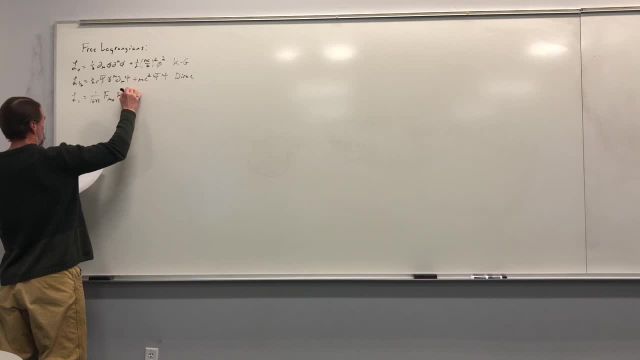 which is one over 16 pi f mu nu, f mu nu, plus one over h-pi mc over h-bar squared. a mu Oops, a mu a nu Or a mu a nu, Mu mu mu, it doesn't matter. 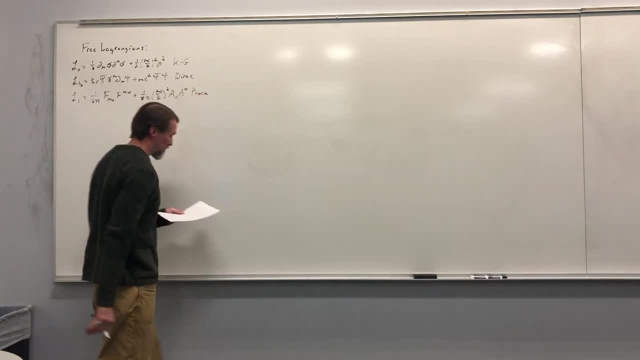 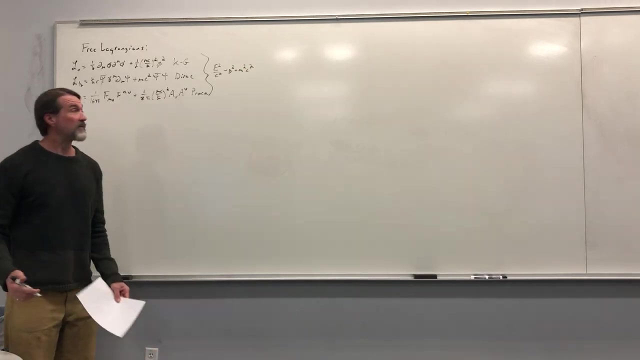 I'll use mu. So this is Prokoh, Okay. All of these, of course, imply the mass shell condition that e squared over c squared, minus p squared, equals mc squared, c squared, Okay, and that's just equal to minus p. mu, p, mu. 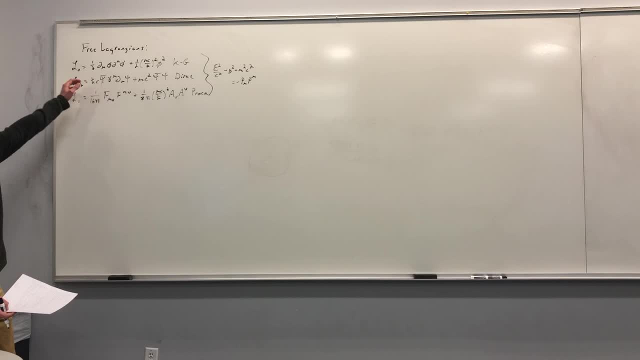 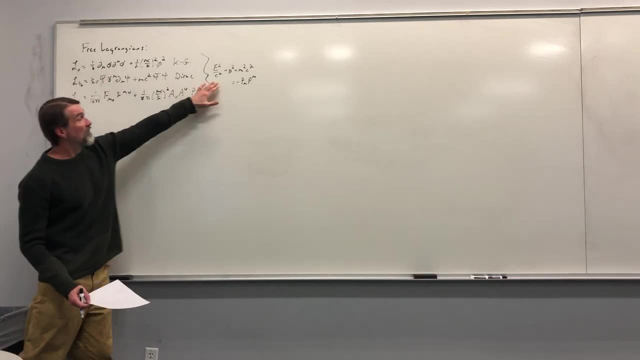 Okay, Remember, we proved or we showed that the Klein-Gordon expression, the Klein-Gordon, is actually contained in the Dirac and the Prokoh. So they and the Klein-Gordon is built from this expression. So the Dirac and the Prokoh, they just have additional descriptions on them. 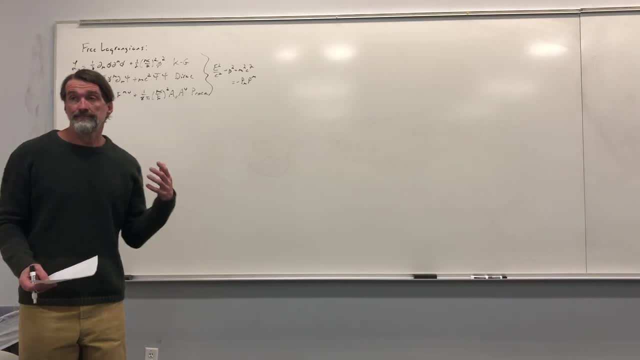 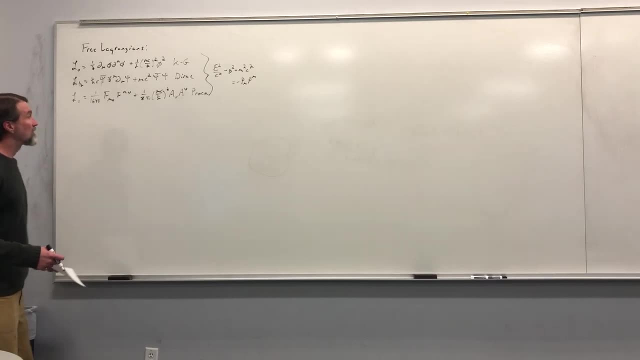 of the spin degrees of freedom that the Klein-Gordon does not have, because it's spin zero. Okay, So what we of course do- or now we know what we do- we start with a spin 1⁄2.. 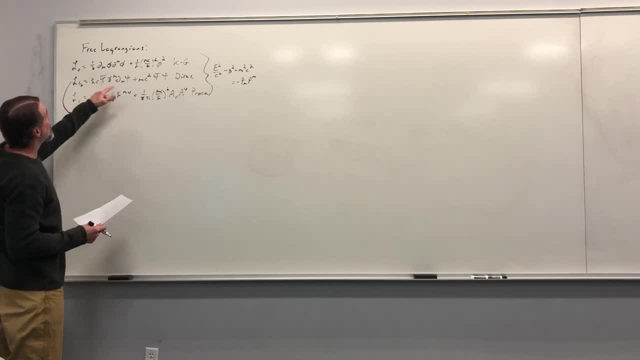 Okay, And we want to write it in a form which is invariant under some global symmetry, which is in which is basically a Lie group, So we'll just say a Lie group G with generators lambda, i. Okay, And then what we want is for the Lagrangian that we start with to be invariant. 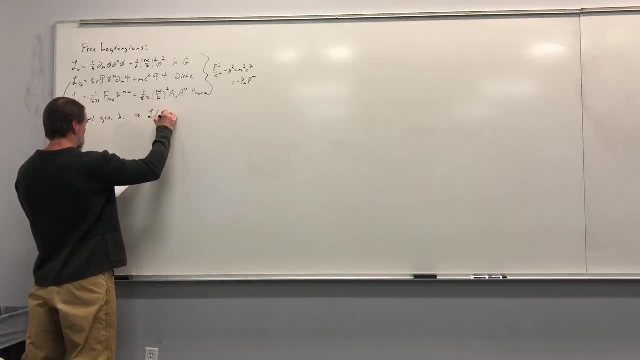 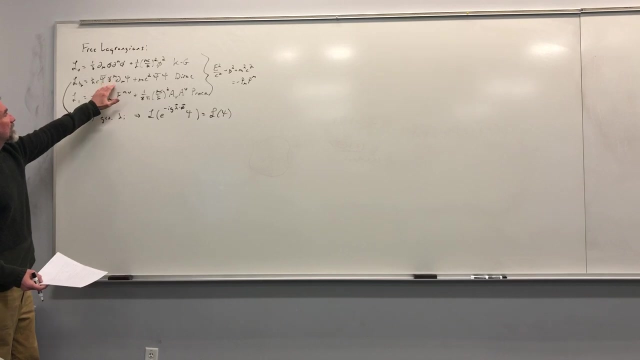 under the global form of this transformation. That is, if I take L And I do the transformation, Then I want to get back the same Lagrangian. Okay, So this is a global transformation. So the reason I'm saying this is because when we did electromagnetism, 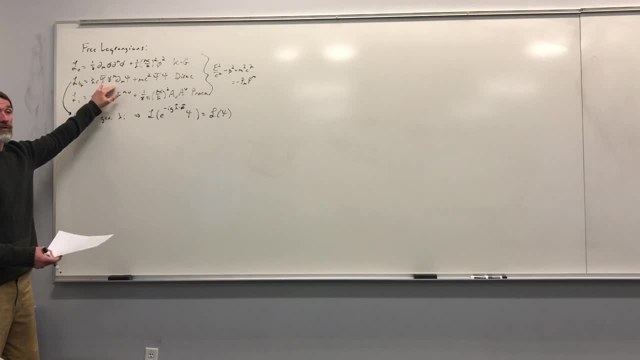 it turns out this Lagrangian, as it was written, was already invariant under that global phase transformation. Okay, Okay, Okay, Okay, Okay, Okay, Okay. used e to the ig phi because there was no matrix form in that. 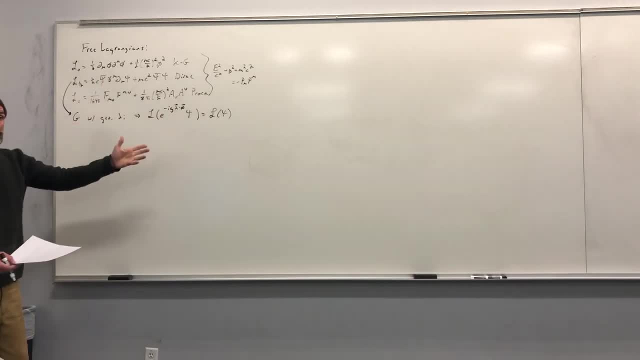 It's just u1.. However, to do su3, where we're working with three by three matrices, we had to promote the size to three component objects. Okay, And then these transformations had eight generators, And so we had an eight parameter. 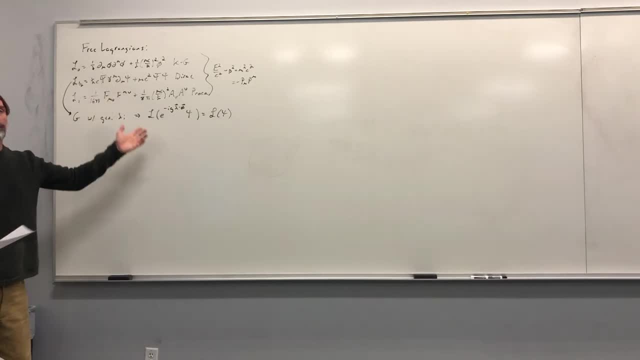 or an eight component parameter vector, And then, when we did su2, left cross, u1, hypercharge, that again brought in these sort of crazy things. Okay, But nonetheless, this is the generic form of a transformation from a Lie group, And this is global. 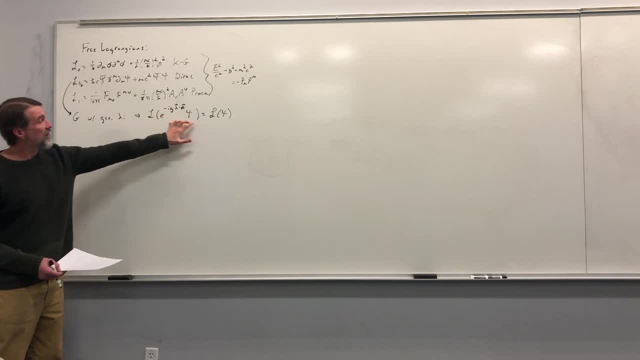 And we just have to massage this a tiny bit so that it's invariant under the global transformation. And then what we want to do, and just just I just want to remind you of things: This is the coupling, These are the generators. 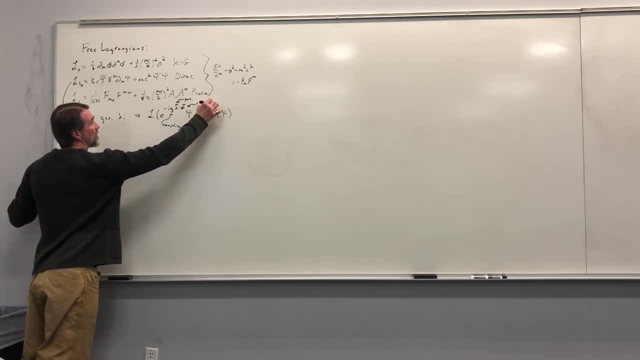 And these are the generators And these are the parameters. So the generators, actually, they're just they're, they're the fundamental building blocks of the group transformations. So so the generators are just sort of a fixed set, And then the parameters are saying how much. 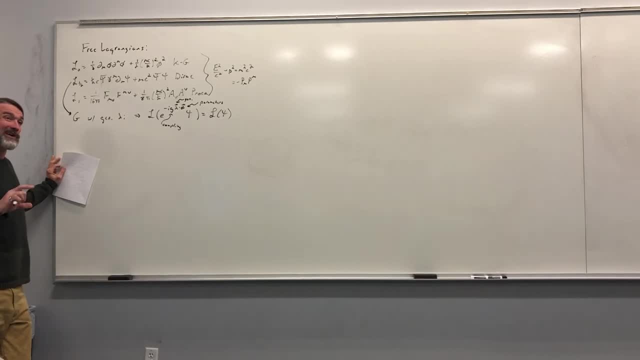 you want to transform for each generator. So if you want to transform zero for a particular generator, you just have this component of this be zero. If you want to transform by two, you make the parameter two. The generators are always the same. 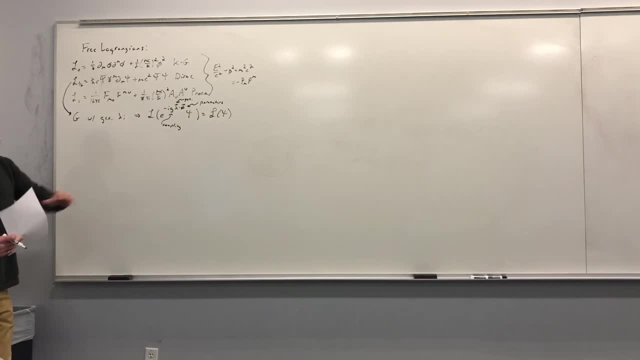 And then the coupling is just a number which tells you how strong this thing is impacting what you're transforming. Okay, So then we of course promoted a constant set of transformations to a local set of transformations. Okay, And in order to do this, 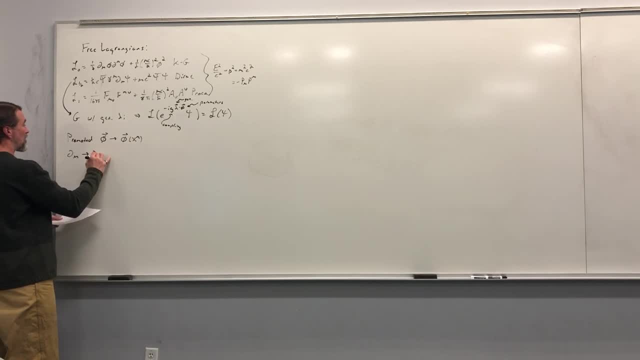 we basically had to redefine the derivative to what we've done. Okay, And in order to do this, we basically had to redefine the derivative to what we've done. We call it covariant form And, in general, this covariant form took the following form: 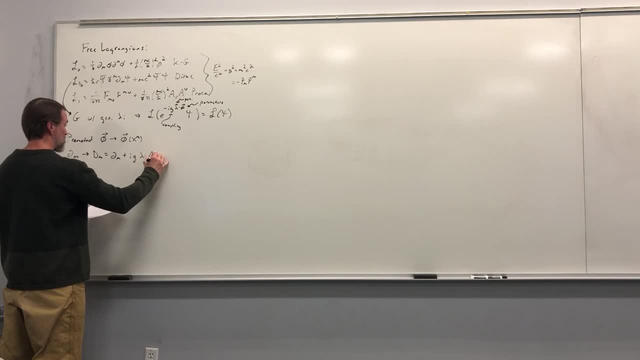 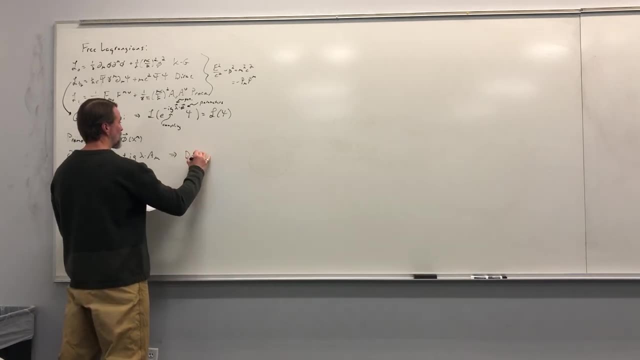 I G Lambda dot a mu. Okay, And what we found is that this derivative was actually covariant, in the sense that if I take d mu, psi and I transform both the derivative and psi, this just comes out to be e to the minus i. 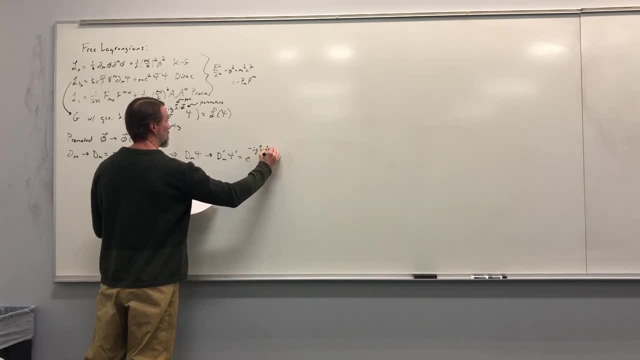 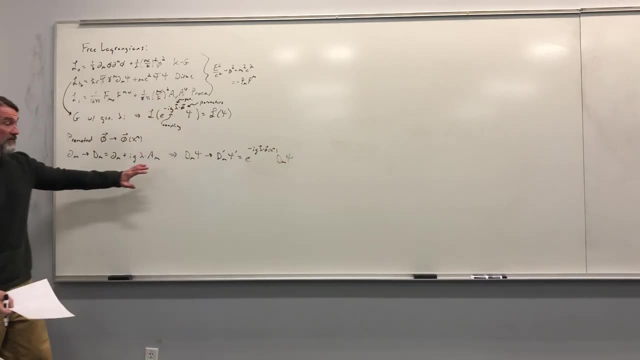 this just comes out to be e to the minus i. this just comes out to be e to the minus i. g Lambda dot phi times d mu psi. Okay, So this is not natural. We had to do some stuff to get this. 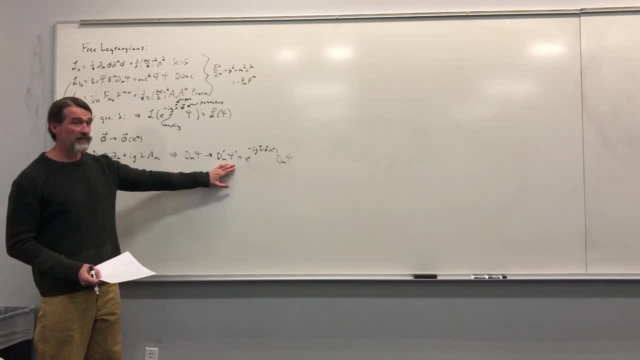 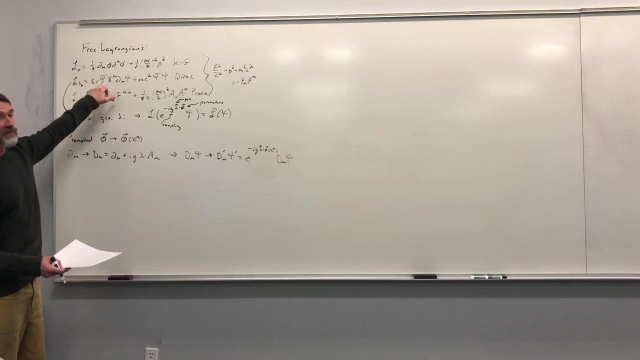 but this is the really nice transformation property of the derivative of psi, because basically the transformation which you would just enact on psi, but because of this newly defined derivative it actually just comes outside of the whole thing And that then cancels with the transformation of psi bar to make it invariant. 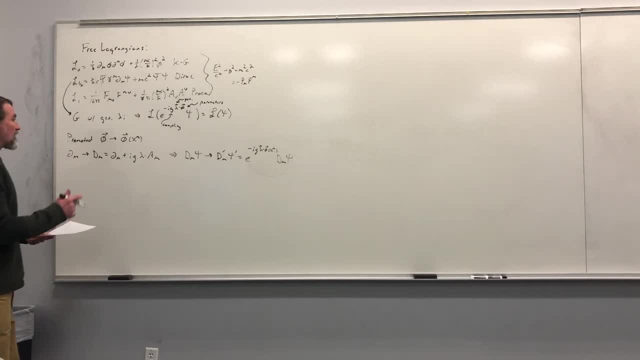 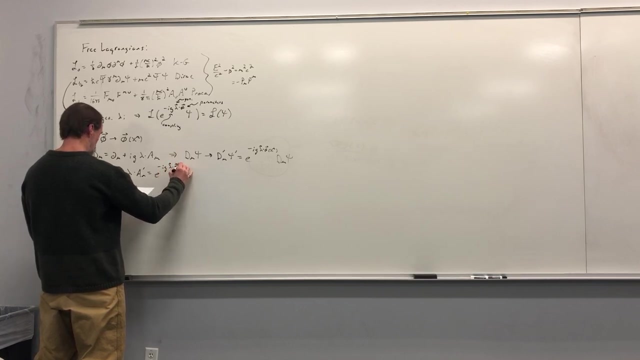 That's the way the story plays out. Okay, Now, this requires that the a mu transform in a particular way. So Lambda a mu goes to Lambda dot a mu, prime, which is e to the minus. i g, Lambda dot phi, And these are all. 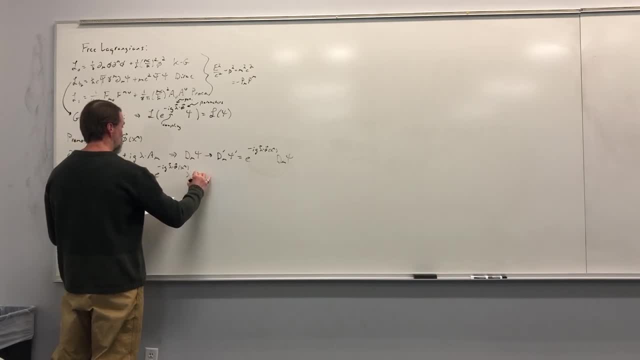 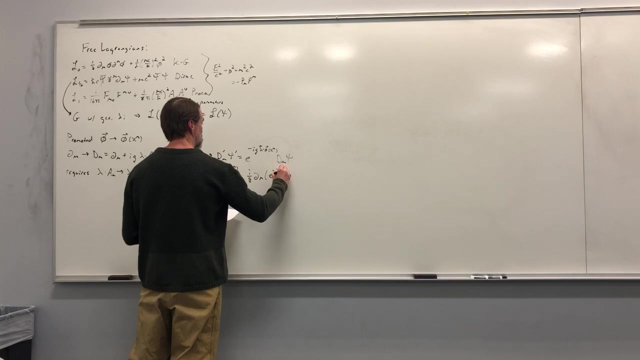 x mu's Lambda dot a mu. e to the plus i g Lambda dot phi x mu. plus i over g d mu. e to the minus i g Lambda dot phi x mu times. e to the i g Lambda dot phi x mu. Okay, Now an interesting question. 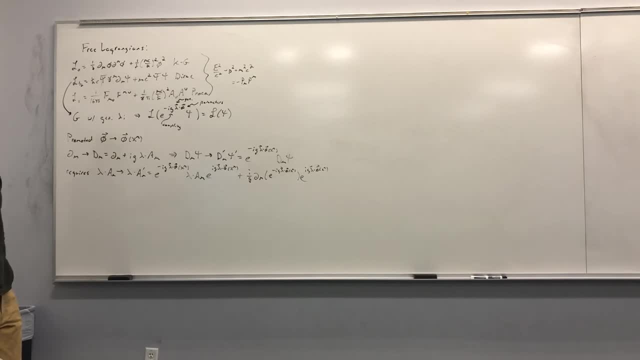 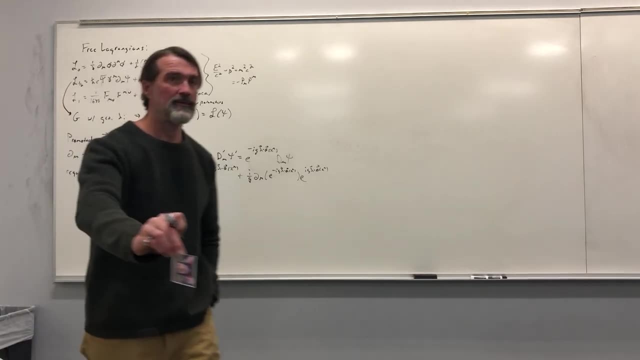 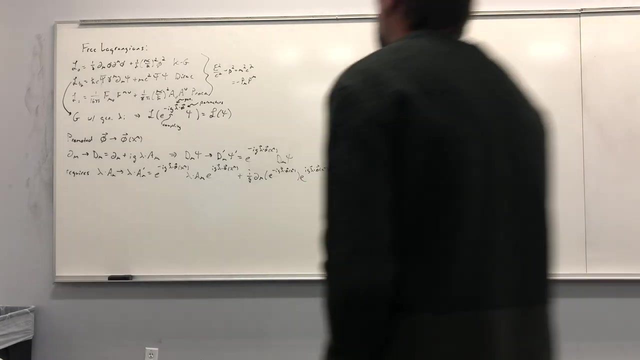 which I'll just ask our newcomer to the card deck, because he just sent it to me, Tanner. Yes, Tanner, Do you want your card? Do I want my card? Yeah, it's a pretty cool card, isn't it, Tanner? if this transformation of psi 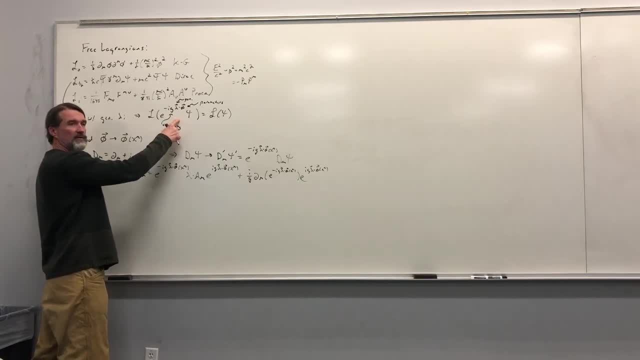 this is actually what we call the fundamental transformation representation. This is the transformation. and to get psi to transform- and we just multiply it by this- And to get a to transform, we don't just multiply it by this, we do this on one side. 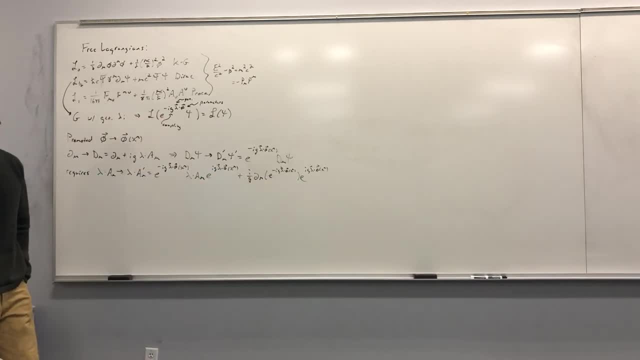 this on the other and then we have to do all this crap. Any idea what the name of that transformation representation might be. The first one was a fundamental transformation. If I said we just multiply it'sriver xt times alpha-i. Fundamental transfer. 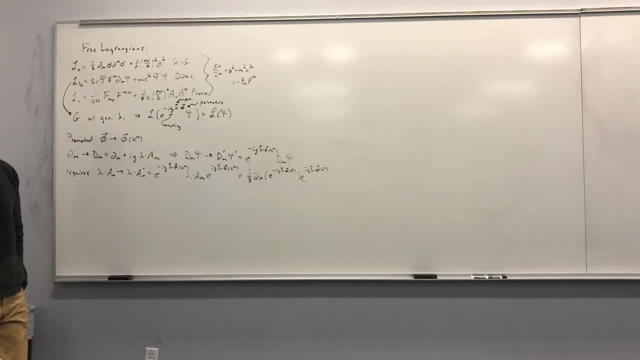 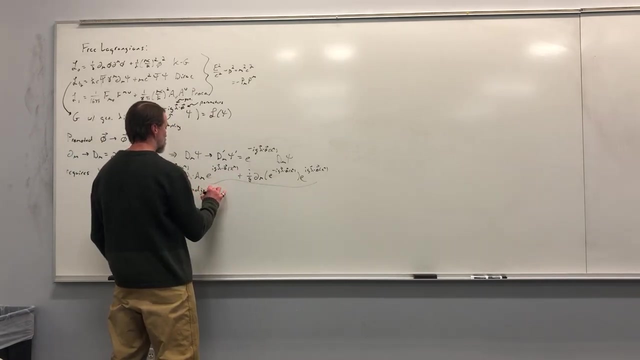 Yeah, this is fundamental. So what might this one be? I'm not sure. Yeah, because I haven't told you guys. Good, good, I'm glad you couldn't answer. This is what we call the adjoint representation. Okay, no one asked, but that's the answer to that question. 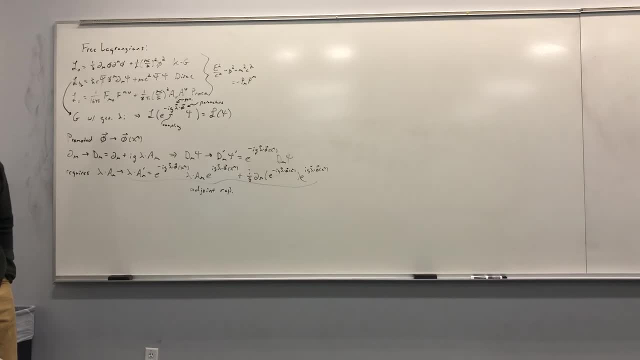 Should somebody then cool off and ask: No, you can keep it So to allow the new gauge fields to propagate. okay, so this is how the gauge field must transform. Now, we wanna allow the gauge fields to propagate because right now we've got this new derivative. 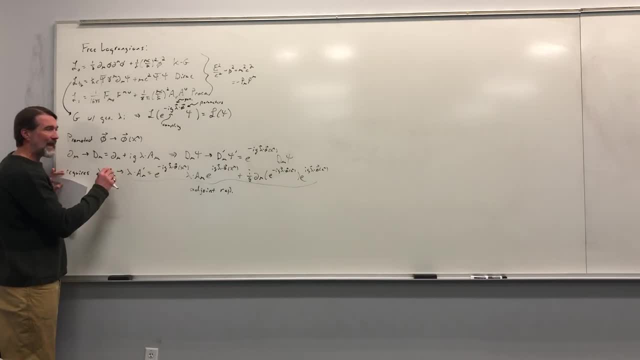 the theories invariant under these local transformations. We're gonna have interactions between the psi and the a. However, the a is just a background, It can't act. There's no dynamic, It doesn't have a kinetics of a, It doesn't have a kinetic term. 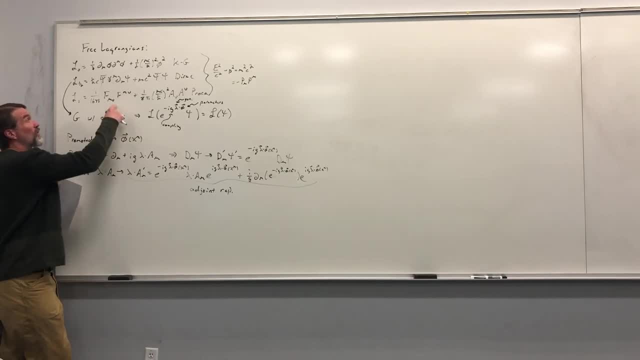 But if we wanna add a kinetic term for a, we should pick the Proca, because the Proca is the kinetic term for a spin-1 particle. okay, So we add the Proca term for dynamical a And that's gonna be one over 16 pi. f mu nu. 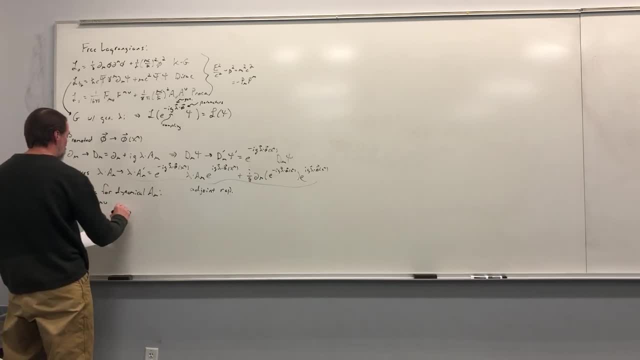 with f, mu, nu equaling minus i over g times the commutator of the covariant derivatives. okay, Notice, I did not add in the whole Proca term, because it turns out that because the a's transform in this adjoint manner rather than in this manner, 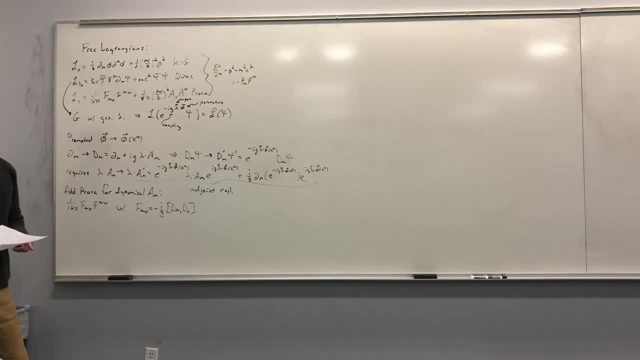 this term is going to be an adjoint derivative. This term is not invariant. okay, That's important because, like, if I consider psi, bar, psi, this term is automatically invariant under this transformation because psi, bar just gets e to the plus, i g, lambda, dot, phi and psi gets e to the minus. 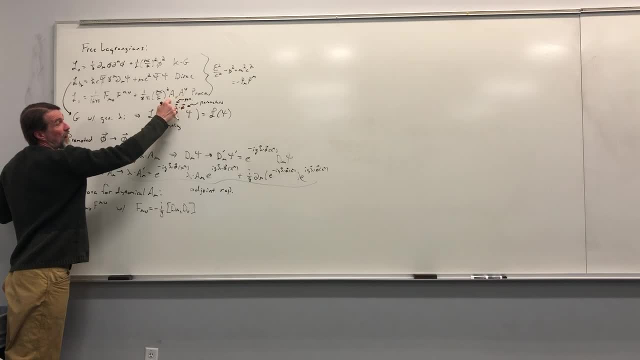 And so you just multiply this and you're gonna get one This. you might also think: oh, it does the same thing, except a doesn't transform like this. A transforms like this. okay, So this is not invariant under this transformation. 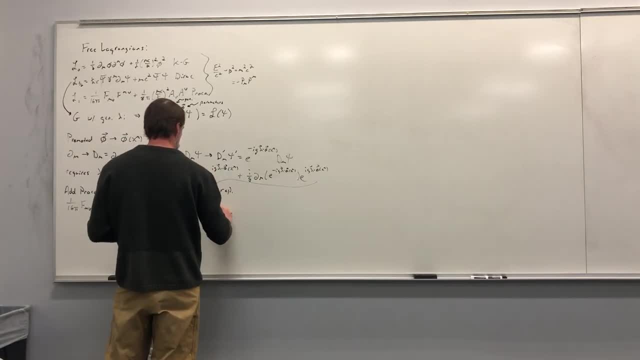 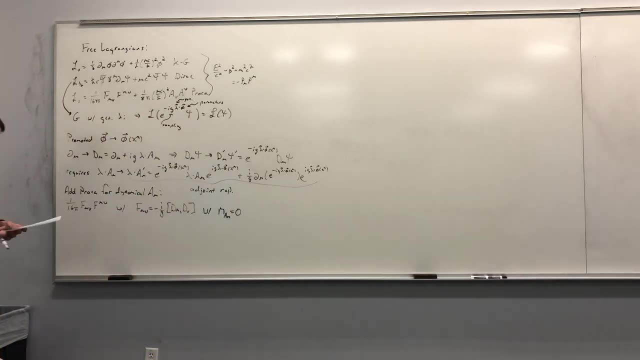 so we have to set the mass to zero. Okay Now, if we do that, then I can just give you a very quick survey of what we use. in the standard model For E and M we use u one on the complex psi. 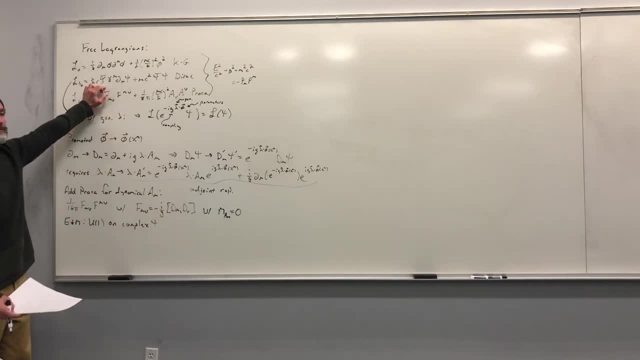 That is, we don't have to do anything to this to get electromagnetism, because the spinners are already complex and so I can talk about multiplying them by a phase. So if I make that phase local, then I get electromagnetism. 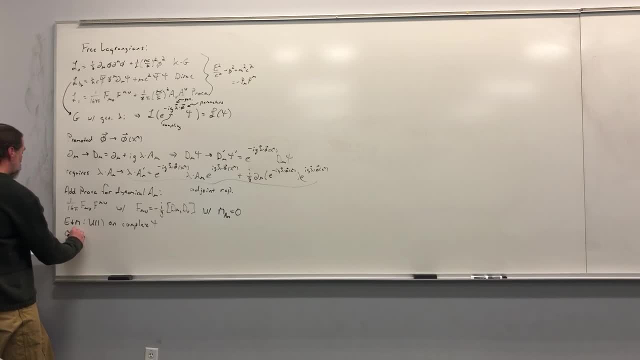 So that's kind of built in For QCD. that's the strong interactions We have. SU3 acting on size, which have three components: There's the red component, the blue component and then the green component. So we have to go back to this starting point. 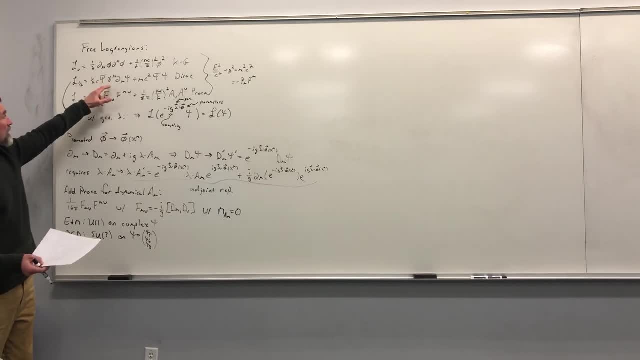 and the global symmetries of SU3 and say, okay, they have to work on three component things. so these sides have to become three component objects, Okay. And then for electroweak, we find that the symmetry group, in this case, 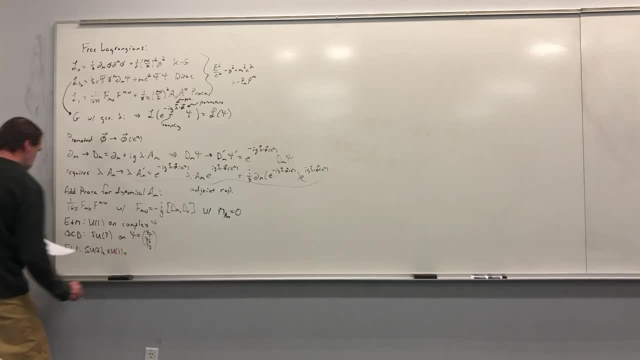 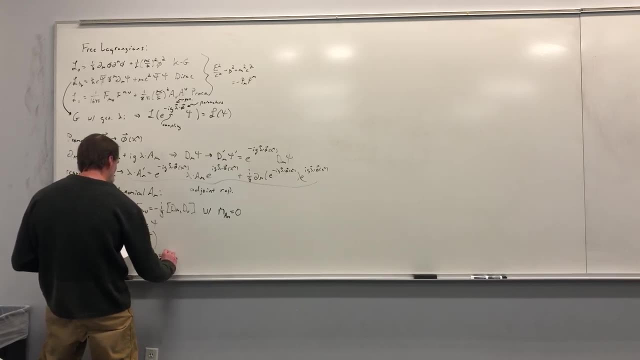 is SU2 left. cross u one hypercharge, okay. And this acts on chi left, which are the sets of doublets and then er et cetera. Okay, So the SU2 left acts on these doublets. These are two by two matrices. 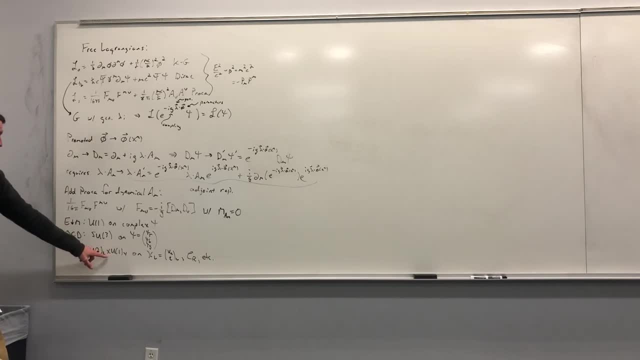 so they have to act on something with two components, Whereas we also have a u, one hypercharge, which acts on the left and the right For the right. we just need this single state for it to act on. okay, In fact, in this slide, 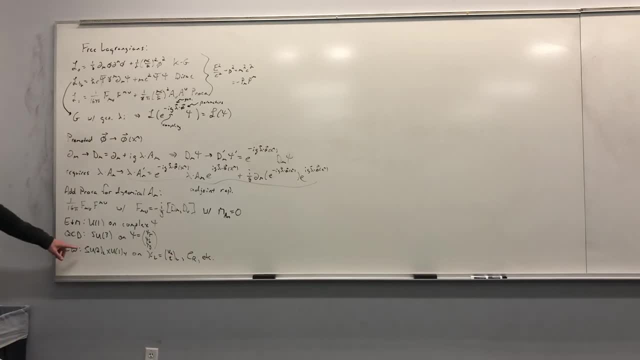 I want to show you guys some arrival show problems- maybe little side- and then I'll go through them and discuss how they work as a simplification. But again, around everything now there's a lot of things that we got to look into. 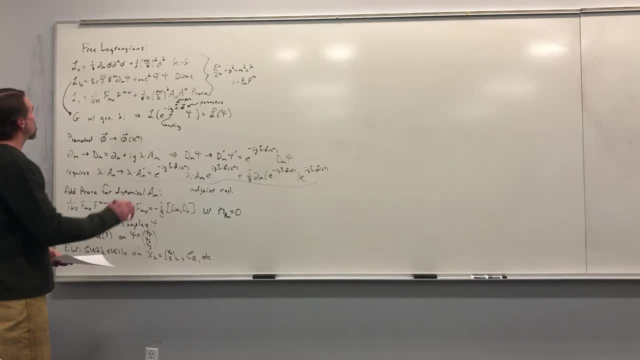 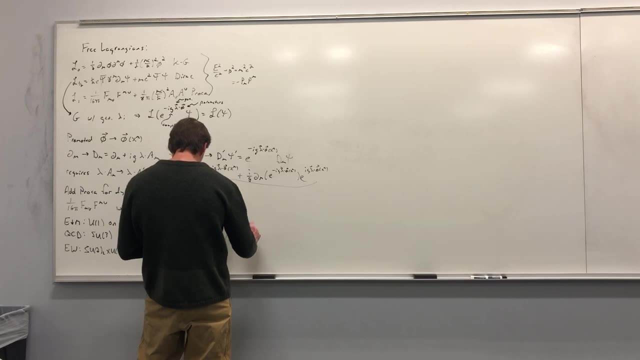 we just haven't sorting them out, but we could just try do a little step by step to see what they really are. But over time some of this will come along. We do think these are possible, theoretically. In fact, some people expect this fancy idea. 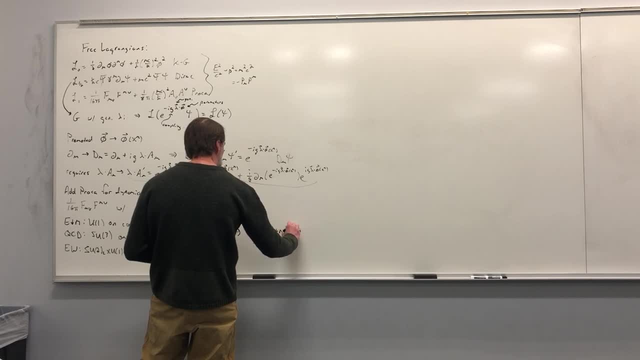 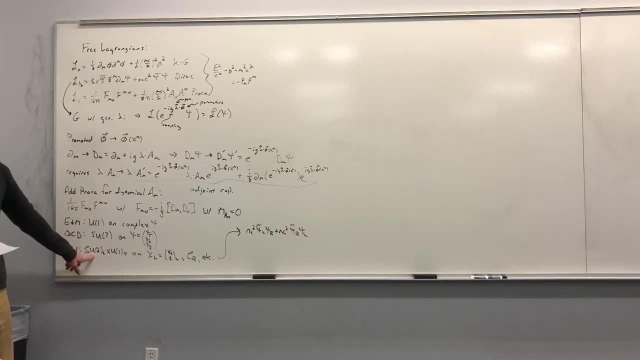 to work as, for example, two pi square sines. we'll gonna pot. we can do two, five forms, m, c squared, psi bar right, psi left. But since this transformation only acts on the left-handed components, there's no way these terms are invariant. 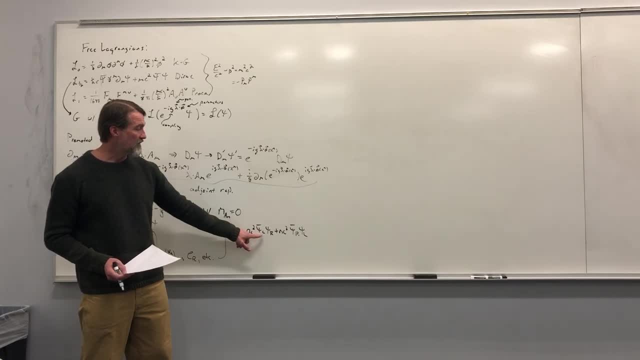 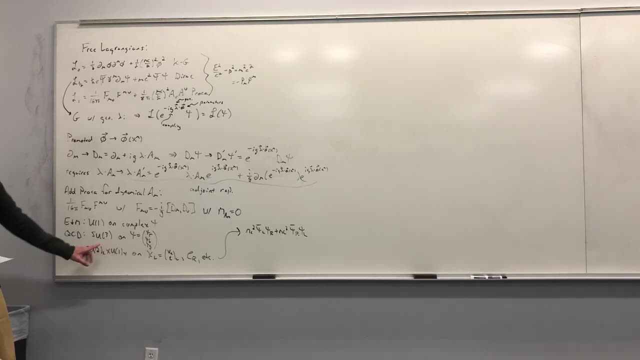 Okay, Because I would only be transforming one of them, not both of them. So that means that this symmetry right here- none of the rest of this story, just that guy right there- means that all matter has to have mass of zero. 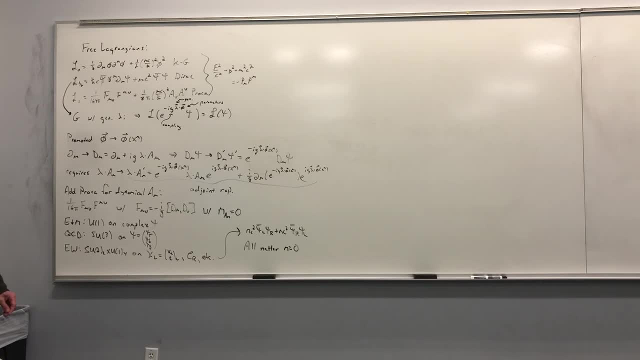 In order for this to be the proper symmetry groups of the standard model. Okay, Oh, Tanner, I see what's going on. Tanner, Which of these conclusions does not agree with experiment? The conclusion that all matter is m equals zero And. 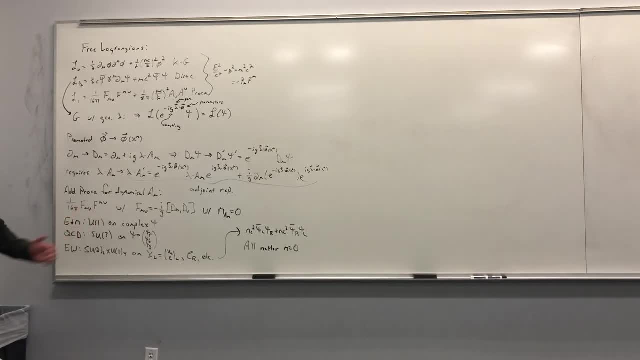 That's true, That's very true. I mean, electrons have a mass, But what else? Maybe I shouldn't ask, I'll ask somebody else, Tanner, Maybe one other one? Yeah, I'm not sure You got a phone. a friend. 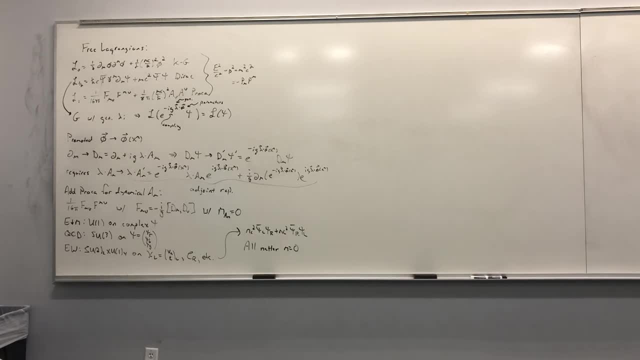 Yeah, yeah, Anybody have an answer? Yeah, I don't know. I know you have a phone. It's a compromise between us on the internet. I'm not sure if it's a good thing. We should be trying to figure out a way to argue with you on that. 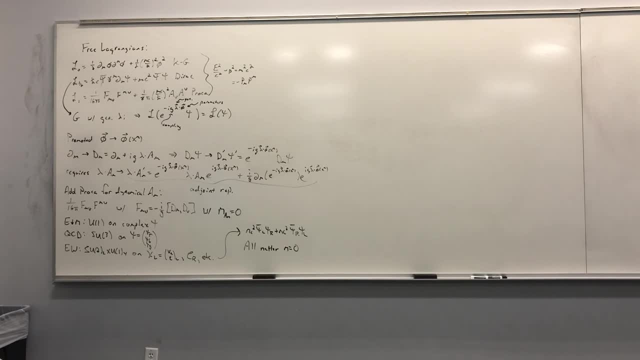 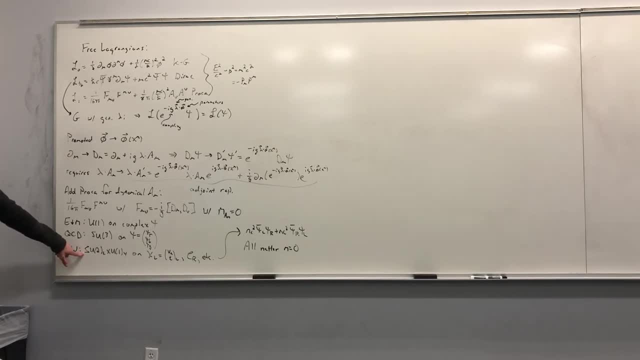 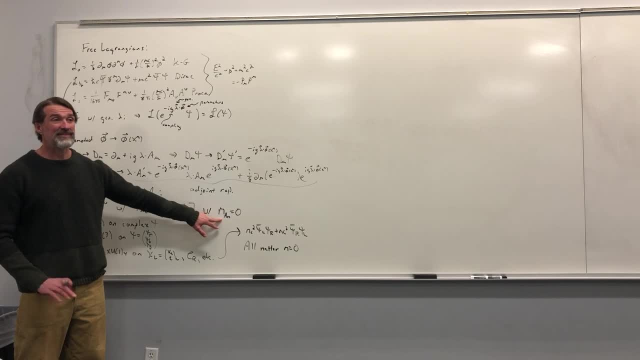 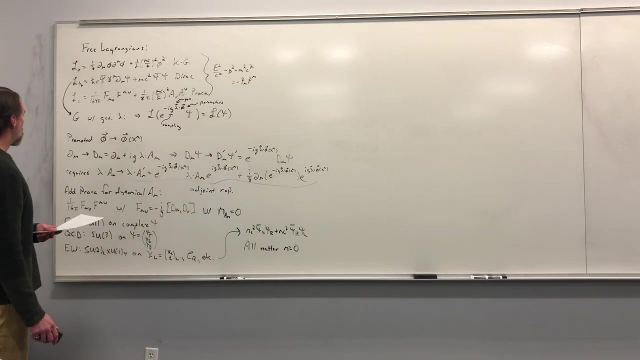 And we have to set the mass of the gauge fields to zero for all the symmetries. but that's not true either. Okay, so what we're going to start today is an exploration of fixing this. Okay, all right, I think I'll keep a little bit of this, but I'll get rid of this. 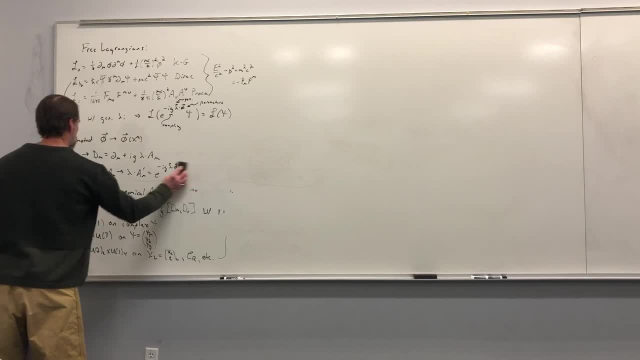 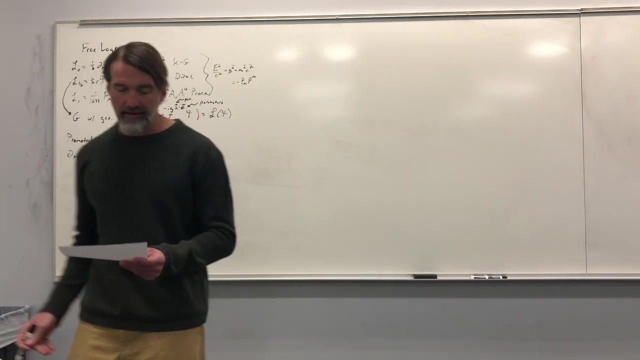 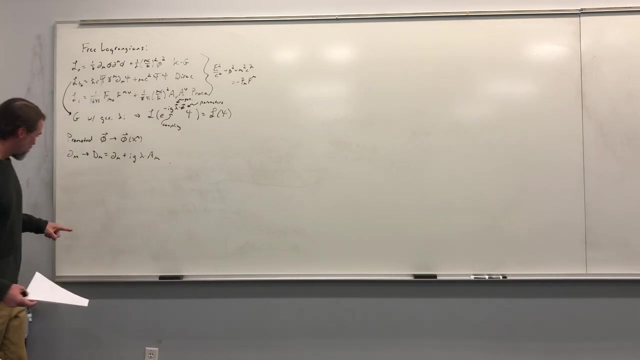 Yeah, okay, All right. so where I'm going to start? it's going to look odd, but in the end it'll play out. First of all, the problems originated from this. See it, It's that SU2 left factor. okay. 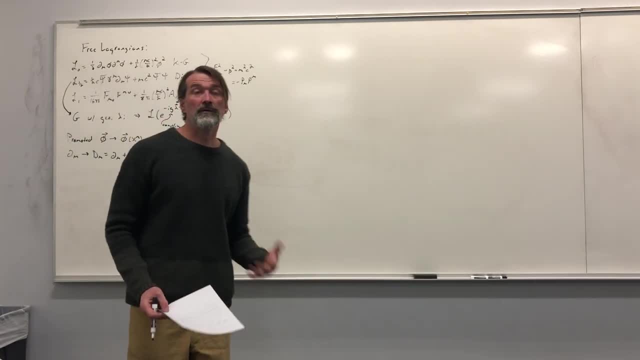 But the first version of this story I'm going to tell you, and probably the only version I'll tell you, is a much simpler one. I'm just going to use a U1 symmetry. We'll just go to an abelian case. 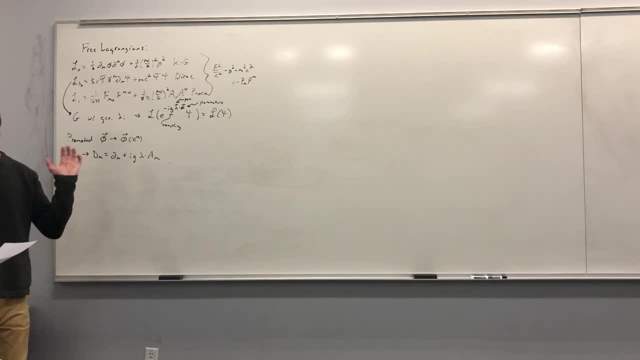 because it's a much simpler one. Okay, so we're going to start with a U1 symmetry. It's much easier to picture everything and you can actually draw pictures of it. But you can imagine at the end of the day. 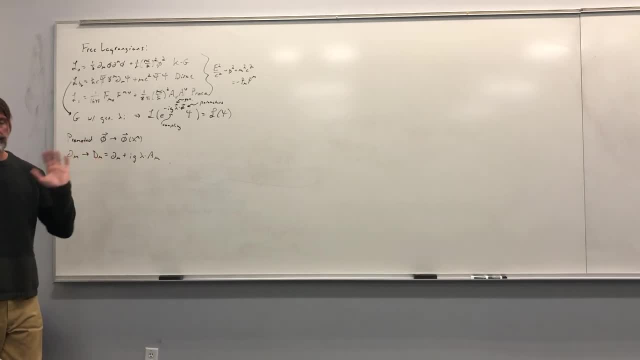 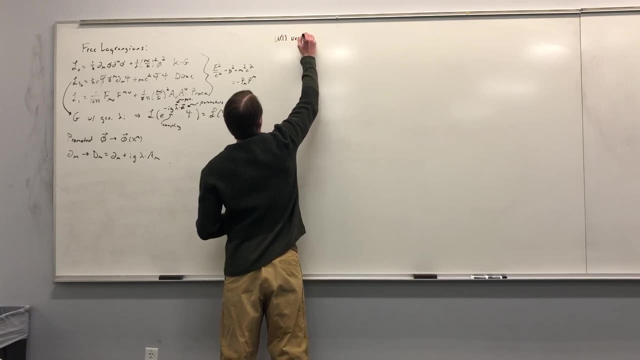 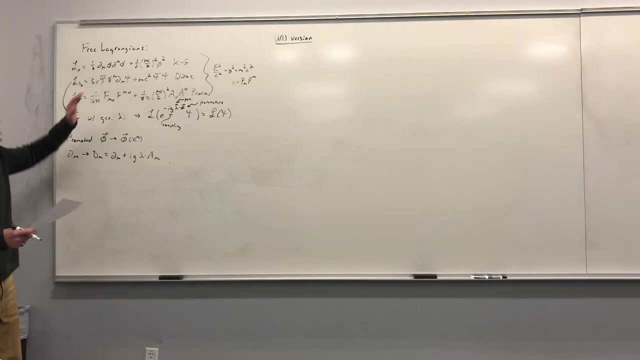 going back and putting this into an SU2 left version, but at any rate. So we're going to consider a U1 version of the story, All right, And instead of starting with a spinner field, which we're used to doing because spinners represent matter, 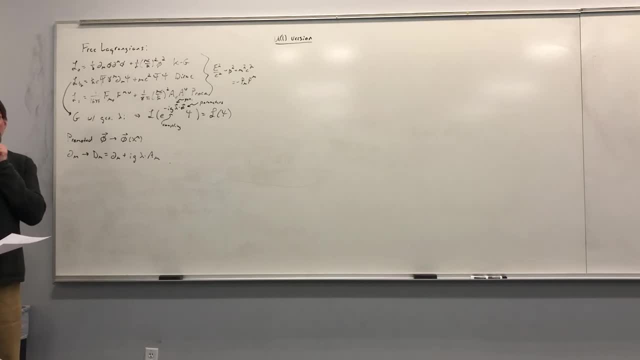 we're actually going to start with a spin zero field. Now, I'm doing this not to give you a simpler example than the spin a half field, because you've done the spin a half field so many times. that should be your best starting point. 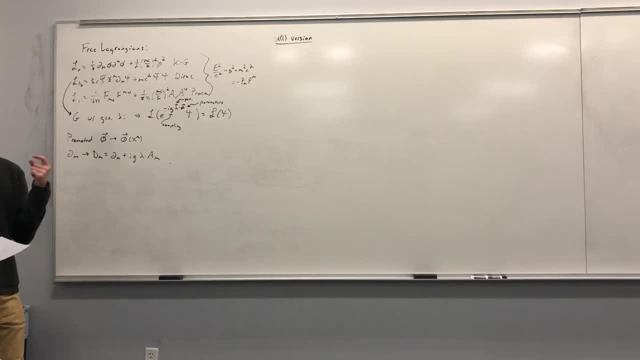 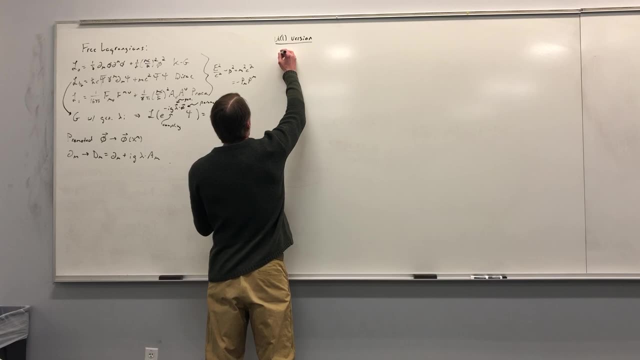 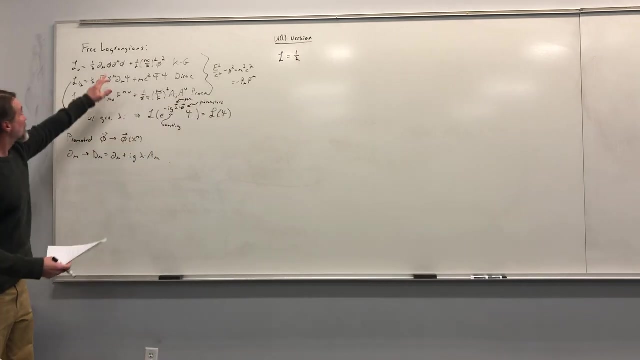 But rather what we're going to work with requires a spin zero field. So let me take the spin zero Lagrangian, and what I'm going to do is I'm going to write it as if the scalar field was complex. So I'll just star the first of the phi's. 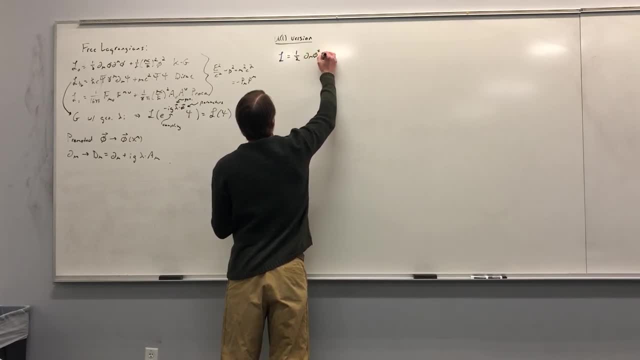 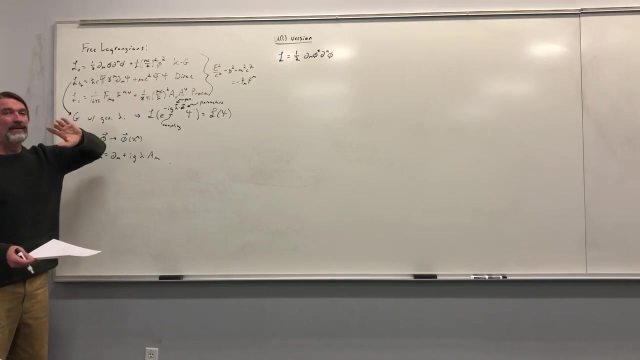 So we'll start with d mu phi. star d mu phi. Okay, But what I'm going to do to change this around is: I'm not going to put in this mass term and I'm going to add in a self-interaction. 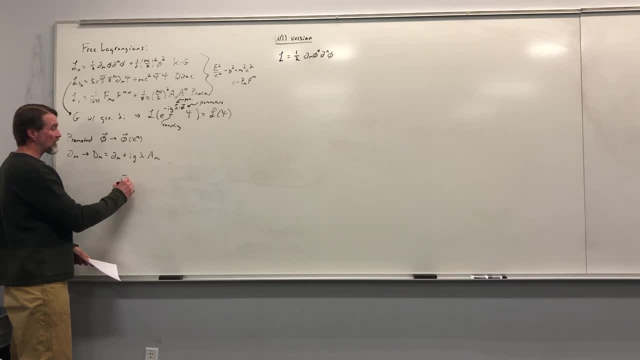 Now remember what interactions looked like For QED. they looked like this. That just says: I have the spinners. These could be the electrons and they're interacting with the photon. This is an interaction, A self-interaction- well, I mean. 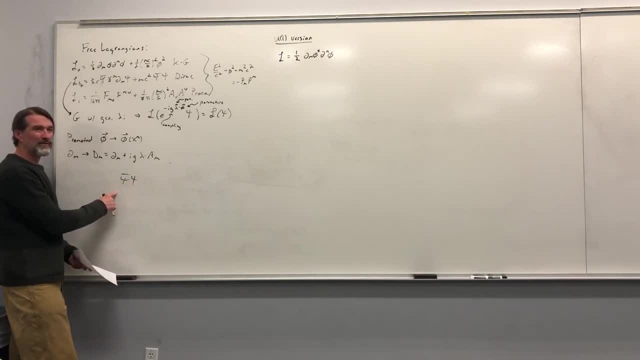 the mass term is a self-interaction, because you've got two fields multiplied But the mass terms are always quadratic and the field and they're plus. Okay, I'm going to add in some self-interactions in this story. First and foremost, I'm going to add in something: 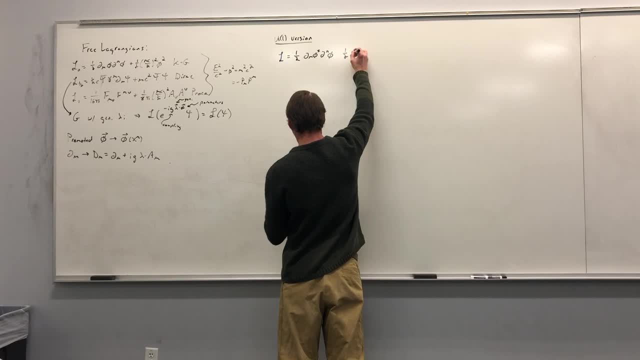 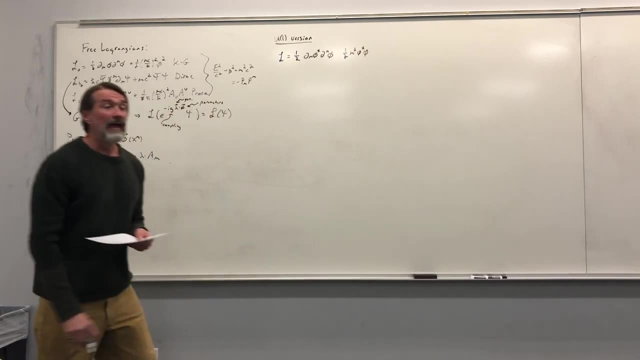 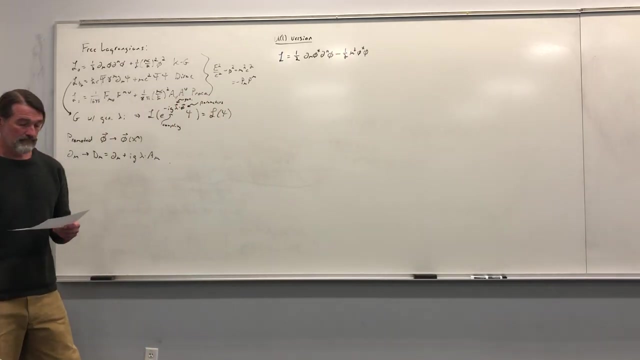 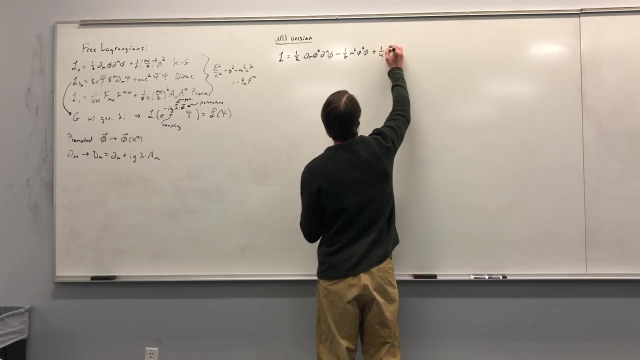 which looks a lot like the mass term. Where am I There? I am Okay, Except I'm going to make it negative. All right, But then I'm going to add in some self-interactions. Okay, And yet another term plus one-fourth lambda squared. 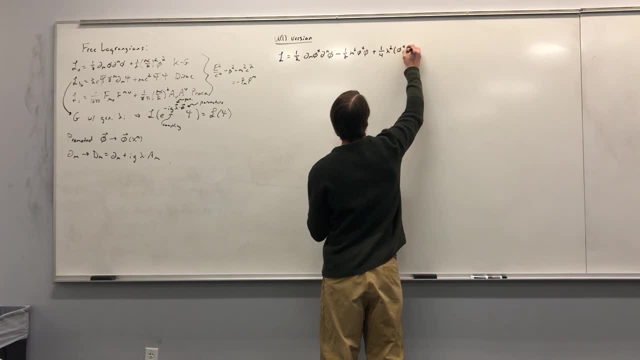 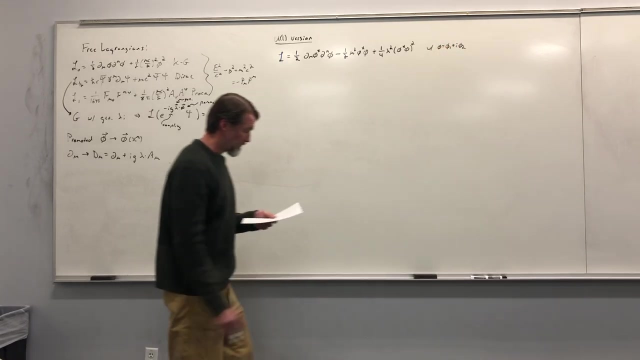 And then this is going to be a quartic interaction, That is, it's going to be phi star phi, quantity squared, Okay, Where of course we can always identify phi as phi 1 plus phi phi 2.. Okay, So this is a quartic interaction. 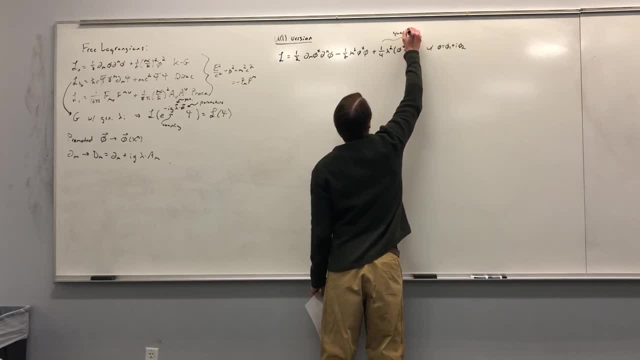 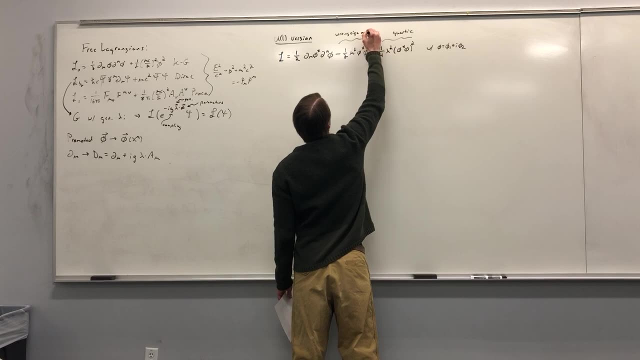 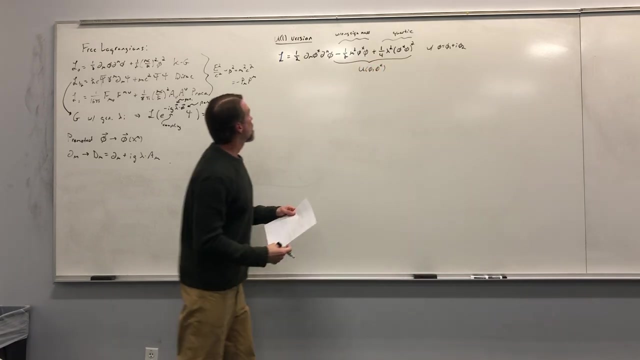 And this is what we might call the wrong sign: mass term. All right, Now what we can do is we can take all of this right here and we can just refer to this as the potential, And so this Lagrangian kind of takes the form. 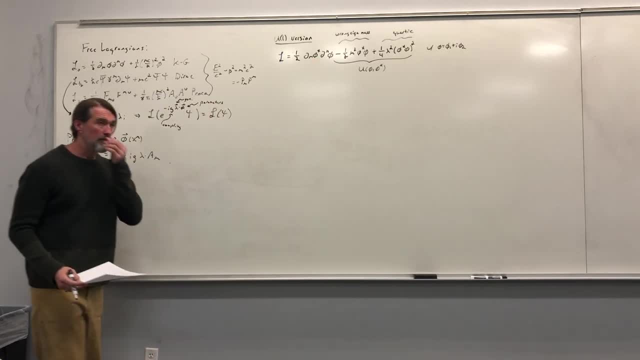 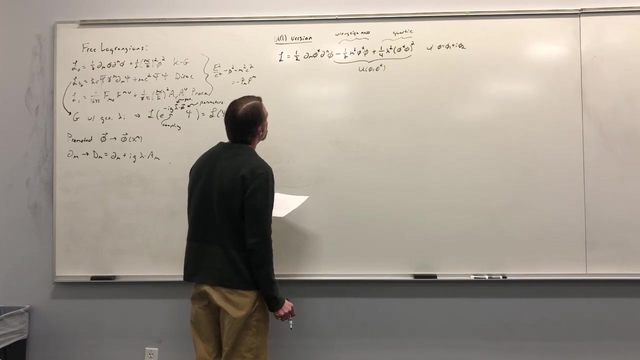 of a kinetic term plus a potential. Okay, And that distinction will be will play an important role in a few minutes. Now let's talk about that wrong sign, mass term, for a moment. Well, it's actually the correct sign. It's actually plus one-half m squared phi, star phi. 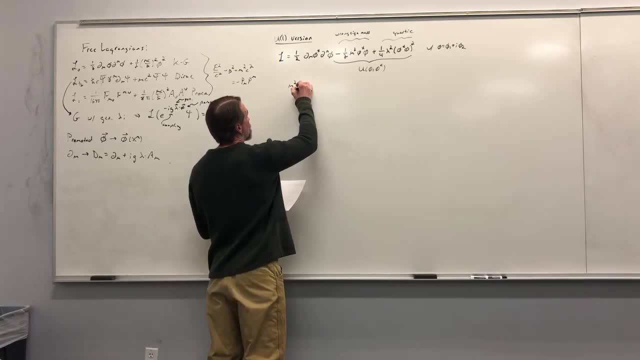 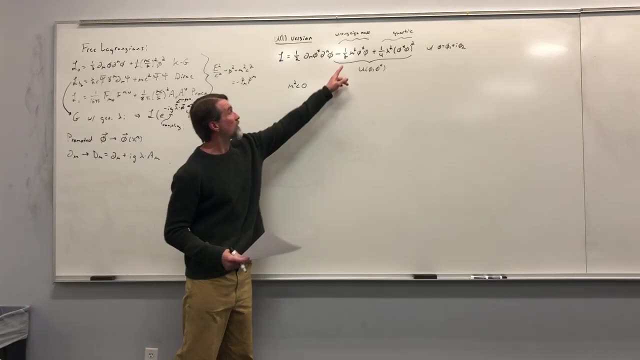 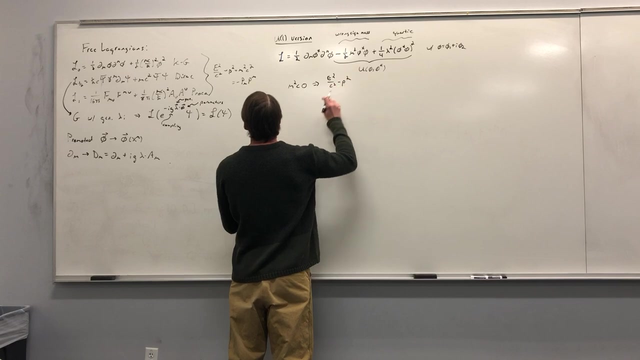 Okay. But what's important is that n? squared is a constant, So n squared is negative. Okay, Hence we call it u squared, All right? So well, let's have a look here for a moment. E squared over c squared minus p squared is equal to m squared. 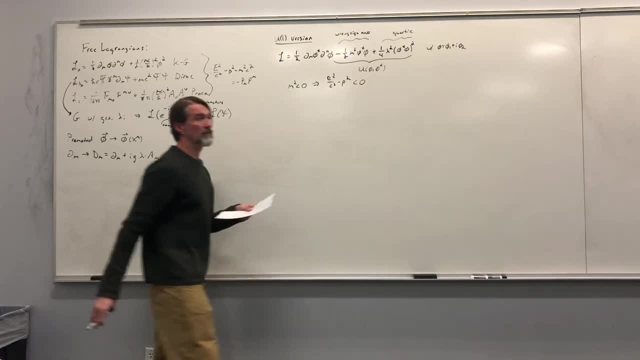 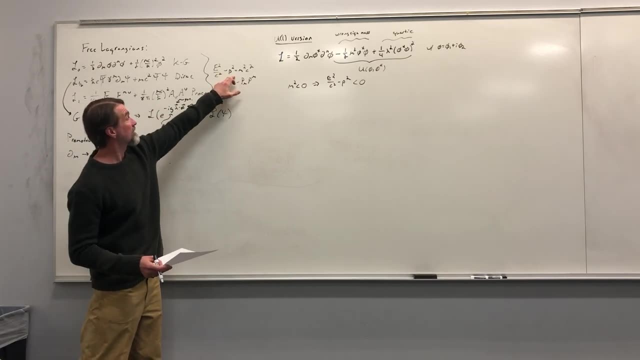 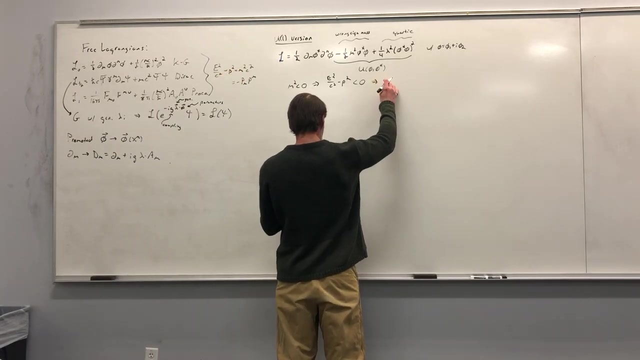 c squared, So this is less than zero. for this kind of field, Where the mass term is negative, All I'm doing is saying: it's satisfies. this M squared is negative, So it's less than zero, Okay. But if I take this and I say, okay, fine. 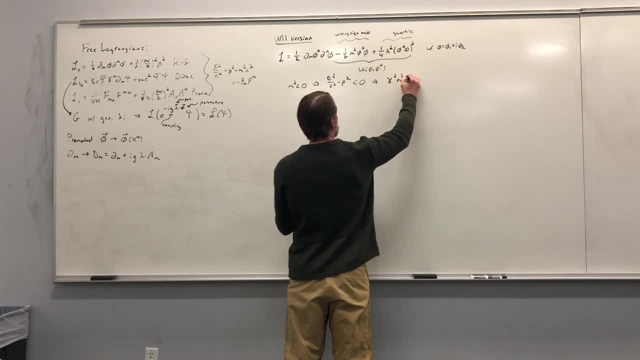 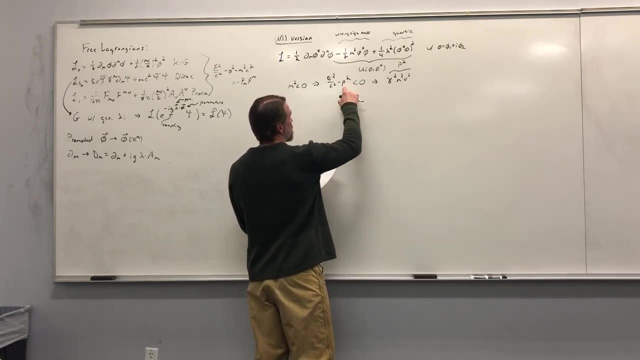 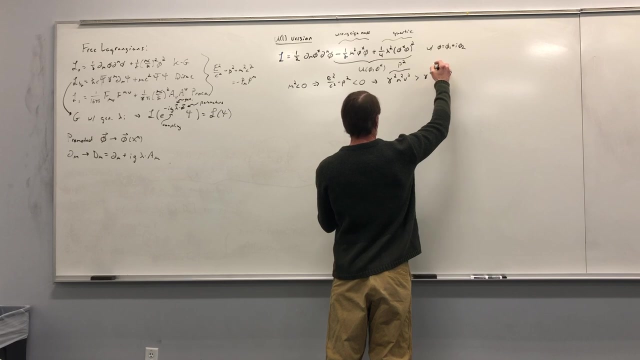 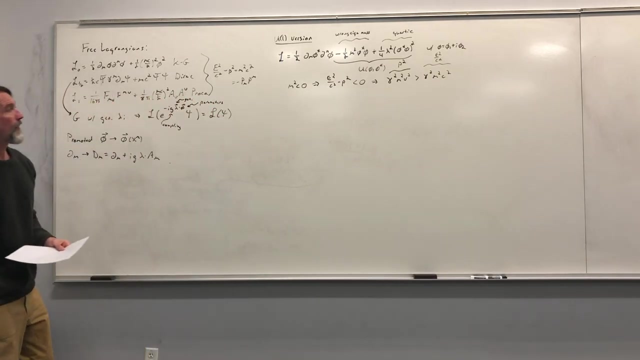 P squared is gamma squared, m squared, v squared, This is p squared. Okay, This means that this is larger than this. Okay, This is just the e squared over c squared. Does everybody understand that? I mean, this is negative, So this has to be large. 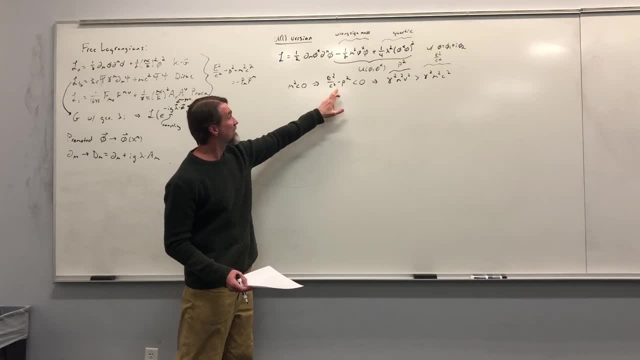 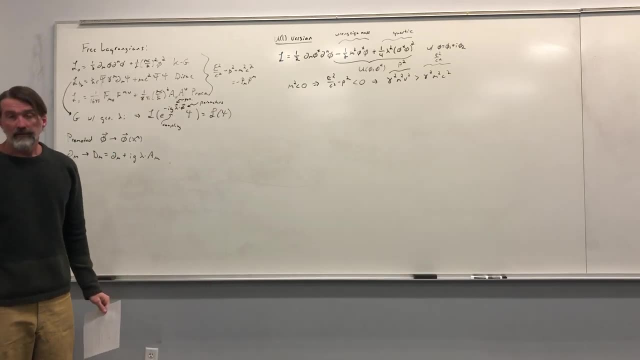 They're squared, So they're positive quantities. This has to be larger than this. So I'm just saying this has to be larger than this. Now I'm going to leave it to Tanner. I started by saying this. Tanner's not doing it. 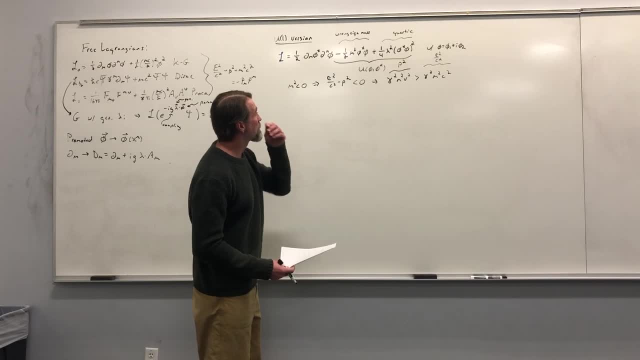 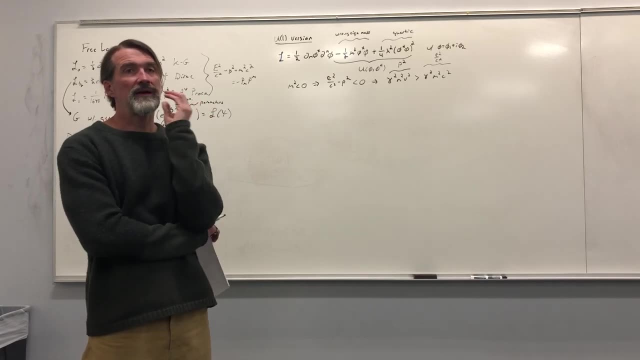 So I'm just going to do that. Tanner's not doing it, So I'm going to do that. I'm crossing the deck, that's all I'm doing. Henner, what can you tell me about the speed of fluctuations in this field? 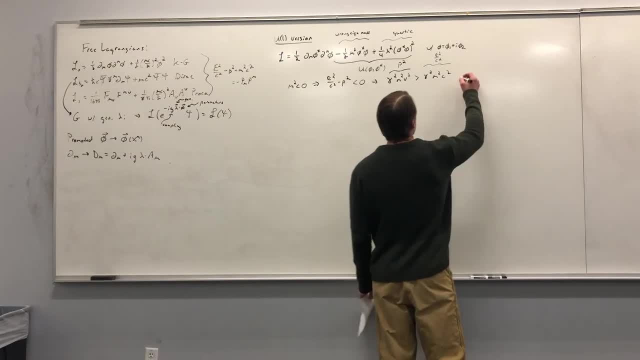 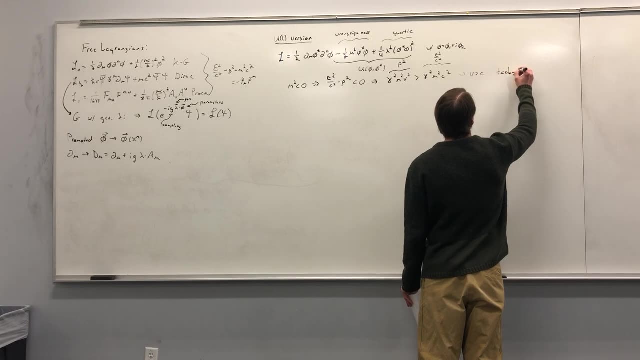 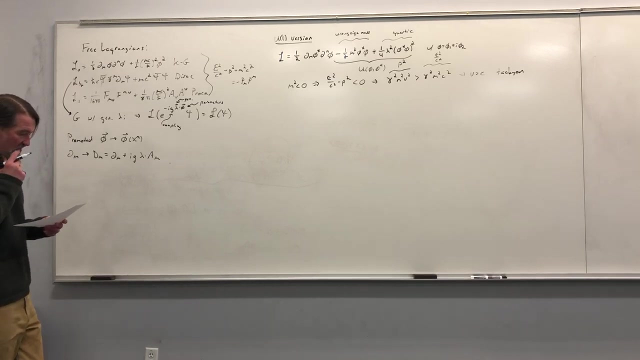 It's greater than light. It's greater than light. This is what is often called a tachyon, That is, it's a particle traveling faster than the speed of light. Again, I'm not to blame for that. I'm not to blame for that. 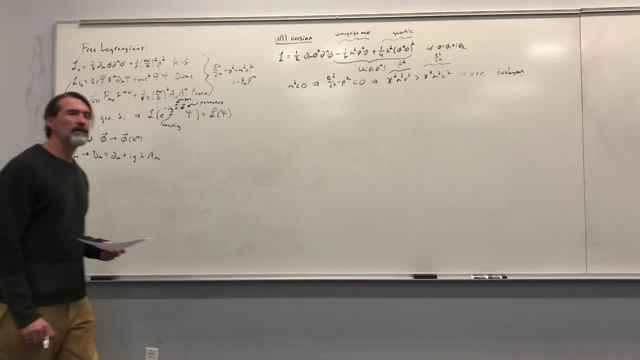 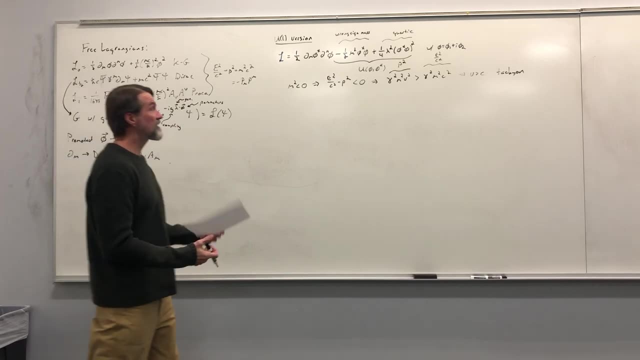 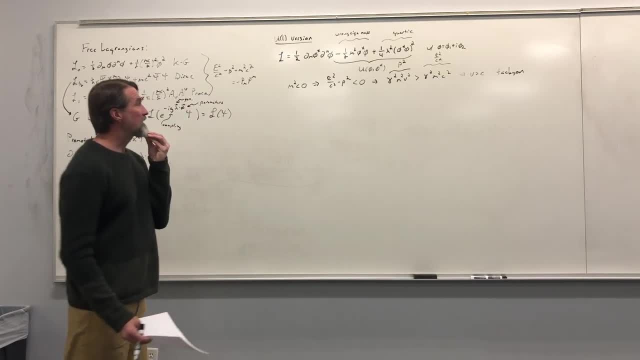 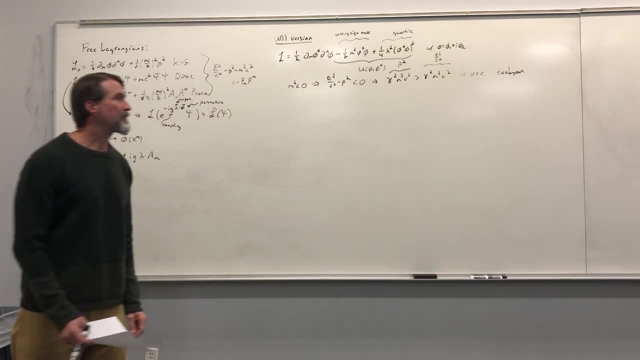 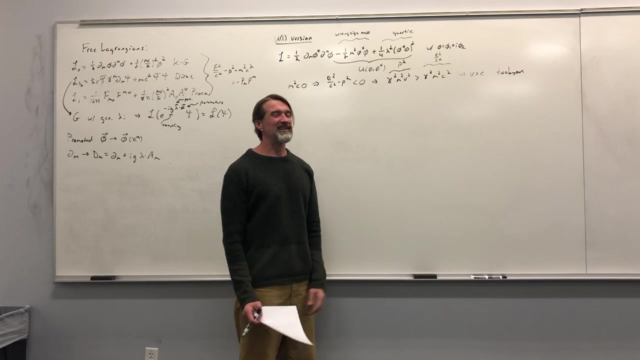 which travels faster than the speed of light. Believe it or not, there are enough people who have heard of this that they've put it into their Star Trek episodes. Next Tuesday I will be giving a talk on. the new research will give you a picture of this, for which you will say, ah shit, that's so boring things don't. 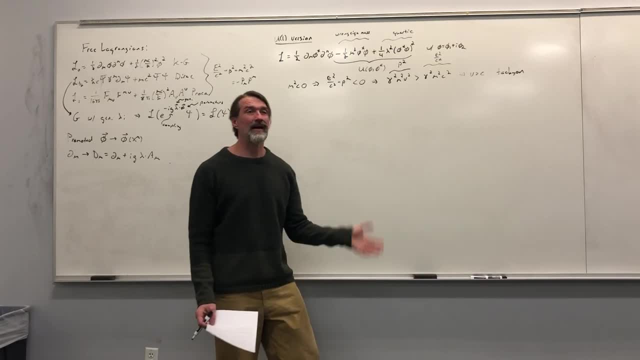 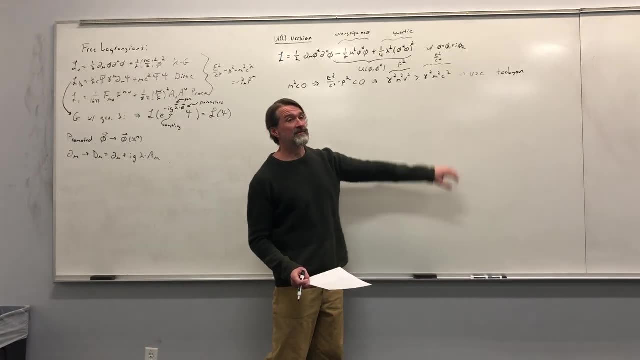 actually travel faster in the speed of light. it's telling me something important, but not that things are traveling faster in the speed of light. but that will come out of our story next tuesday, but for today there's the interesting observation that it seems like excitations of this thing. 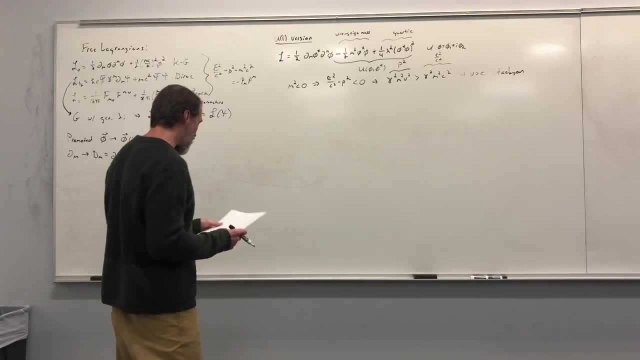 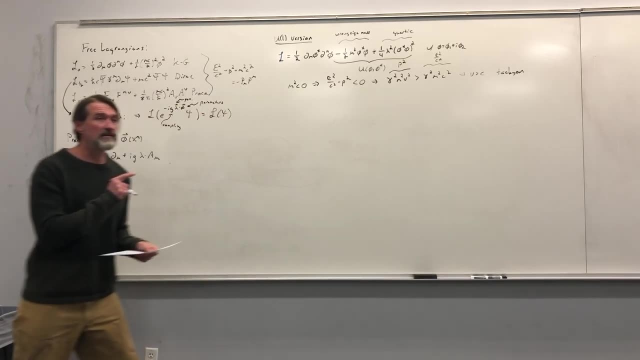 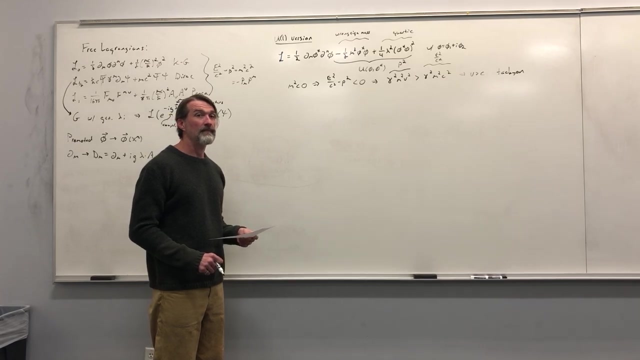 travel faster in the speed of light. okay, all right now. um, oh wait. since phi is complex, that means that we can immediately identify a global symmetry, and that global symmetry would be: oh, oh. is that the start of your answer? is that a remark? it was me trying to remember the question. so these are complex. so what global symmetry can? 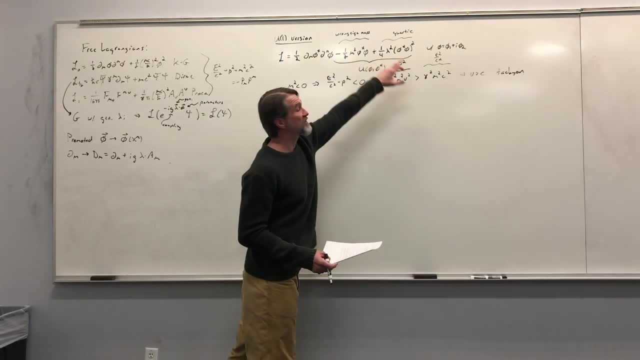 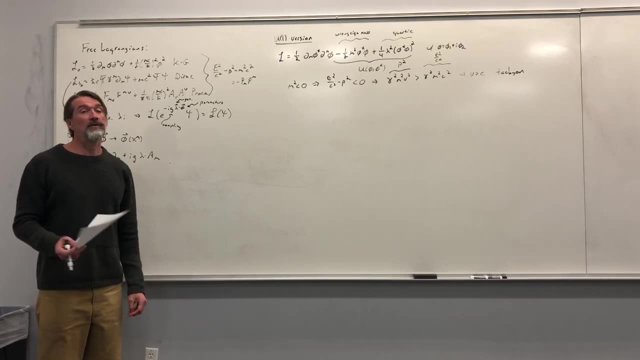 we have this is everything is star. and then the original starting in your room start. so what, what kind of transformation can you do? you can phone a friend, any friends. you don't have any friends. friends, oh, you guys. yeah, a face. so basically, you want to transfer the same transformations that 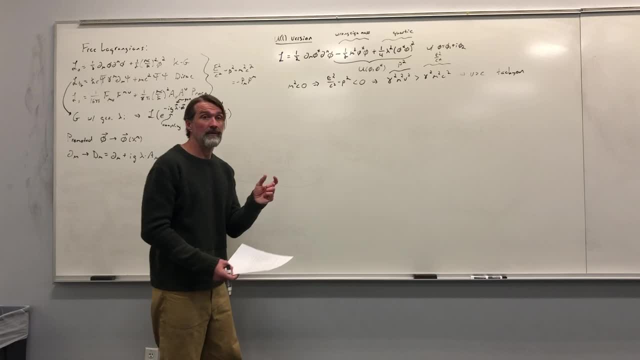 you had. you have imagine that you've had a lot of people do the things that you want to do. you're you're not planning on doing the same thing. oh, but you can do it, you can, you can do it. you can start the story and you start the process. you can start the flow, you can start the process. 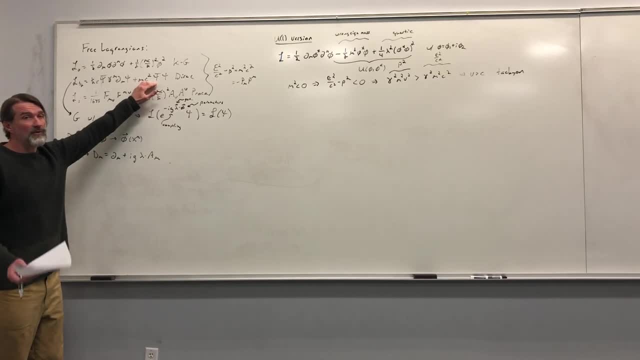 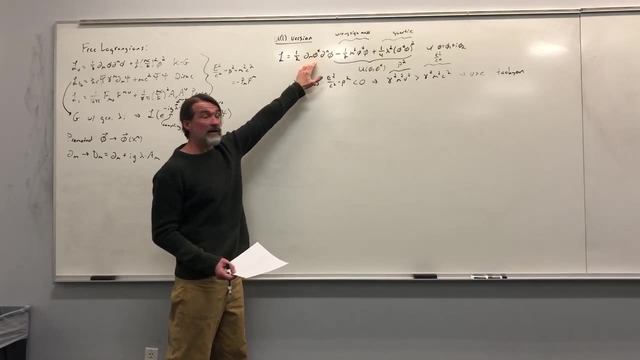 but you can start with something more complex, and so that's why you can use the form of the lagrangian to formulate electromagnetism u1s. okay, remember, for for that story we could start out with this lagrangian, and since the size were complex, we could do it without changing it at all. 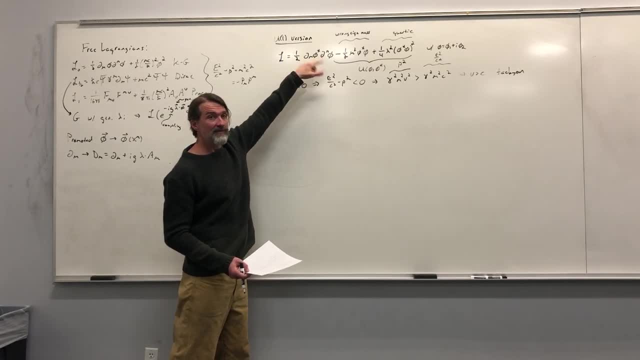 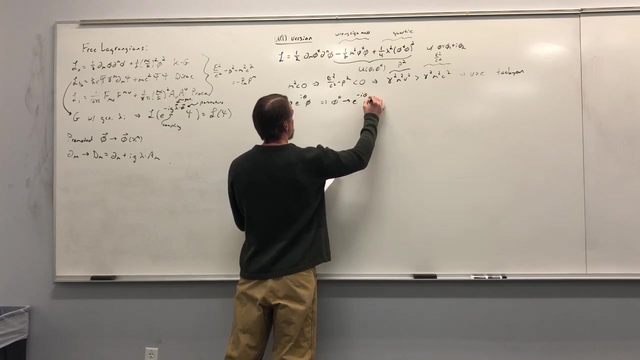 same here. since these are complex, we can immediately recognize there's a phase invariance. if i multiply a phase times this, i do the complex conjugate of the phase and then those two factors just cancel. So step one: we realize that the phase e to the i theta phi, and this of course means that phi star transforms as e to the minus i theta phi star. okay, 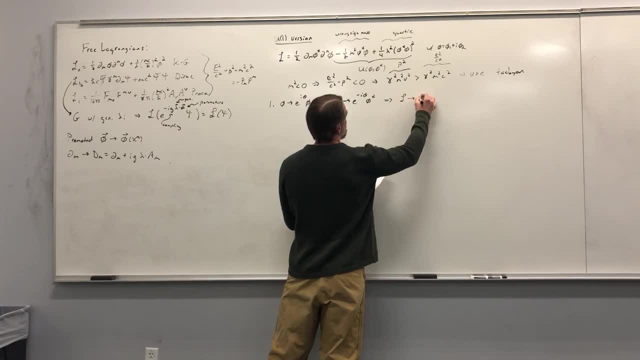 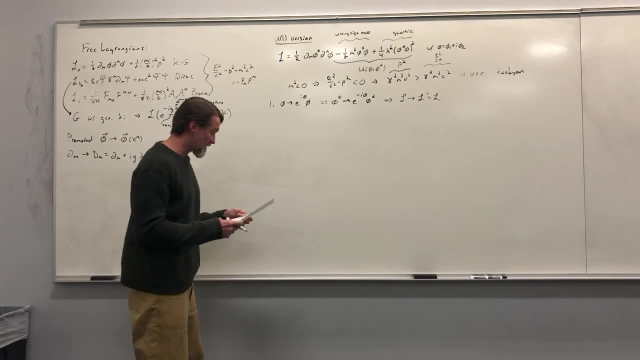 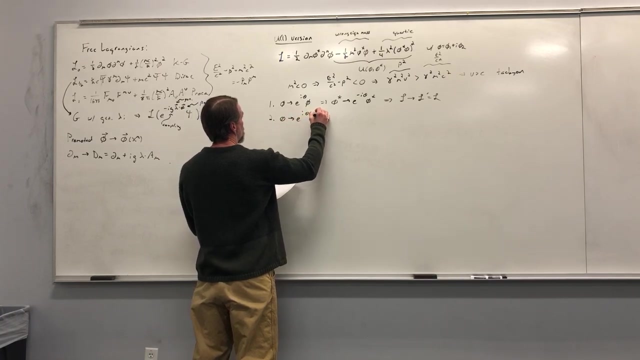 But this means, of course, that that Lagrangian up there is invariant. Okay, so this is an invariance, a global invariance of this Lagrangian, And then, of course, we can promote this transformation to a local form. all right, 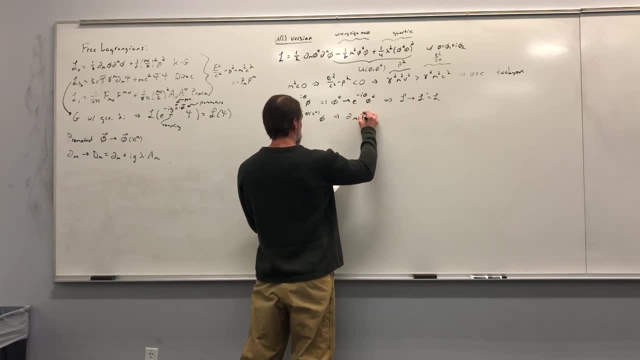 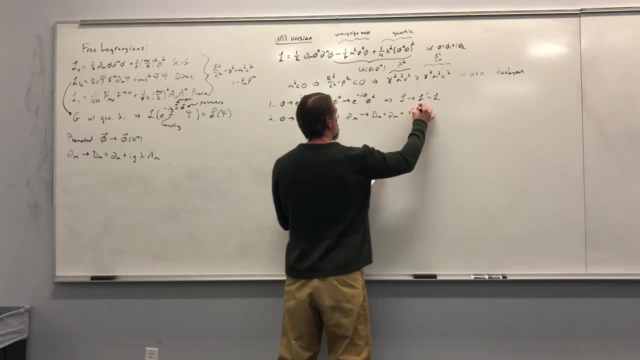 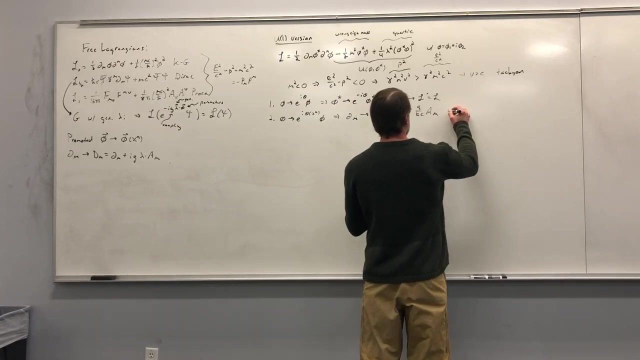 And in that case we're going to have to redefine the derivative that we're using to the following form: d mu is d mu plus i, q over h, and all of this should be a review- a mu with- and this is a nice, simple abelian story. 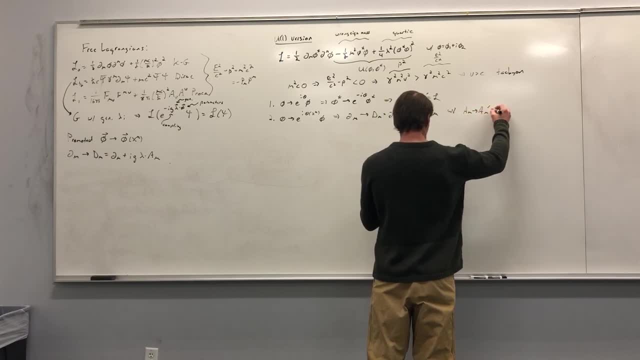 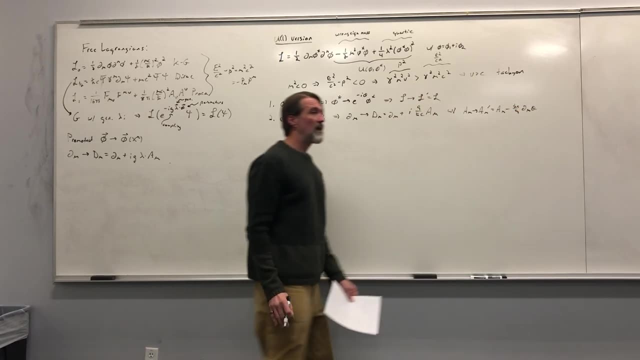 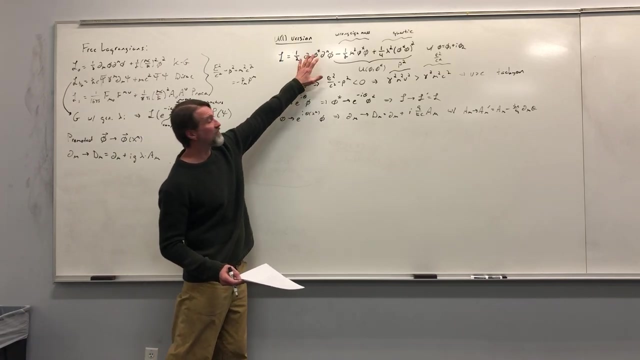 So a mu goes to a mu prime, which is a mu minus h bar of c over q d mu theta. okay, So this is exactly what played out in electromagnetism in terms of localizing this symmetry. Yeah, this is a two-derivative thing, but that doesn't really change anything, okay. 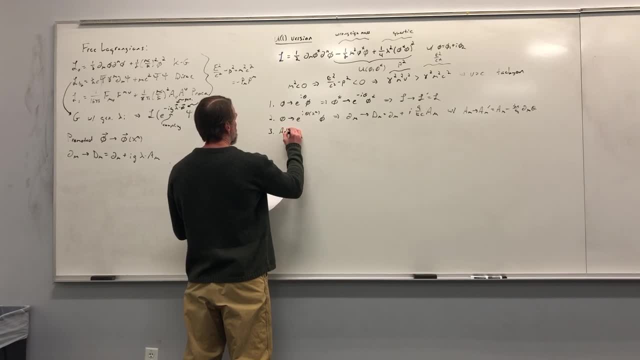 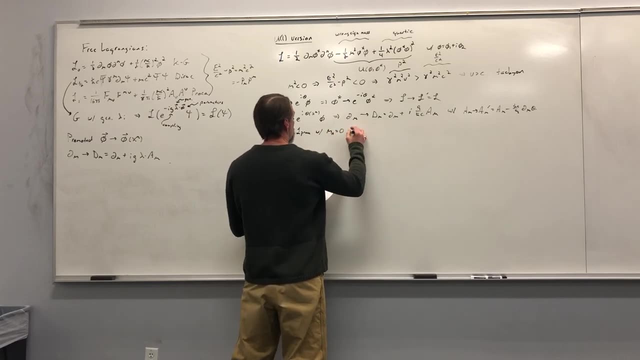 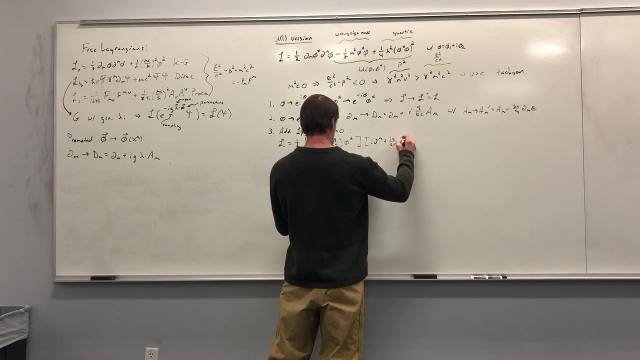 Now we add Prokha with, of course, the mass of a, To obtain the following: And now I'm going to put everything together: One-half d mu minus i q over h bar c phi star d mu plus i q over h bar c a. whoops, I've got to have a lower mu here. 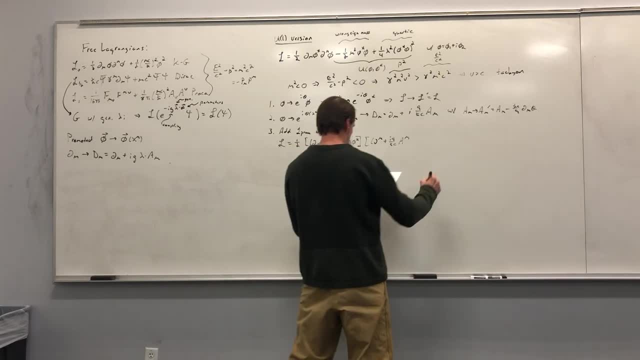 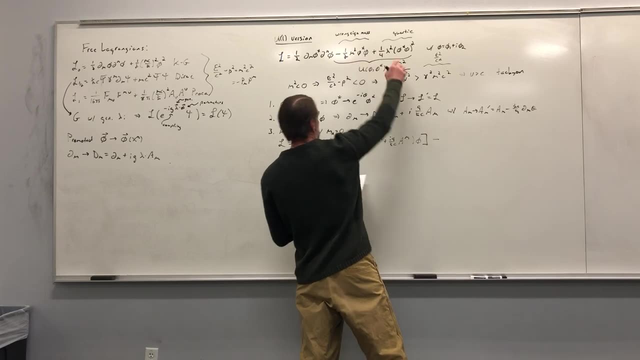 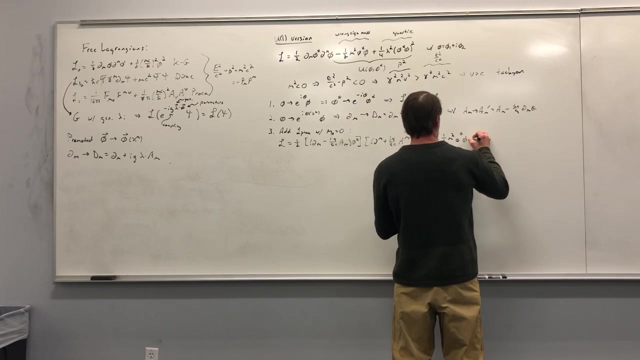 times phi. okay, And then of course we're going to just keep these terms. So we're going to have minus 1 half mu squared phi star phi, plus 1 quarter lambda squared phi star phi quantity squared, plus the usual 1 over 16 pi f mu, nu, f, mu, nu okay. 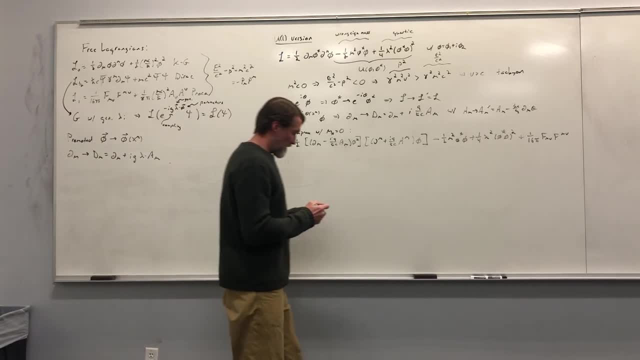 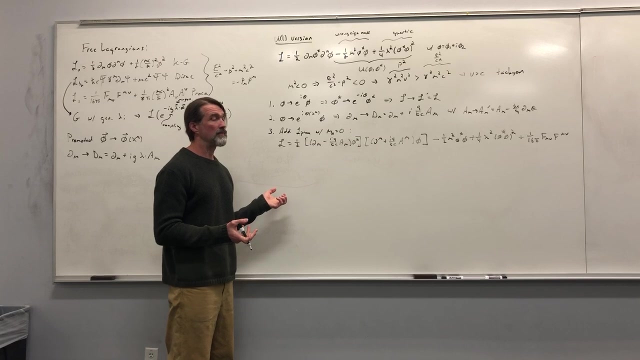 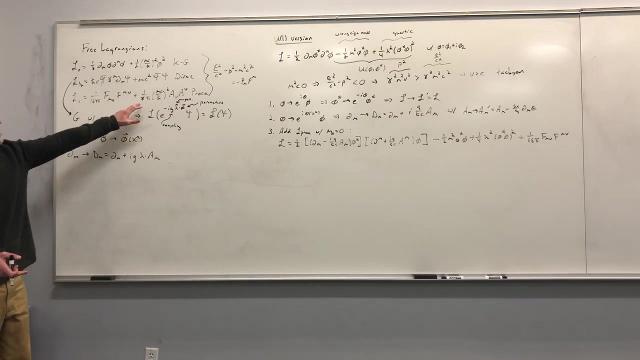 All right, So far we have a gauge theory which basically just means we have a localized symmetry. now okay, Okay. But of course, notice that the gauge field in this story is massless. It's the same way it played out for electromagnetism. 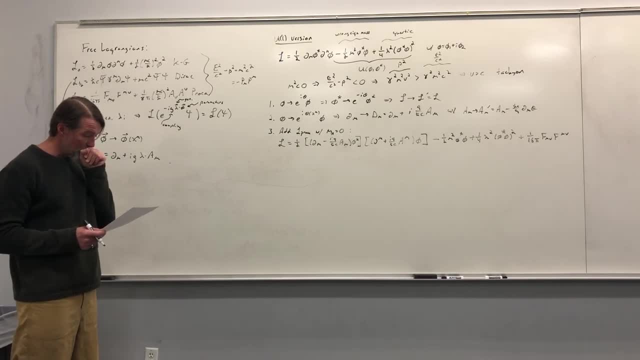 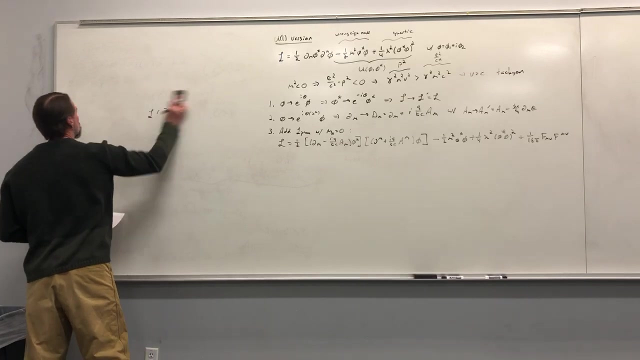 Exactly the same. So the gauge theory with a massless field. Now let me make an interesting observation. When we do particle physics, what we're mainly focusing on is: you have a field, say phi, and you're really focusing on these tiny fluctuations in the phi field. 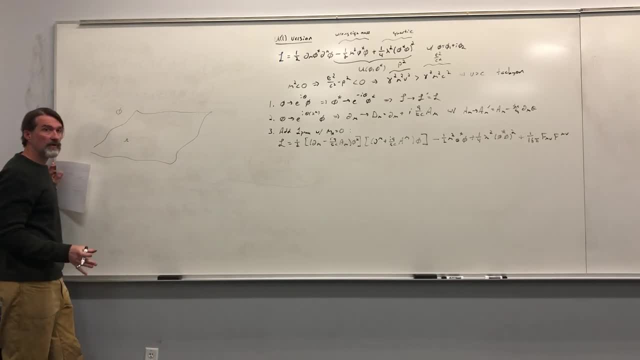 because these are the things that behave like particles, and everything in our universe is made of particles. So we're really focusing on these tiny fluctuations. Okay, Well, let me ask you a question. I'm focusing on these little tiny ripples in the field. 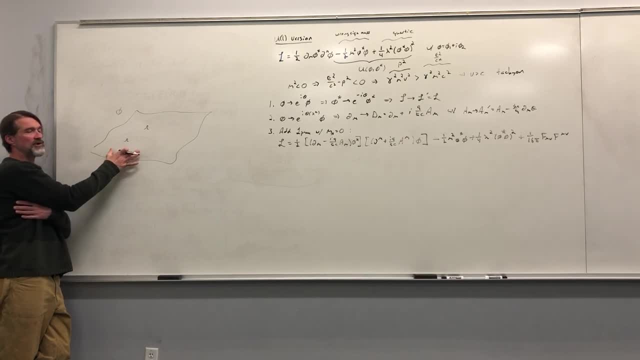 but what is the shape of the overall field? Yeah, you can always flick it Booger. Yeah, Get these little ripples and have them fly around. but what is the configuration of the overall field? Well, 99.999% of the time, we take the field to be zero everywhere. 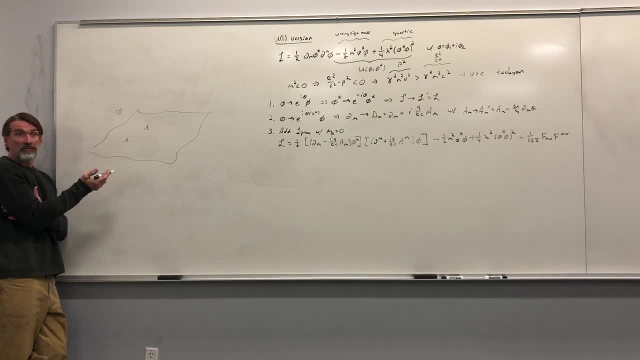 except where we have these little fluctuations. Super easy, We take the field to be zero. Okay, But do we have to? Okay, Okay. Well, you might wonder what rule is there for how I can pick my background field? This is called the background field, and then these are the fluctuations. 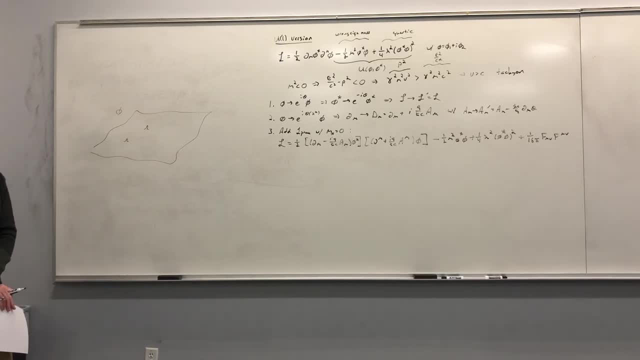 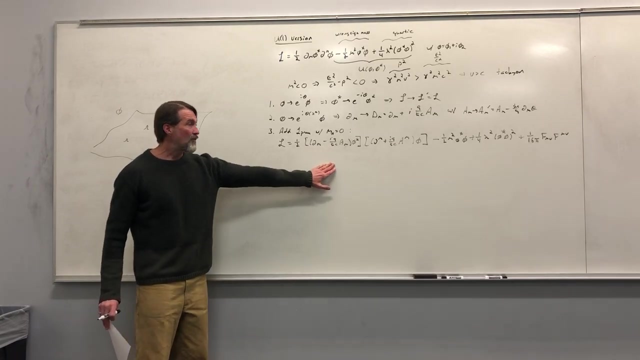 You might wonder: what rule do I use to figure out what background field configuration I can use? Well, it turns out that if we take the Lagrangian for our theory and we write down the equations of motion, these are the equations of motion that you get from treating this as a Lagrangian. 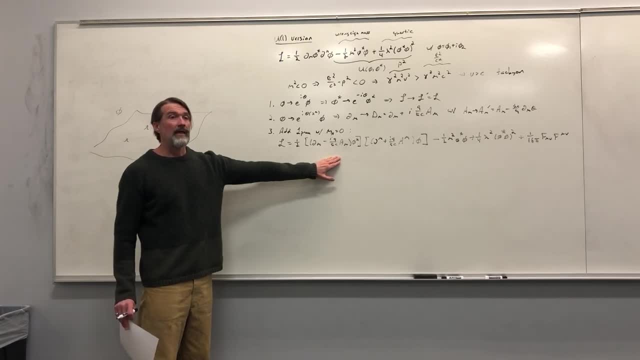 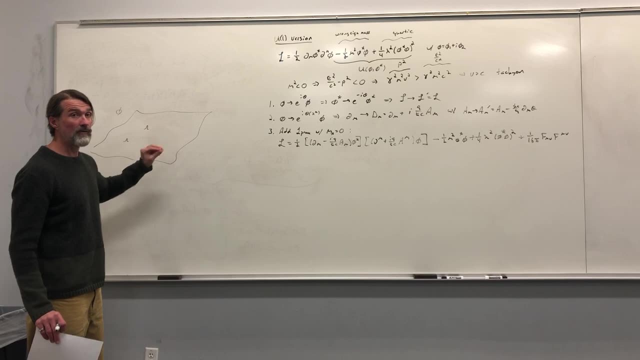 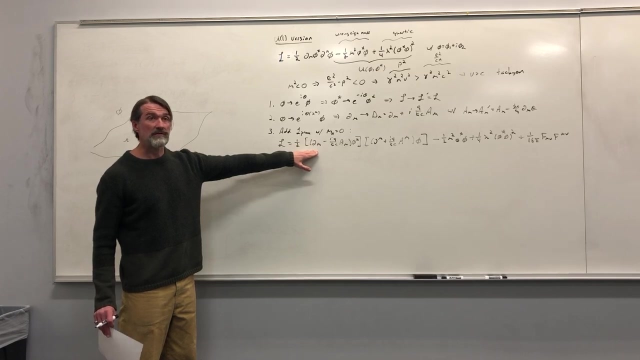 and using an action principle. Then- and this sounds perfectly classical and it largely is- because we're dealing with a whole field background, not just tiny quantum fluctuations- We take the equations of motion and we find solutions to the equations of motion. 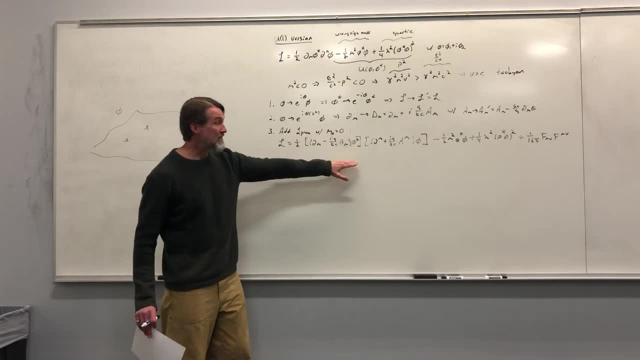 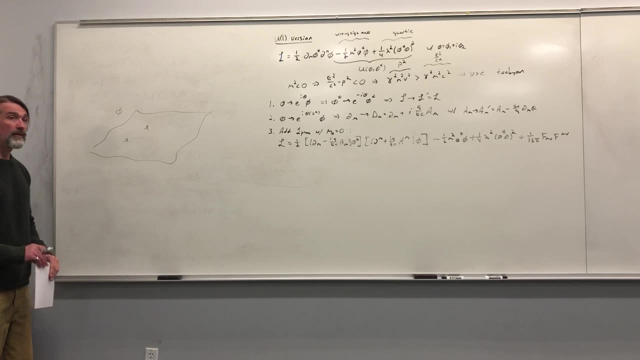 And the solutions to the equations of motion are basically: what is the background, phi and a, The. rather, if you want to figure out what's going on with the fluctuations, you have to use quantum mechanics. You can't just use non-relativistic quantum mechanics, because this is relativistic and it's field theory. 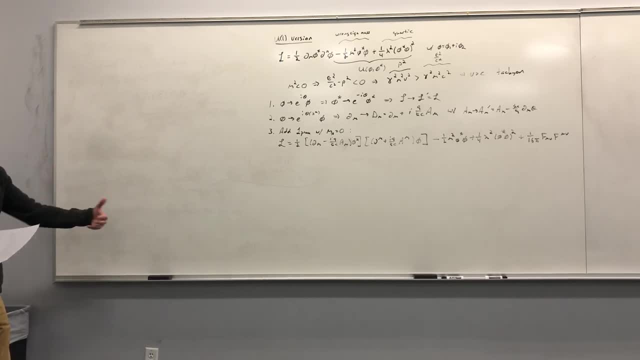 So after spring break is when we will learn how to do those calculations, But for now, we can play around with this classical calculation, because it's going to reveal something rather amazing to us All. right, So here we go. First of all, if I write the Lagrangian as a term, T plus a potential. 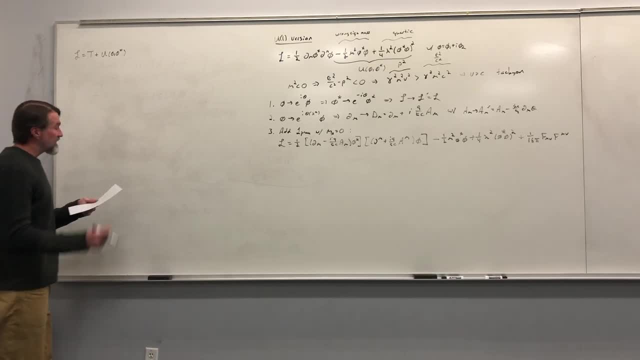 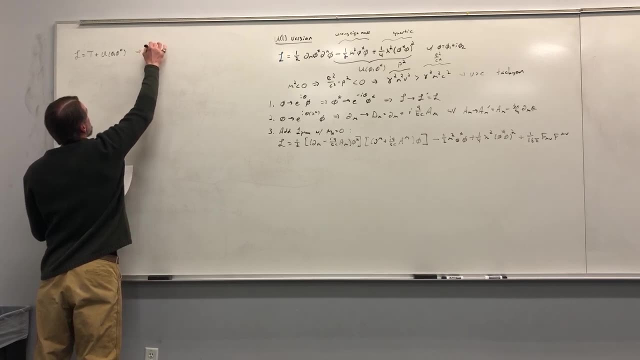 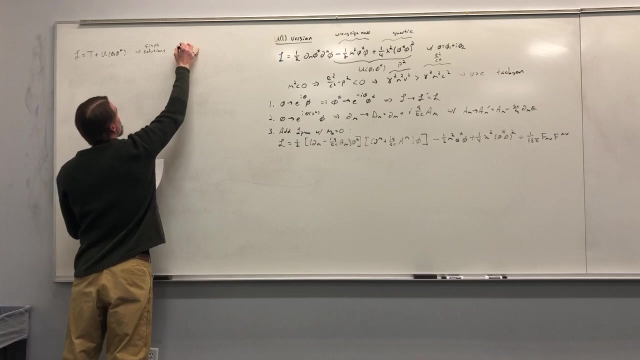 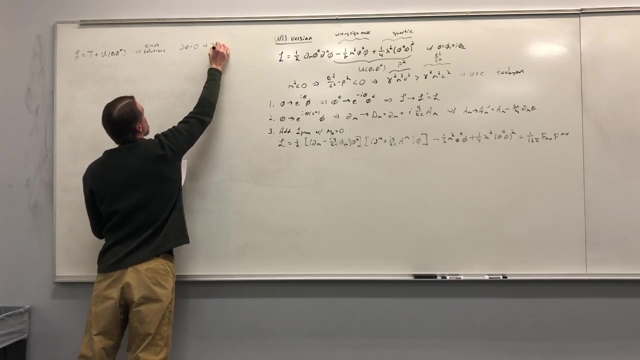 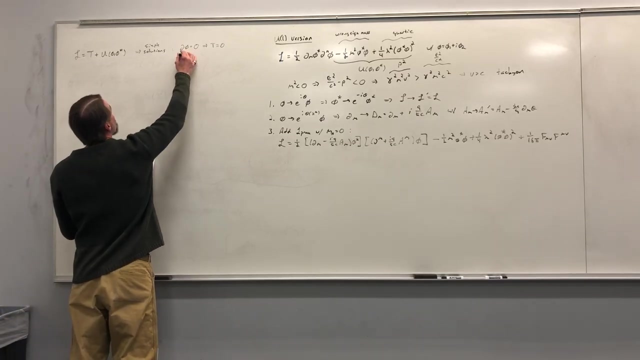 Okay, Then the simplest solutions for backgrounds- and I'll just write simple- are in setting the derivatives of phi to zero, which of course sets the kinetic term to zero, Okay. And then the derivative of phi to zero, And then also setting the derivative of the potential, with respect to, say, phi star equal to zero. 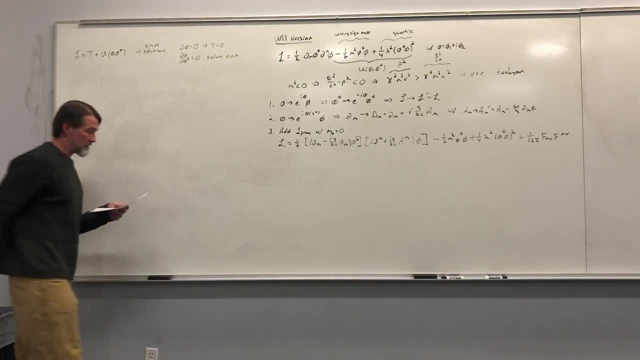 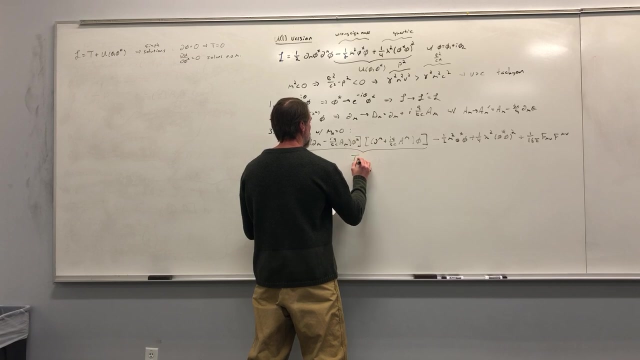 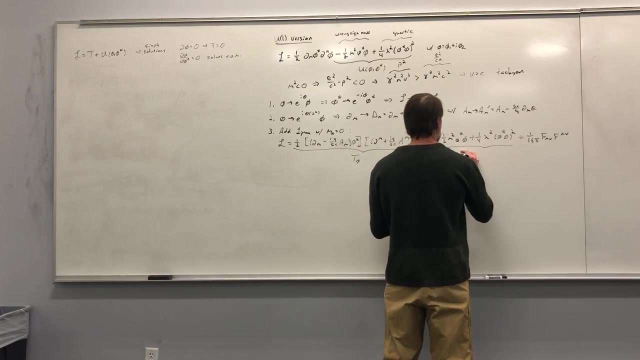 And these two combined solve the equations of motion. All right, Now in here I have the T of phi term- This is the kinetic term for the phi field- And then here, of course, I have the U of phi phi star term. 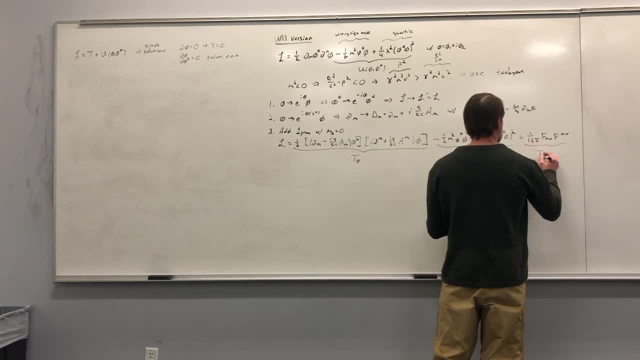 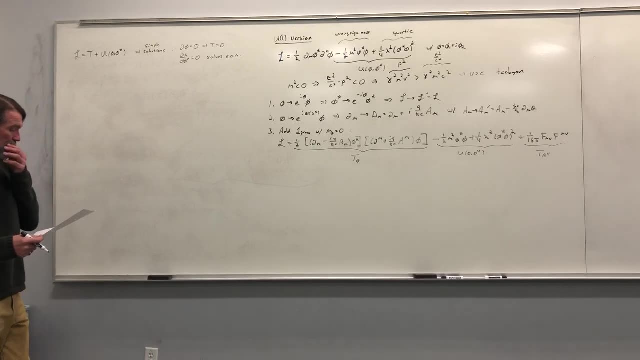 That's the potential, And then this, of course, is the kinetic term for the gauge field that I added. Okay, So one solution which we can immediately write down is: I can set the gauge field to zero everywhere, And I can set the phi field to zero everywhere. 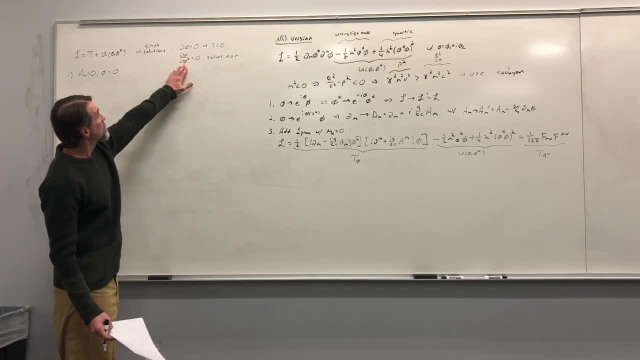 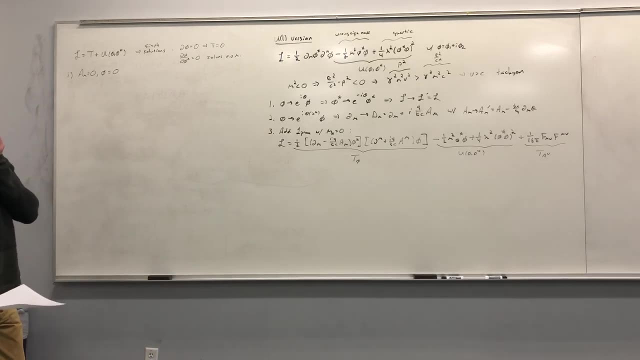 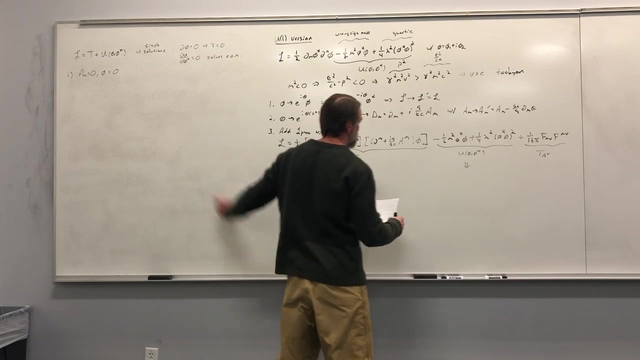 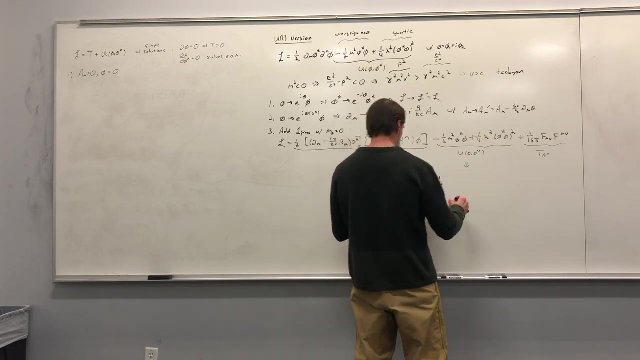 That is clearly a solution of this form to this thing. Okay, Well, let's see. Okay, Let's look at this for a minute. I want to set d mu phi star x to zero, So d mu d phi star x is just minus 1 half mu squared phi plus 1 half lambda squared phi star phi phi. 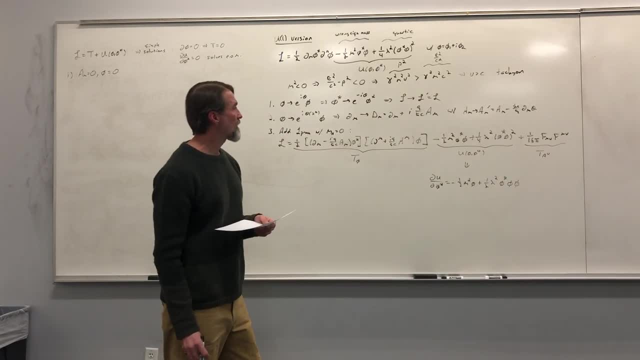 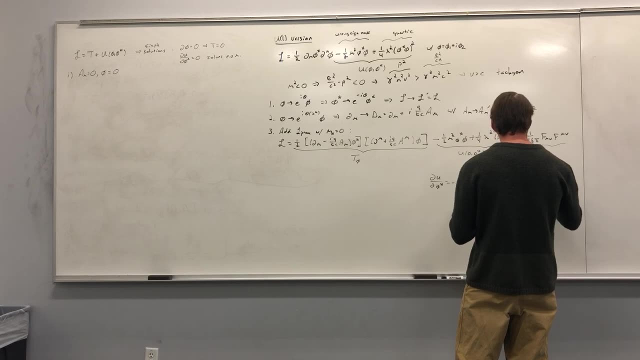 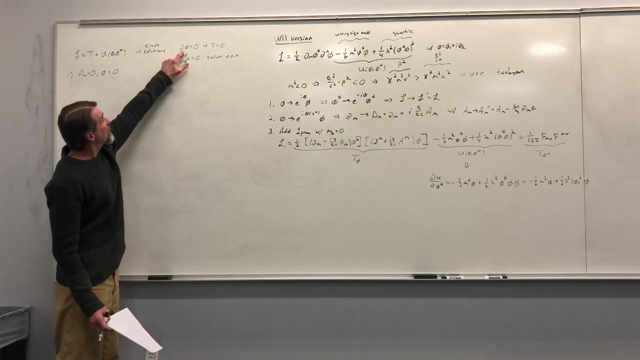 Okay, Which of course we can write as minus 1 half mu squared phi, plus 1 half lambda squared complex magnitude of phi phi. But what's important is we're going to set the derivatives of phi to zero, So we're going to set these T terms to zero. 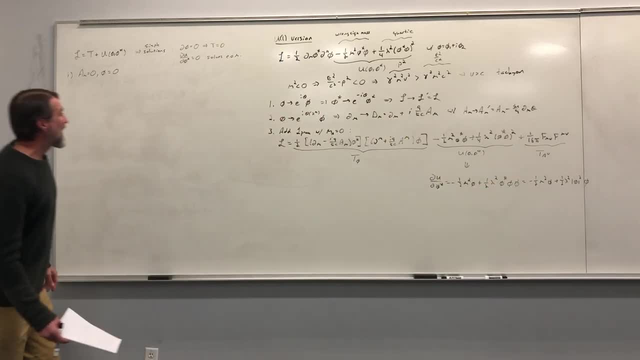 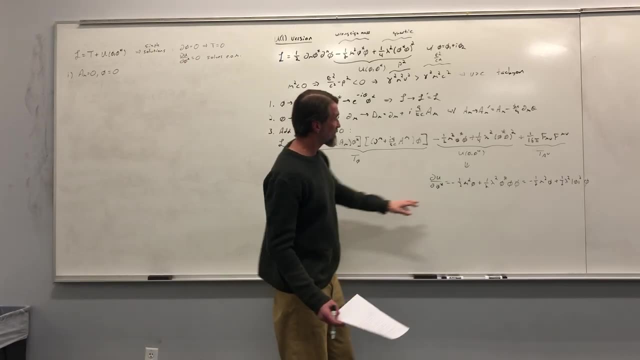 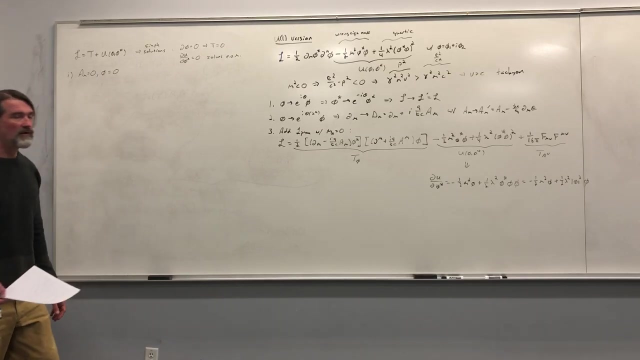 Okay, And then we just want to show that phi equals zero satisfies this derivative condition, which obviously it does. There's a phi, There's a phi. If you set phi to zero, you've got d mu phi. d mu d phi. star is zero. 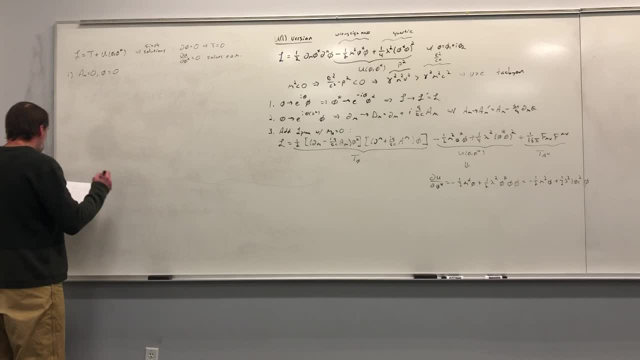 Okay. So now what we can do is we can ask: all right, how do fluctuations behave in this background, To figure out how fluctuations behave. what we basically do is we say, okay, I'm going to take the field phi of x to be the background. 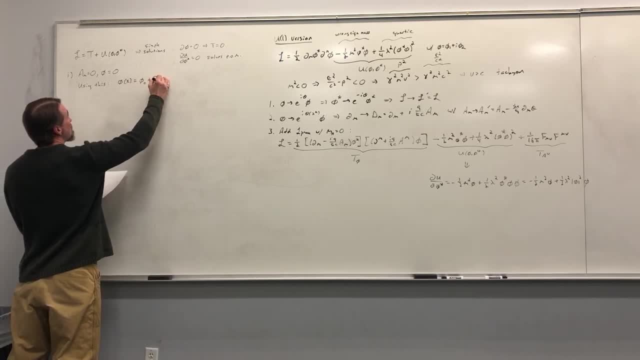 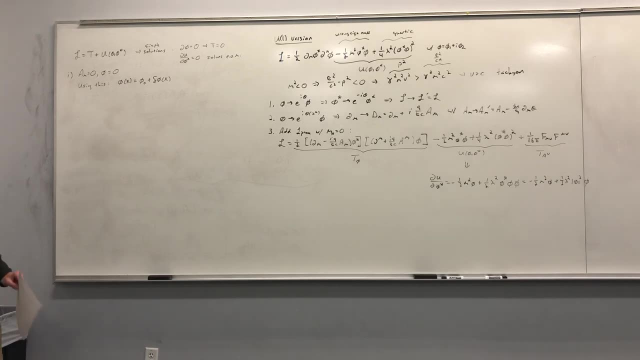 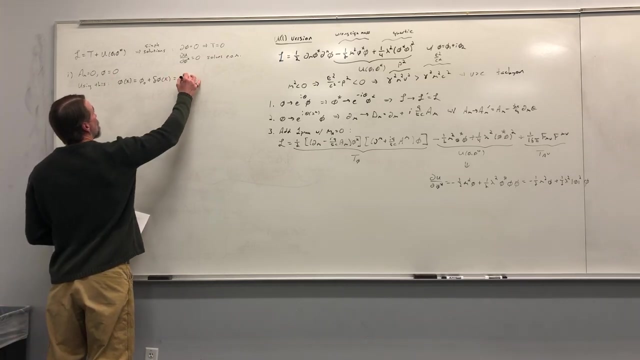 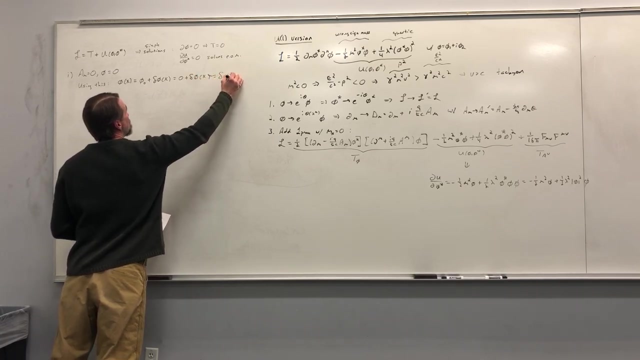 which I might call phi, naught plus a fluctuation in phi, And I'll just write x, and by x I mean x, mu, Okay, But the background configuration for phi is just zero, Okay, Which means of course that the field configuration in this Lagrangian is just in terms of the fluctuations. 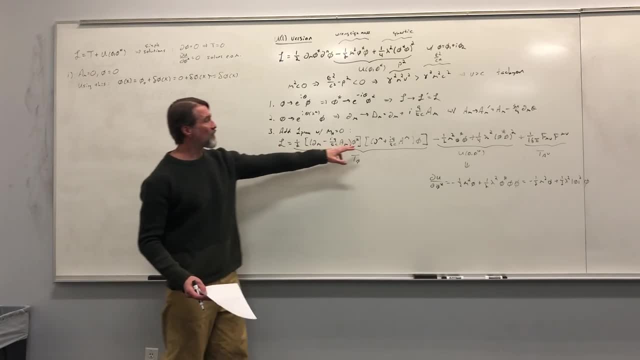 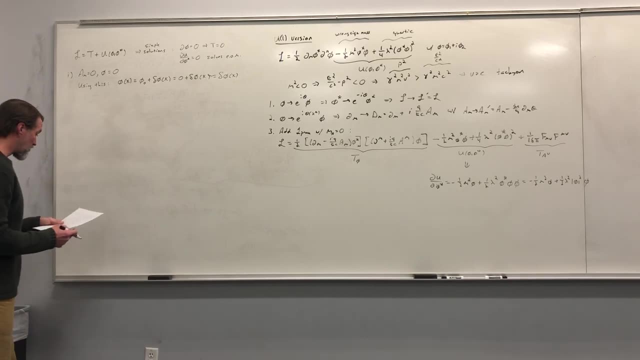 So I can literally take this Lagrangian, and everywhere I see a phi or a phi star, I can replace it with delta phi or delta phi star. It's that simple, Okay. And then similarly a mu x, Since a mu x is zero. 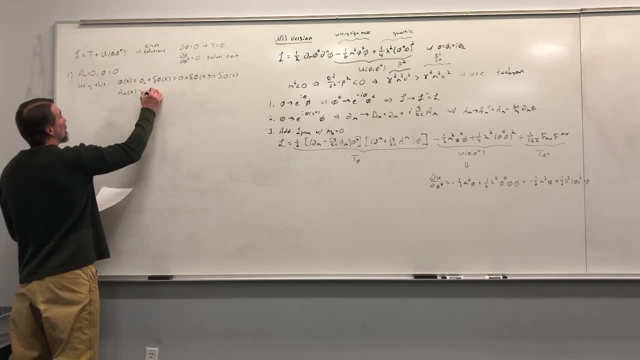 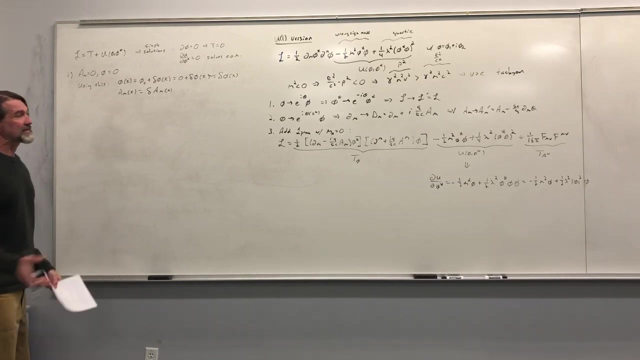 Since a mu background is zero, this is just going to be delta a mu x. So everywhere I see a mu in here, I put in delta a mu. Okay, Now I'm not actually going to write this down, because that's a waste of time. 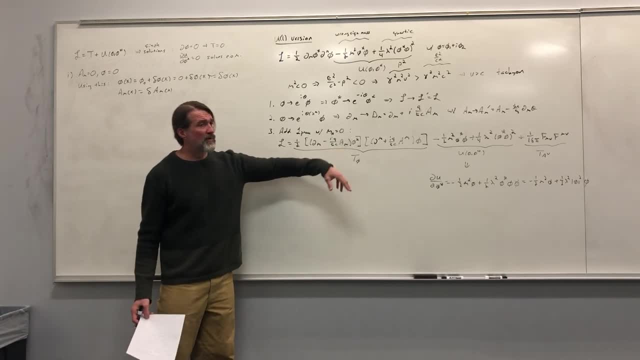 But you can literally take this Lagrangian. and everywhere you see a mu, replace it with delta a mu. And everywhere you see phi, replace it with delta phi. And everywhere you see phi star, replace it with delta phi star. Okay, 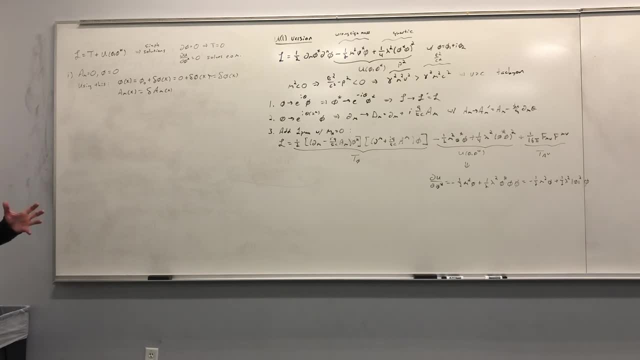 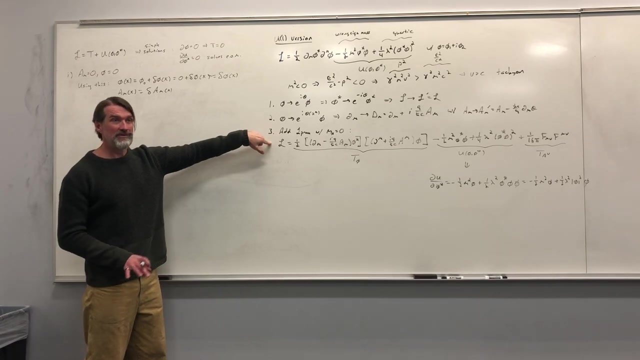 What we have now is the Lagrangian, describing the tiny fluctuations around this background, And it just so happens to look exactly like the defining Lagrangian. This is a trivial story. We need something less trivial, To which we now turn. Are you ready? 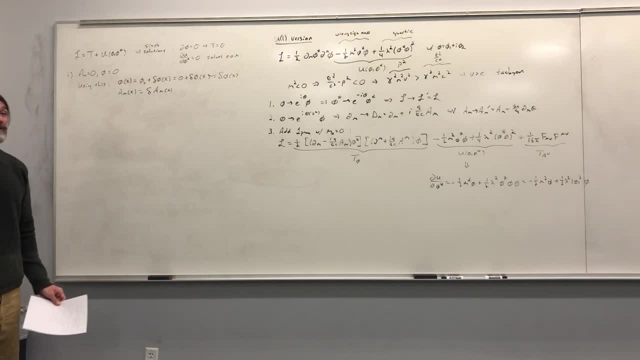 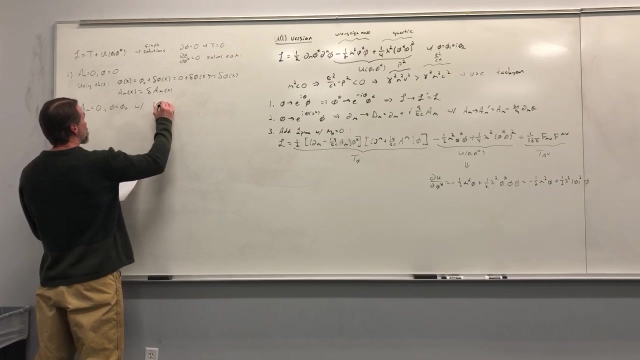 Okay, And it turns out there's some incredibly magical sauce in the less trivial case. Well, here's another solution. A mu equals zero And phi equals phi naught. Okay, Where phi naught satisfies that, phi naught squared equals mu squared over lambda squared. 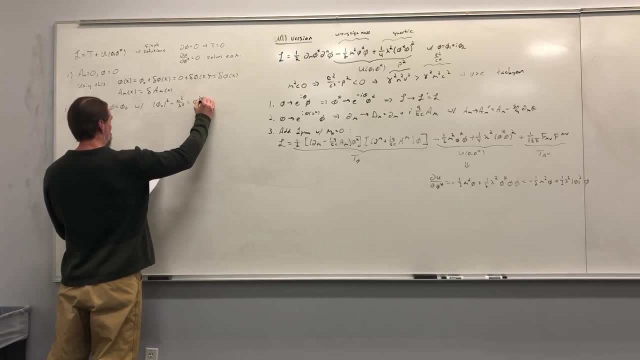 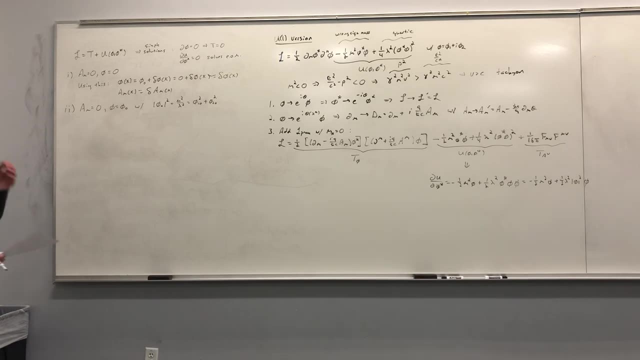 Which is, of course, phi one naught squared plus phi two naught squared. I might need some help to prove that that's true, Can I? Oh, Is this going to satisfy these conditions? So the naught is just indicating that this is the background. 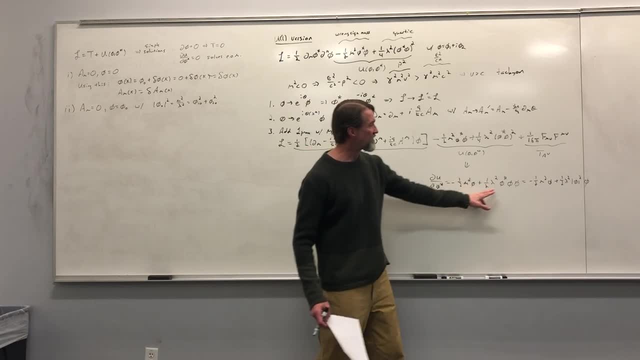 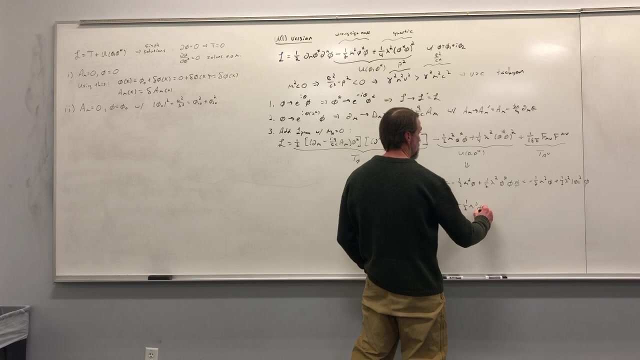 So you can take this expression here and just replace phi with phi naught everywhere. That's fine, Okay. So you know this is going to be partial, u partial. phi naught star is minus one half mu squared phi naught plus one half lambda squared phi naught. complex magnitude squared phi naught. 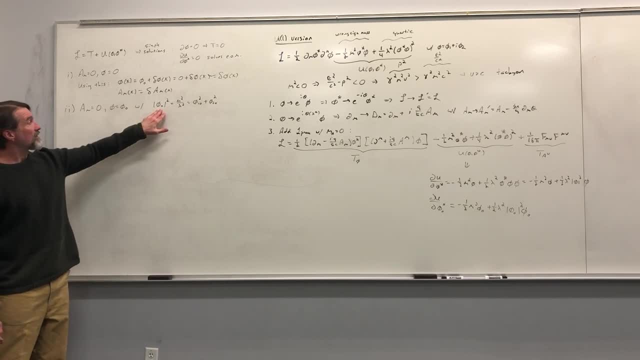 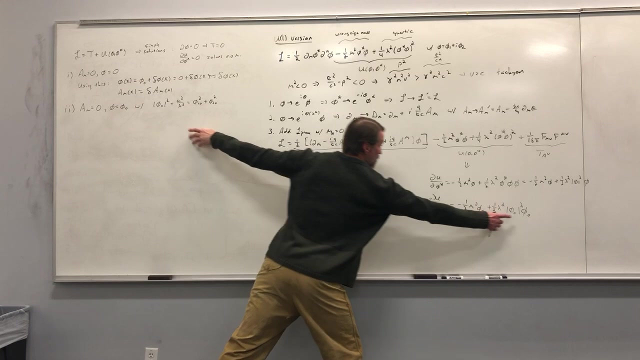 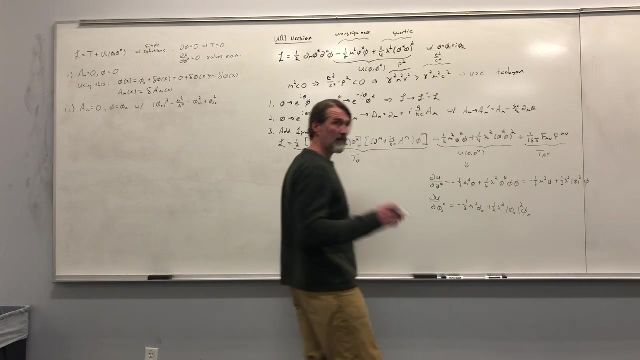 Is that going to be zero for a phi naught whose magnitude squared is equal to zero? No, No, This which is right there. if I plug that in for this, what will I get? Zero, Zero. Okay, Everybody see that. 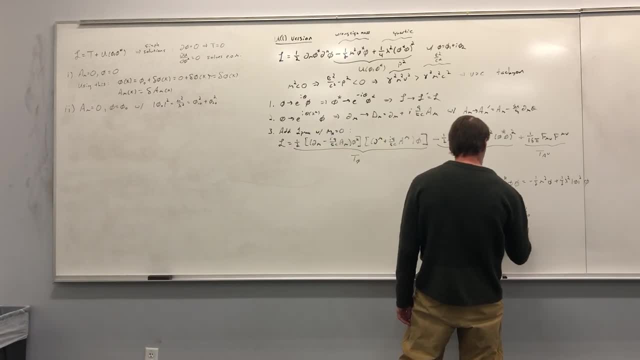 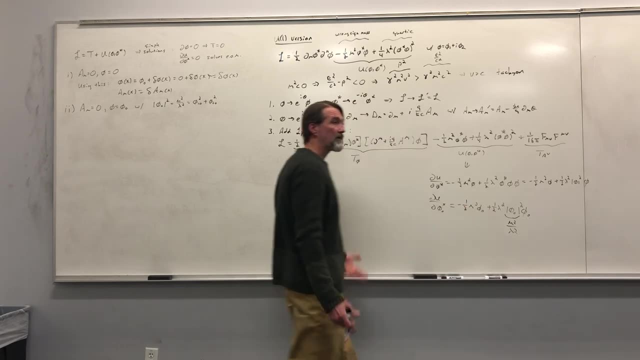 Is that obvious? I mean, obviously, if I put in mu squared over lambda squared, Then the lambda squared's cancel, And this is one half mu squared phi naught minus one half mu squared phi naught. It's zero, Okay. 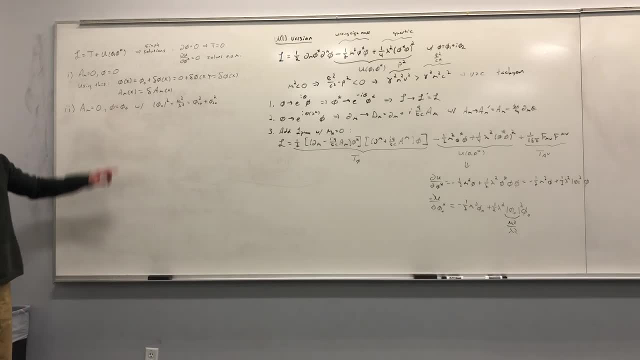 Here's the important thing: It ain't zero, It ain't zero. So now we have to investigate what consequence that brings. Well, this is the condition that it has to satisfy, And I'm just going to pick a particular value for this. 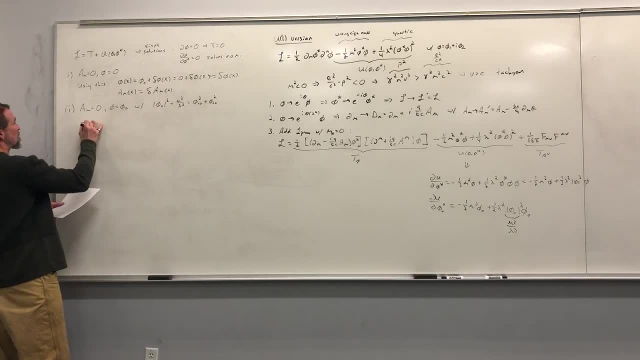 I mean, you can use, you know, anything you want. So what I'm going to do is I'm going to say: let's suppose that the real part of this is mu over lambda And the imaginary part is zero. That's one way to get this. 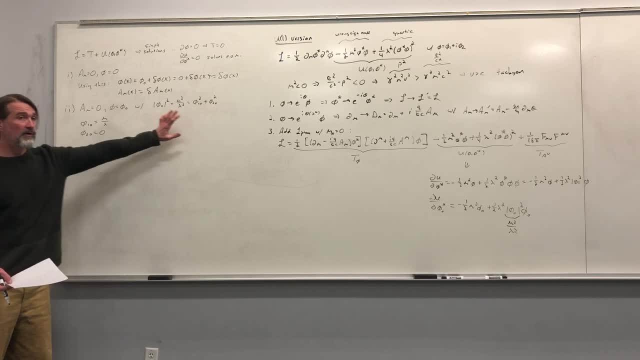 Remember, this is a complex field. So this is the real part squared plus the imaginary part squared, Because we're doing a complex magnitude squared. I'm just going to take the real part to be mu over lambda, The imaginary part to be zero. 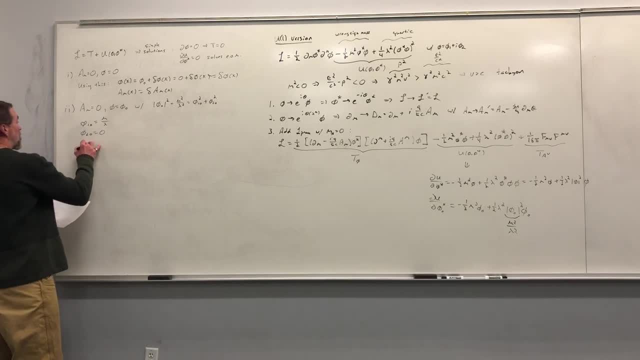 That's the way this works out, And then, of course, we're going to take a mu to zero, Okay, And then what we want to do is we want to study. So these are the background configurations. Now we want to study in terms of our new fields, whatever the background is, plus fluctuations. 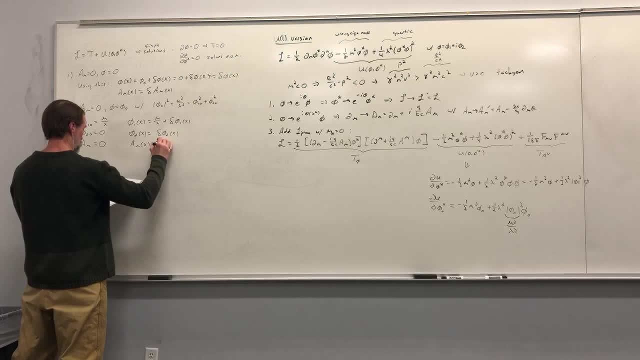 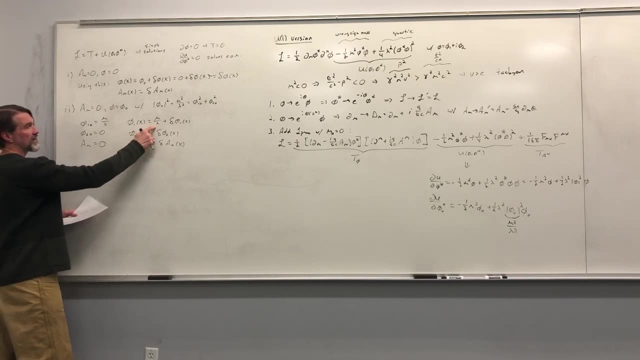 Okay, Where the only change is that right there. So the fluctuations in the field in phi 2 is just the fluctuation, The field in A is just the fluctuation, But the field in phi 1's case is the fluctuation plus this guy. 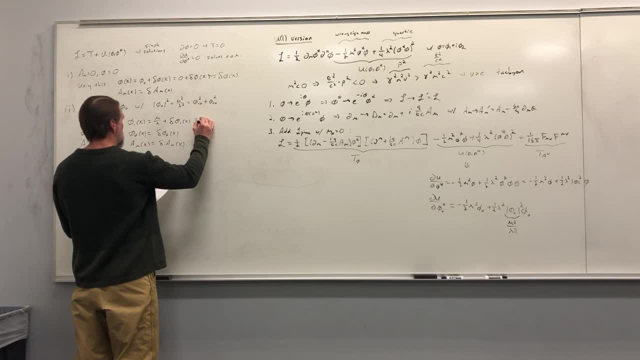 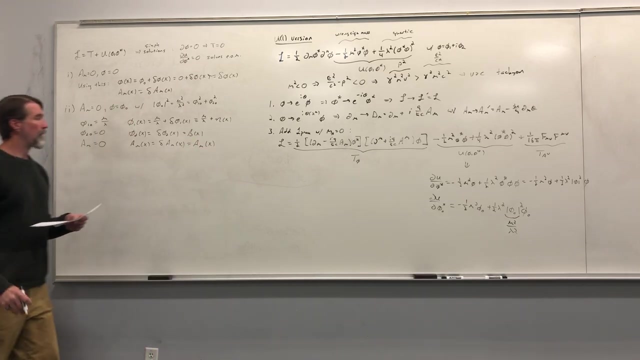 All right, Now I'm going to give these some new names. I'm going to call this mu over lambda plus eta. I'm going to call this beta And this will be, of course, eta mu. Okay, We don't really need this delta in here, because the delta A mu is the same as A mu. 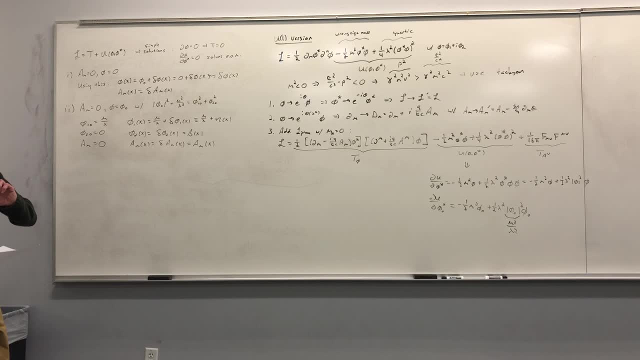 So we'll just call it A mu. Okay, Now what I'm going to do is I'm going to take this for phi 1x, This for phi 2x, This for A mu x And I'm going to shove it in here. 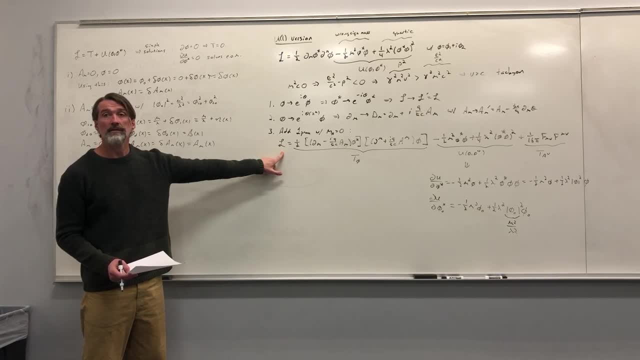 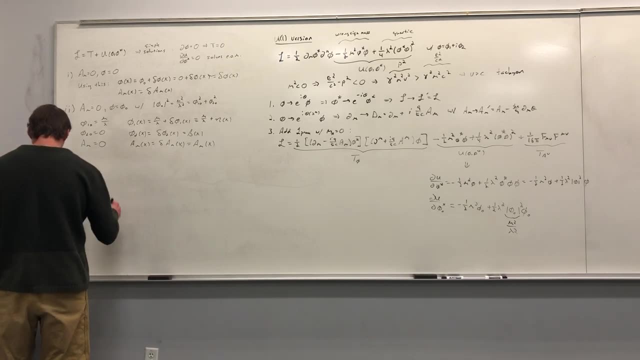 And I'm just going to write down what I get. It's going to take a minute. Get your jokes ready, Starting with huh. Tell a joke, Tanner. It's going to take a minute. It's awfully quiet in there. 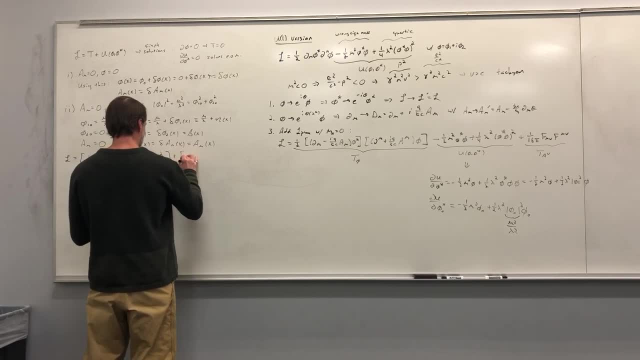 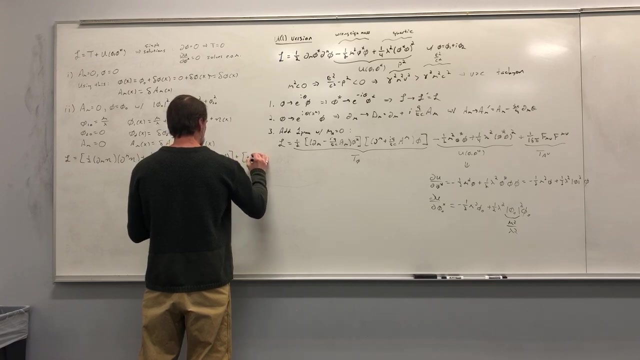 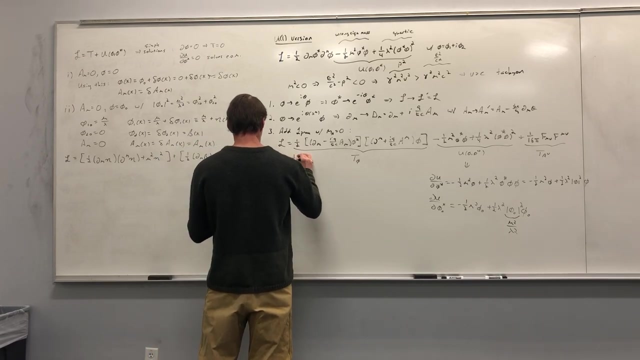 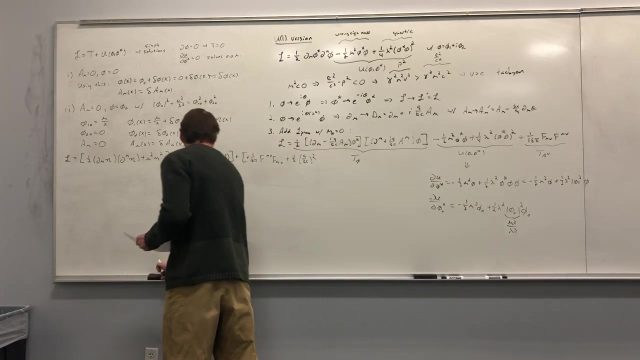 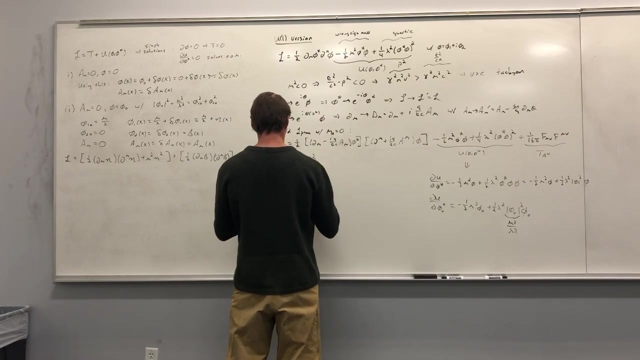 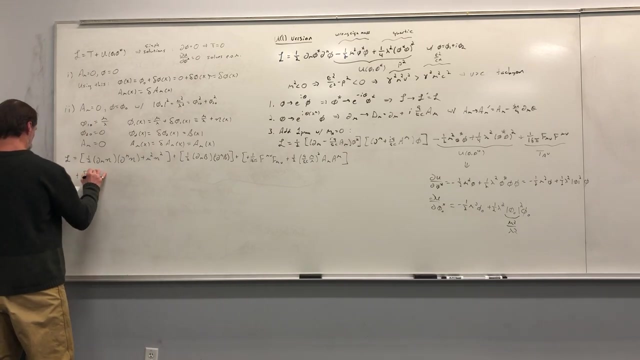 Watch Right as I'm writing the last piece of information down. I'm going to be like: oh yeah, I remember It's the best joke ever. No, it doesn't matter what you think, Just tell them. 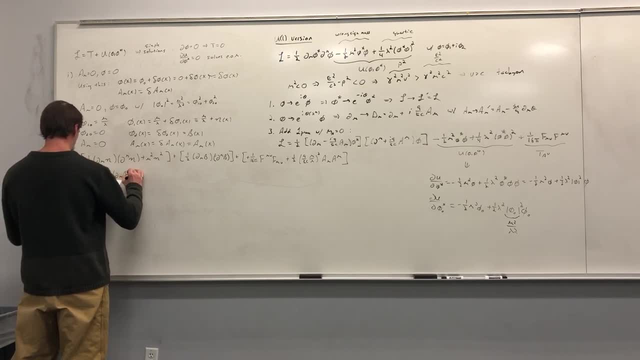 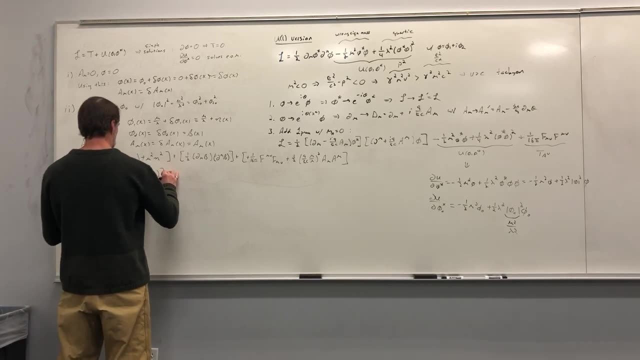 You got a joke. I have a joke, I have a story though. Okay, We'll take a story. It's a story about a little bee on its first day of school. So he was so excited Finally went off to college- freshman year, you know. 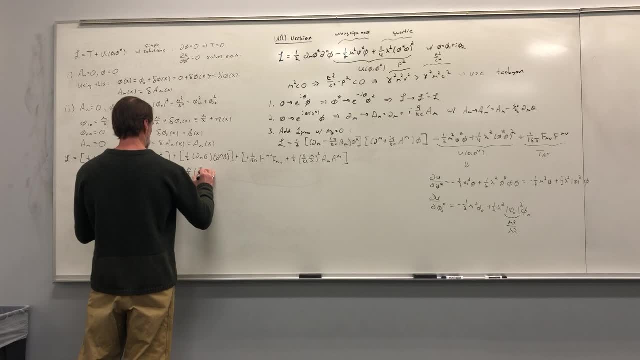 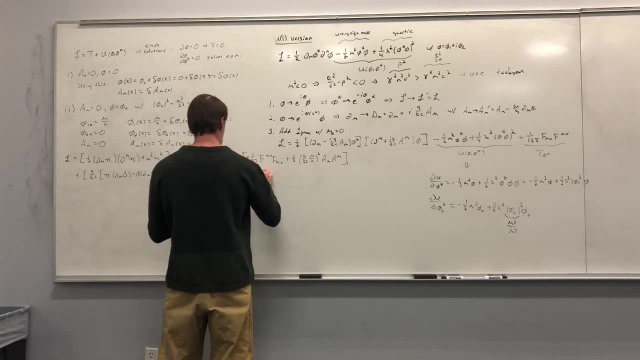 Kind of nervous about it, Decided to start talking to people, try to make some friends. Finally, a weekend came and he was invited to go to a party. He's like: oh my goodness, I'm going to go dress up, put on my fancy party clothes, go party with my new friends. 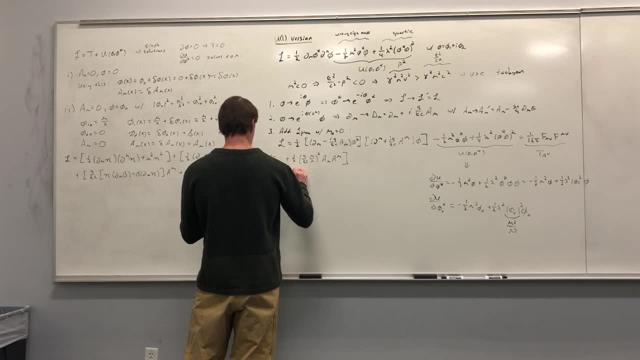 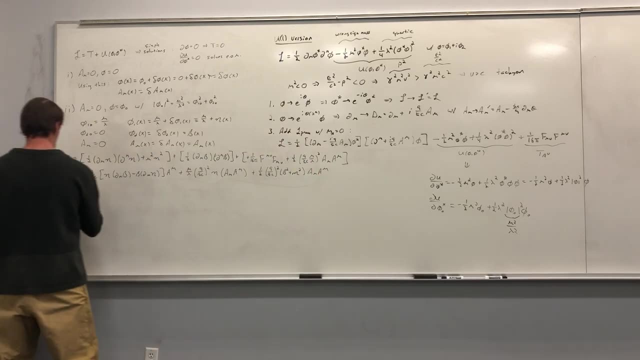 So he got there and he was bussing And there were tons of people at this party, He was making all these great new friends And he was talking to this group And he was finally like: oh my goodness, Do you guys want to go get something to drink? 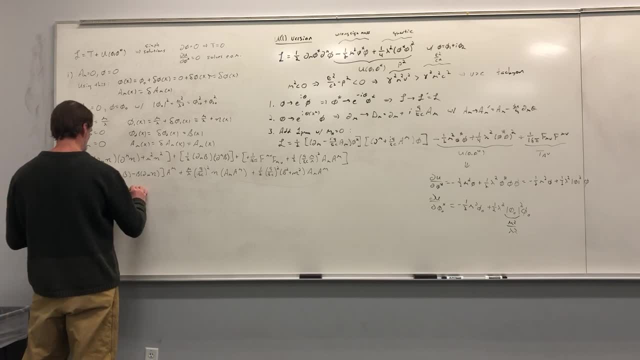 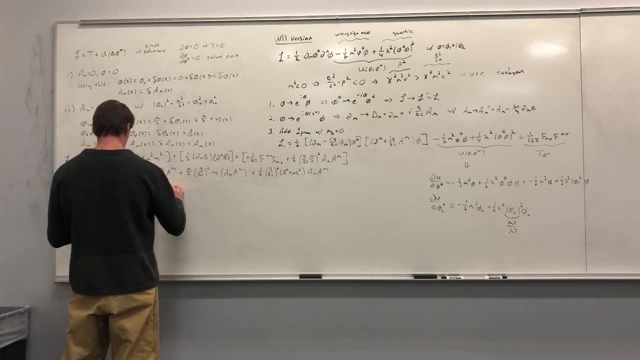 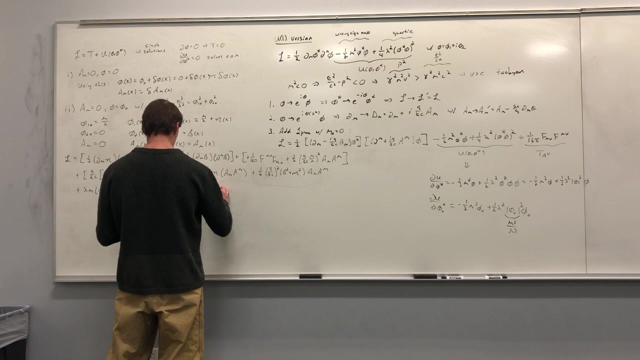 You know there's this big long line, So I'll go stand in line for us and get us something to drink while you guys keep on hanging out and having fun. So he's waiting in the punch line, Waiting forever, forever, forever. 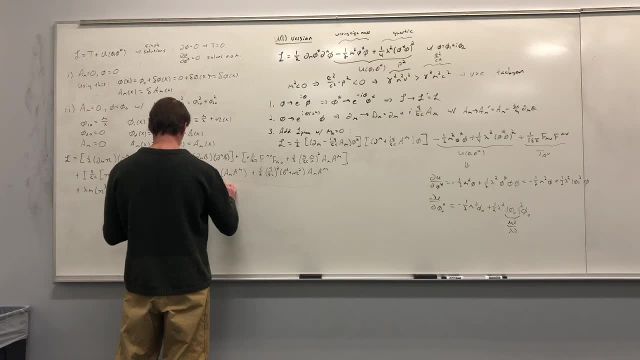 Finally he's like: okay, I need to go to the bathroom. So he talks to the person in front of him. He's like, oh, my goodness, I need to go to the bathroom. I'll be right back. Please tell me if there's a line. 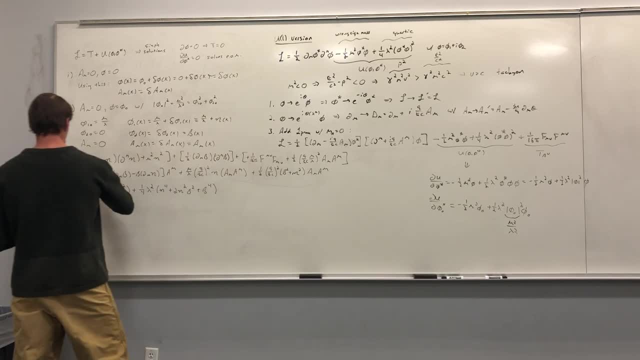 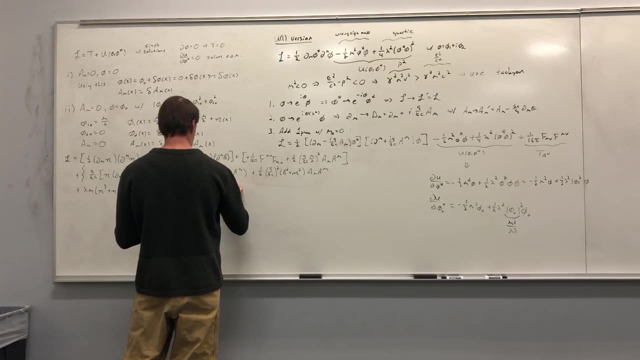 The guy in front of him is like sure, of course, Anything for a new B friend. So the B went off to the bathroom And when he came back there was no punch line. Good night. I wish I could have focused on that. 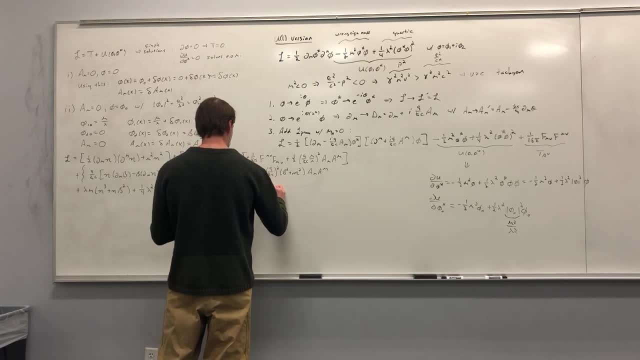 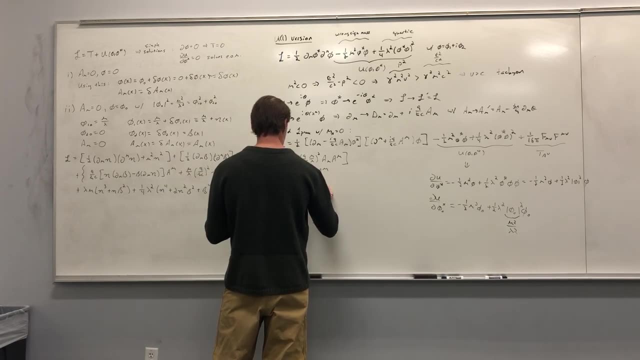 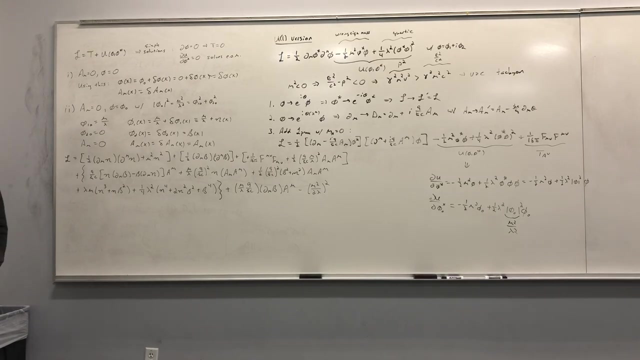 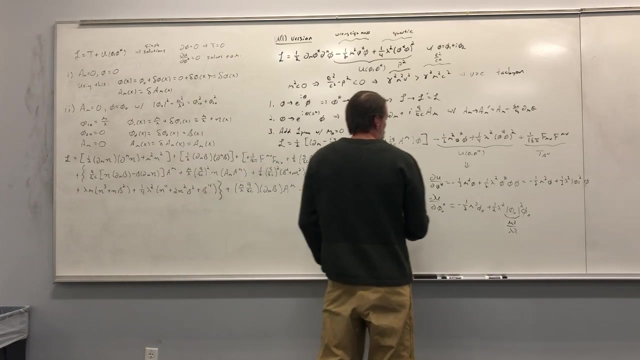 I'll be glad you're laughing. I'm trying not to screw this up, But it's excellent timing because I'm almost done, So I'll give you that. There you go. It's a pretty simple expression. Pretty simple expression, isn't it? 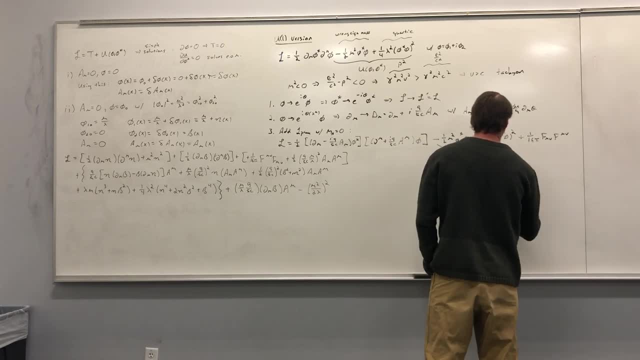 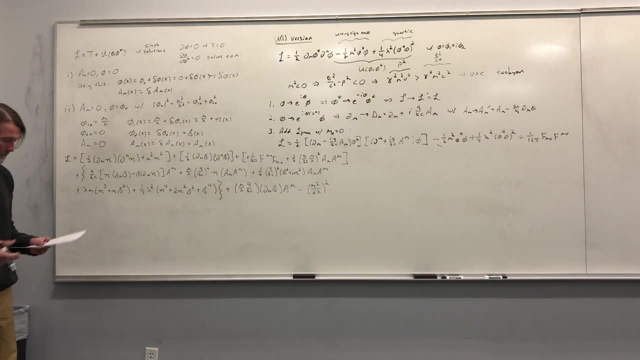 All right. What do you think? It's pretty, isn't it? It's gorgeous, That one damn term. Otherwise, we would have gotten exactly this, Exactly this, Because all of the Phi 1 and the Phi 2s would have just combined into complex things if they were behaving exactly the same way. 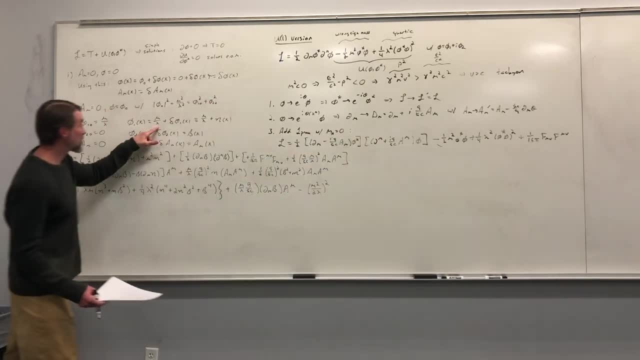 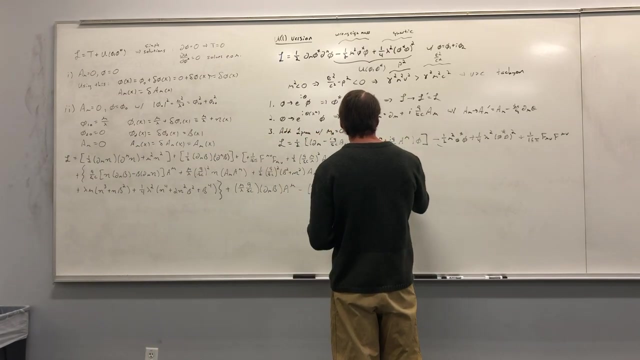 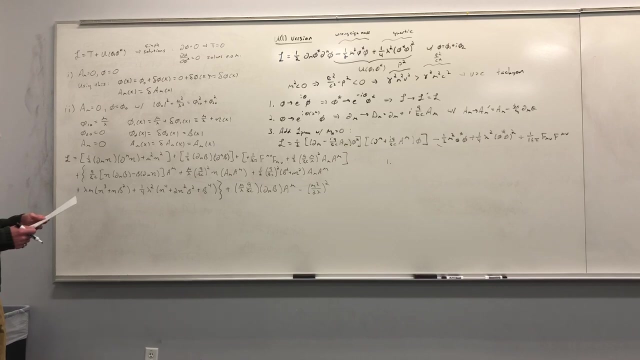 And it would have just basically spit out this: if this had been zero. But this is not zero, Okay, Sucks, But this has got some interesting properties, Okay, Oh shit. Oh, wait a minute, Hold on. What is that? 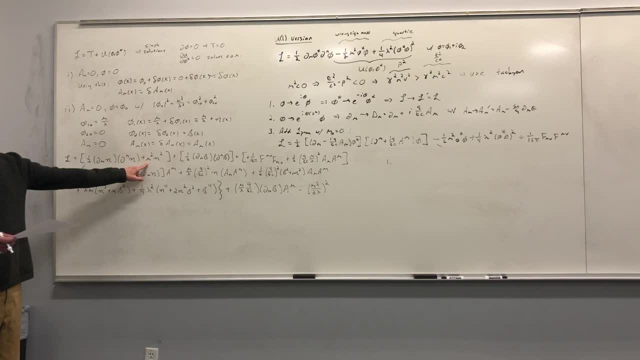 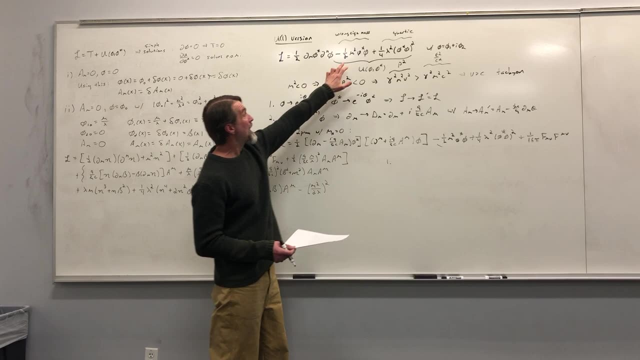 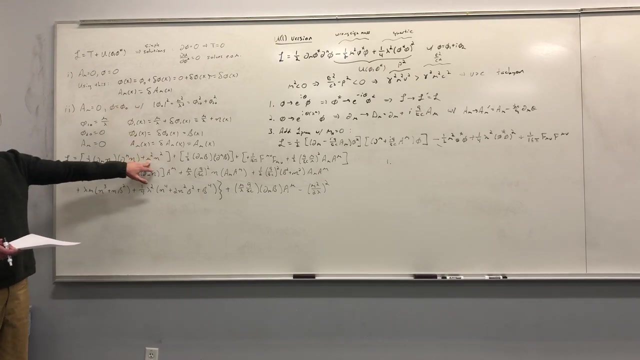 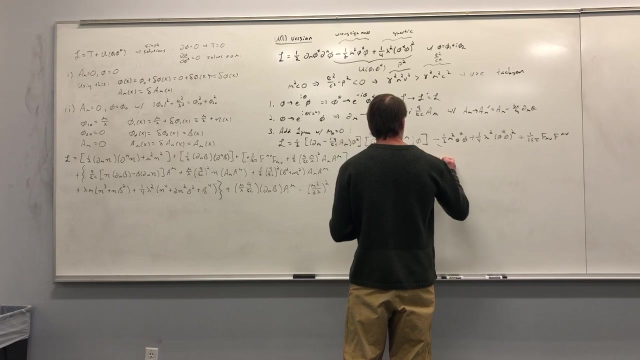 That's a mass term, The scalar field, which did not have a mass term. It had this tachyonic mass thing. Because of this background, all of a sudden we have a positive, mass scalar field. Okay, So we have a massive, real scalar field. 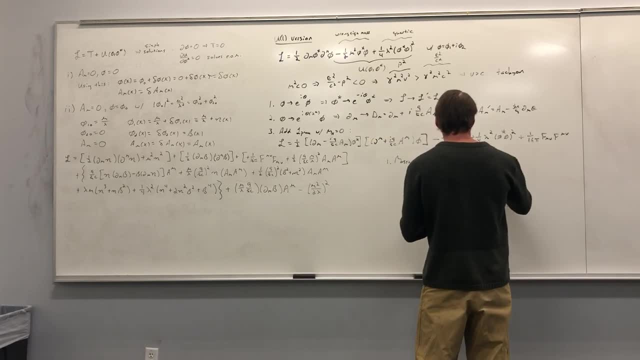 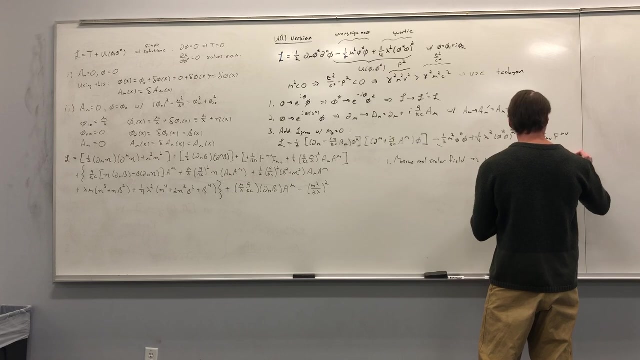 Okay, And then we have an eta with, of course, mu squared equaling one-half the mass of eta, c over h-bar squared, which of course means that the mass of eta is root 2 h-bar over c O times. 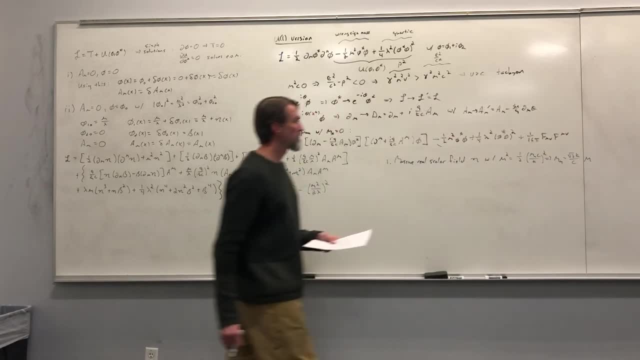 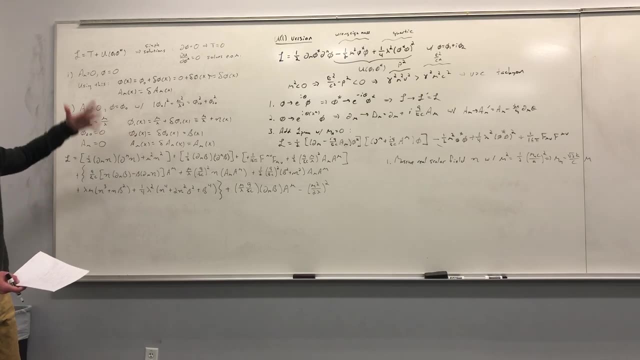 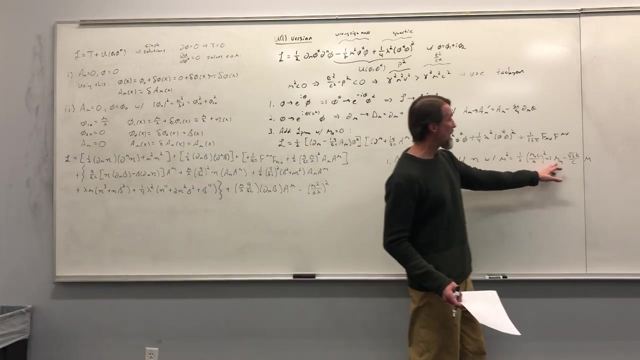 Okay, So that's just taking this and setting it in the form of an obvious mass term, which I don't have up there. But if you had set this equal to the coefficients of a mass term for a scalar field, then you could find that the actual mass is root 2 h-bar over c times this parameter, mu. 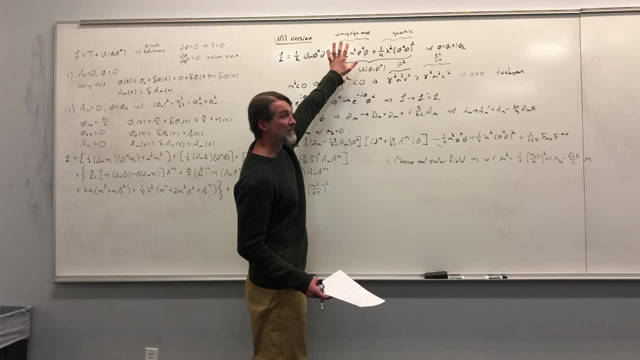 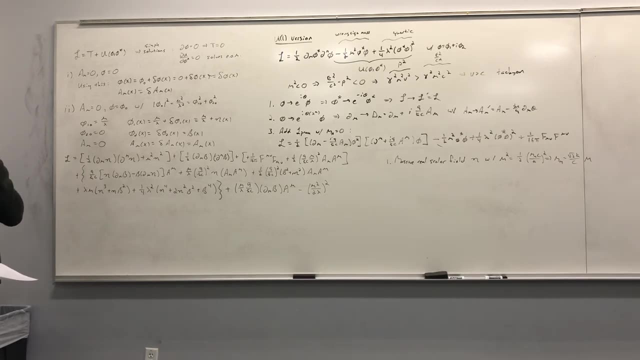 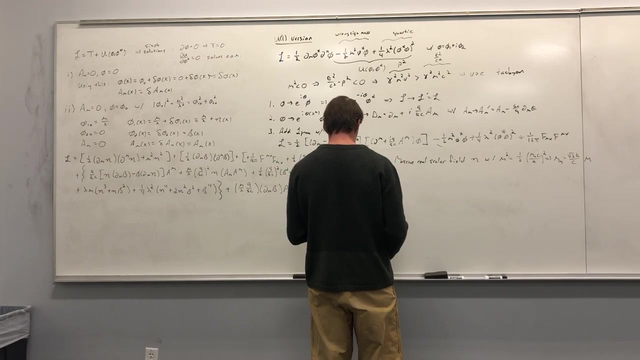 Which I might as well just call this a parameter, mu. I shouldn't call that a mass, because that's not a mass term, Okay, But what's important is this scalar field is massive, Okay, But it gets better than that. Remember that. 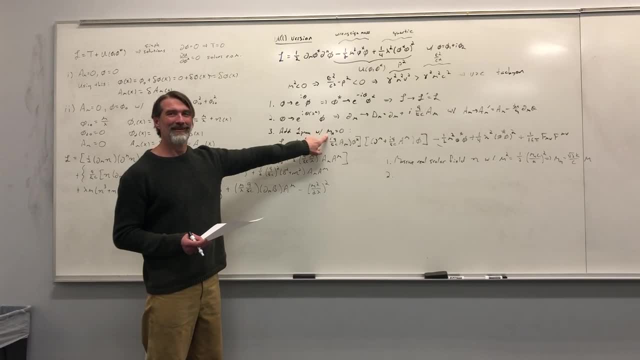 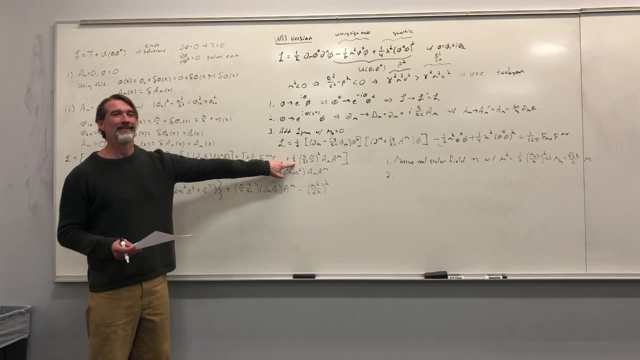 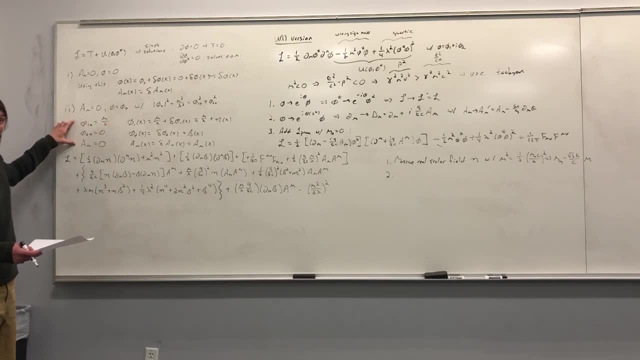 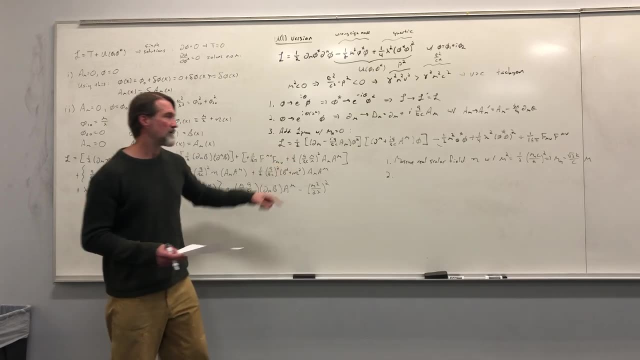 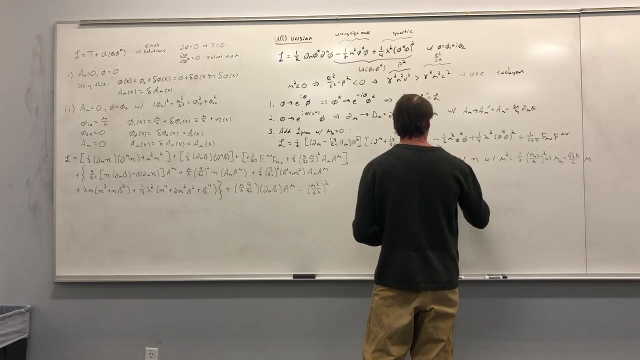 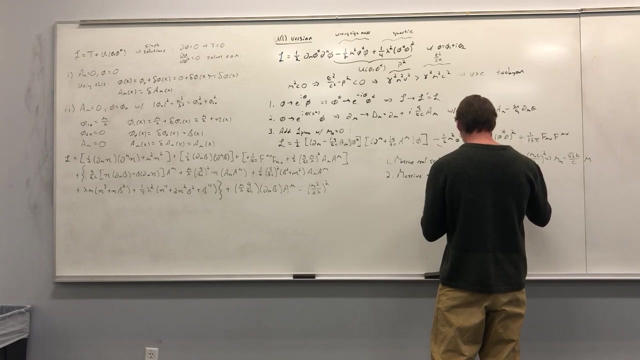 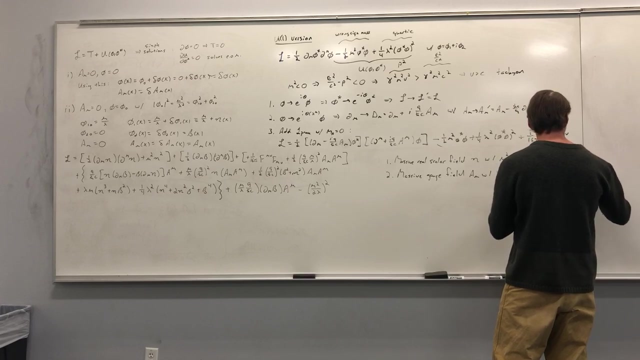 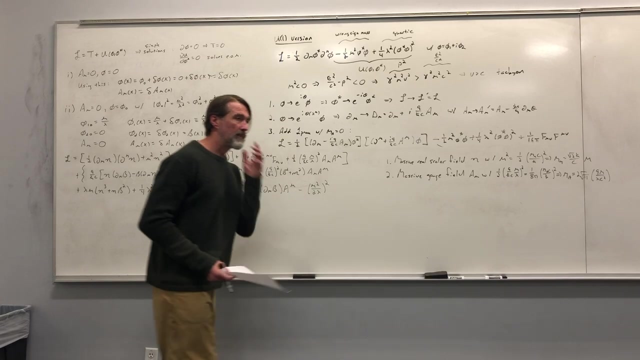 And by using this solution for the background, we suddenly find ourselves with a massive gauge field. We have a massless gauge field. The gauge field is 2 root pi, quantity q, mu over lambda c, squared Again. all you do is you take this and you bang it into the usual Proca mass term. 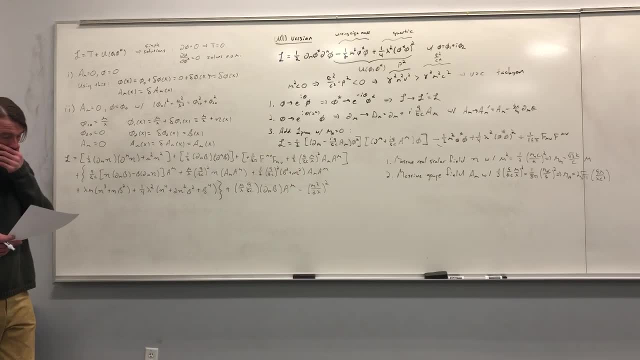 and then that lets you find out what the mass itself should be. Okay, So notice, we have a scalar, We have a scalar fluctuation which is now massive. We have a gauge field whose fluctuations are now massive. What about this scalar fluctuation beta? 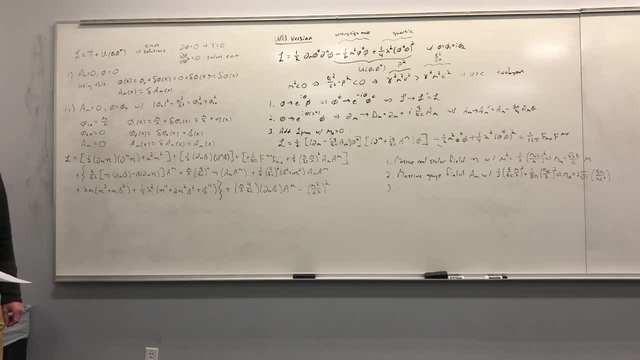 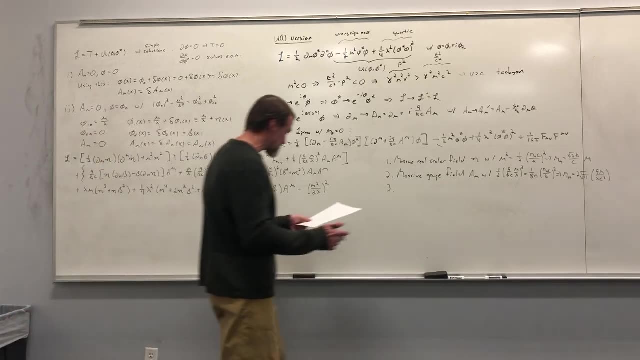 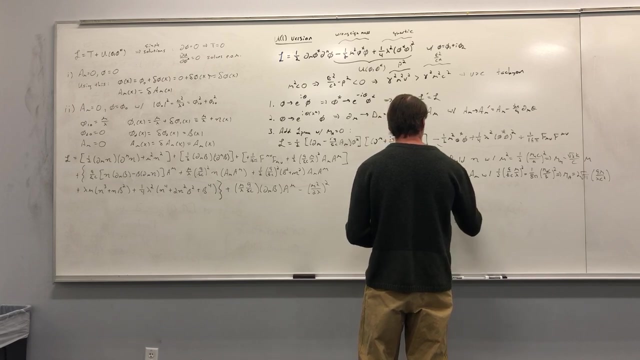 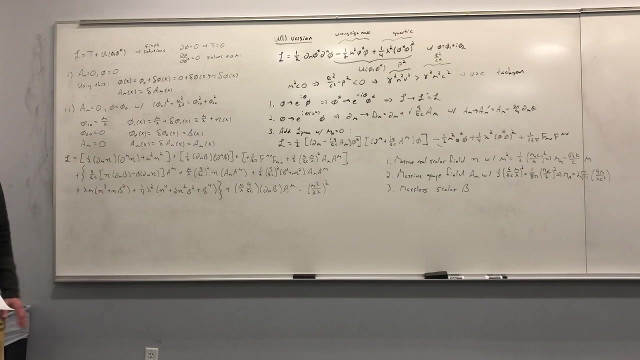 Is it massive? Oh, you're here. Oh shit, I was wondering right there. No, that's massive, massless. Okay, All of them are interacting with each other in very weird ways. Most of these were interaction terms. 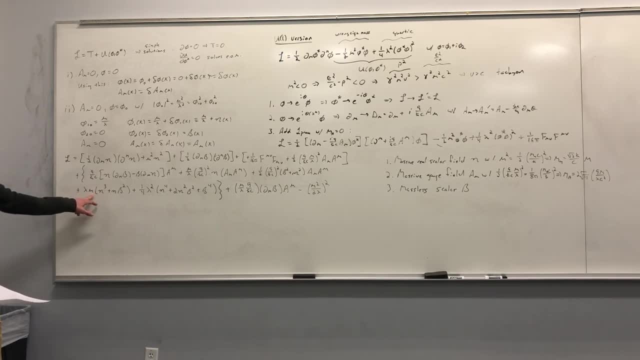 Okay, This is a mu Or sorry, this is an eta- cubed interaction. This is eta interacting with itself in a cubic fashion. This is eta interacting with beta squared. So most of these you can interpret as interactions between eta, beta and a. 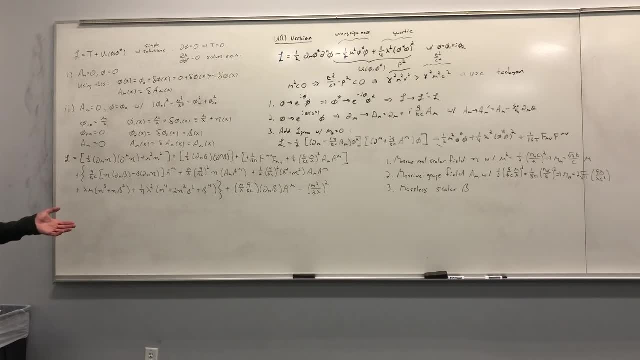 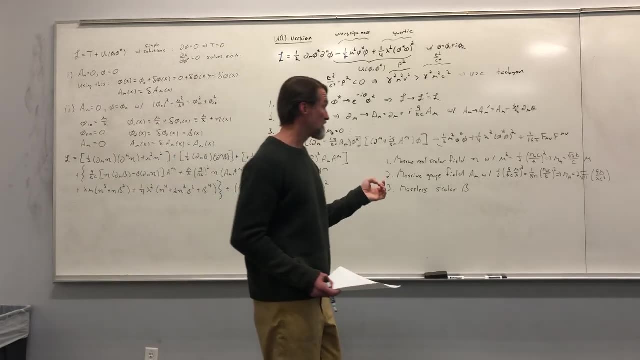 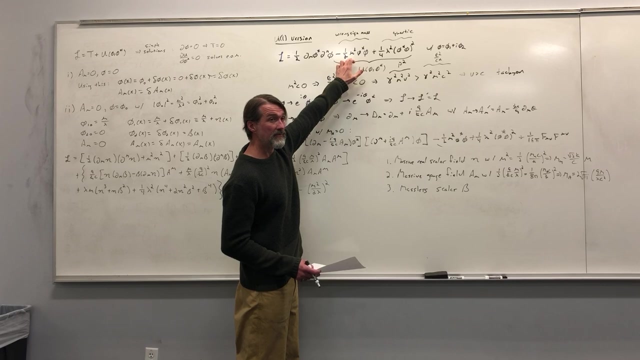 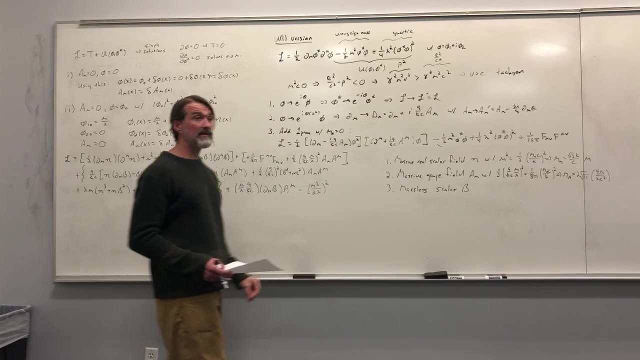 That's fine. We got what we wanted. Okay, We started out with a zero mass field or a zero mass gauge field, a weirdly negative massed scalar field, and ended up generating a positively massed scalar field and a positively massed gauge field. 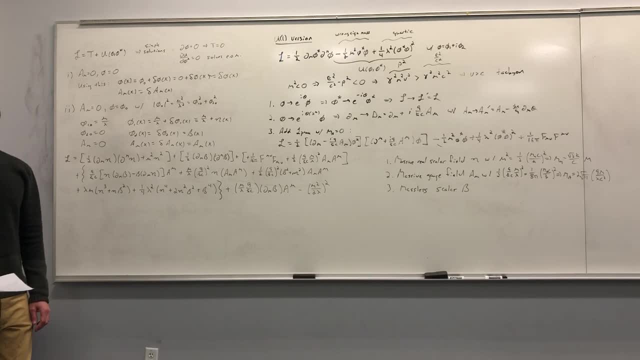 And that means that the background is generating mass, Is it? what Is the background generating mass? Is it creating mass? Yeah, We'll talk about that next time. I'll go into a pictorial version of what's happening for the background. 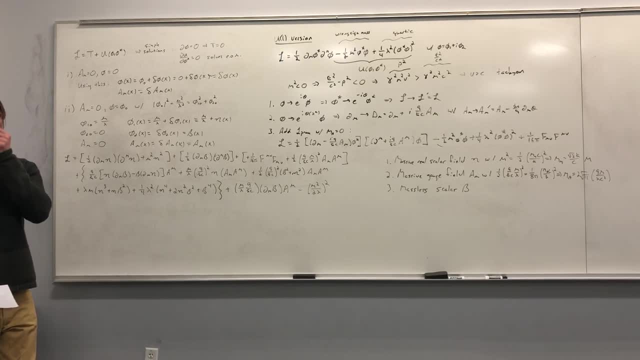 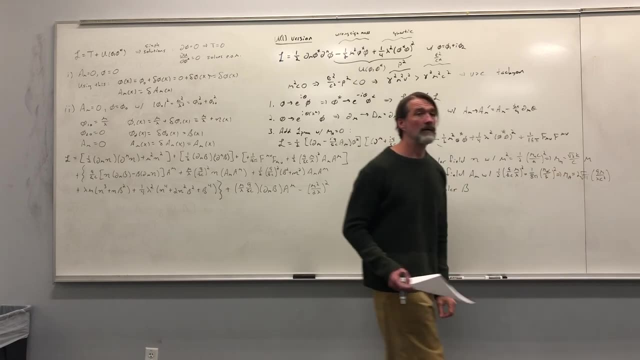 So we'll save that question for next time. Remember it. Okay, What's in the Sperm for the gauge field, The mass, The one that's on the right side? Oh, That's pi. Okay, Okay. What did I just explain to you all?